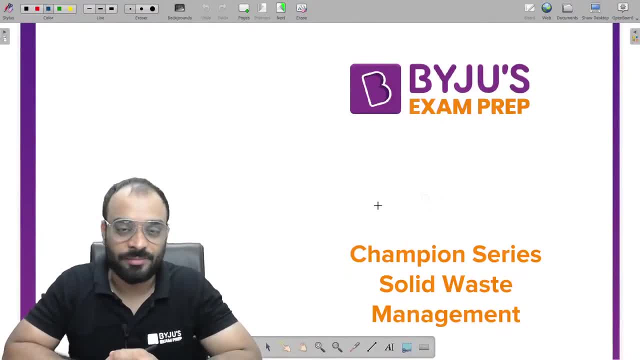 Hello, dear students, Very good evening to all of you guys and welcome back again on Baiju's exam. So today I am in front of you guys and today we will discuss the solid waste management problem- Another topic, guys, and from this particular topic you may get the question like a fundamental question, like fundamental property of solid waste. So those type of question are important for the gate exam, Not the complete treatment process or not the complete. you can say that the what are the treatments are there, how we can? 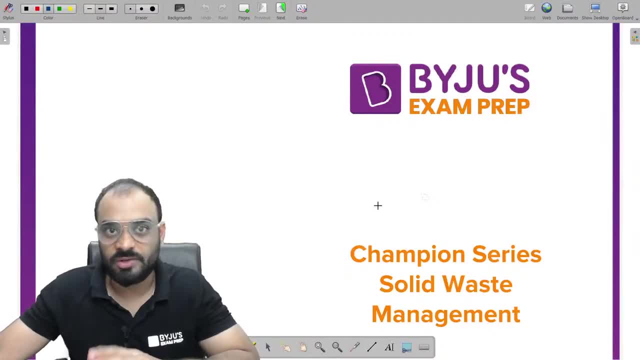 design it type of topic are not important and not relevant from this particular topic, guys, for the gate exam, Right? So good evening to all of you, Bhaskar. good evening. Come first, guys. come first and join the session and please share to other students also that everyone can join over here. And today, guys, we are having a lot of question with respect to this topic also And you may get like one question from this particular topic in your gate examination in your environmental injury. Okay, So let's start this. 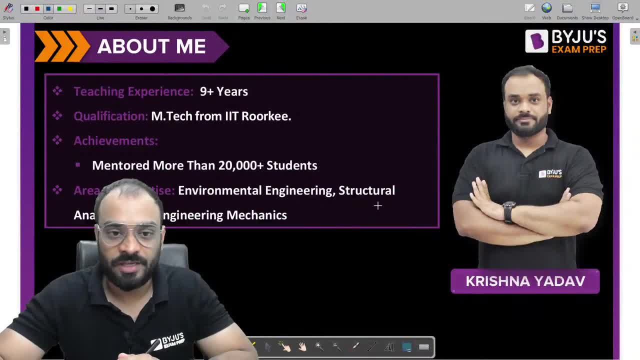 session and before starting it, guys, let me explain about me also. I think all of you know about me because you have seen a lot of lecture, Right, And I have taught you many times. But, guys, still those students who are new over here- let me explain myself also. My name is Krishna Yadav and I am teaching from last night And, guys, these are my subjects generally in which I deal, basically environment structure. Okay, So, guys, there is one more information which I want to give you. You can 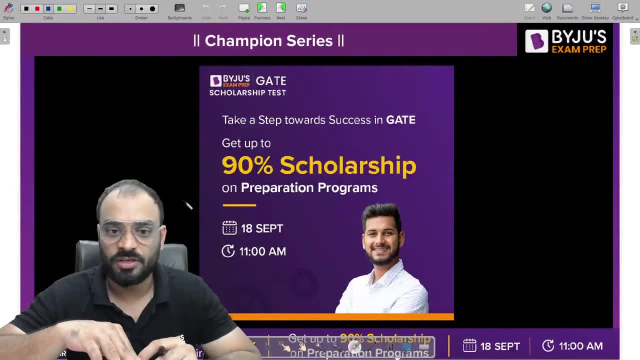 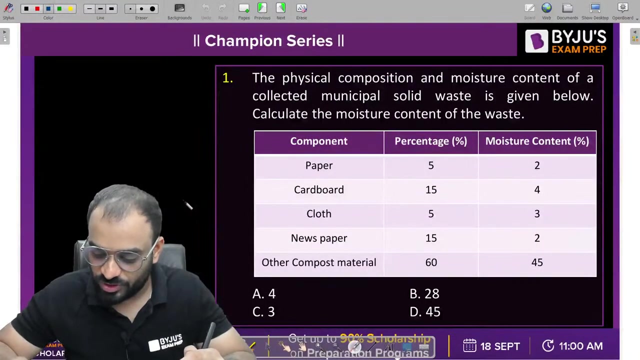 get the 90% scholarship on the gate preparation program or ESC preparation program. So what you have to do? just you have to give a scholarship test on the 18th of September at 11 am, Right? So please give it, so that you will get the scholarship for the gate preparation. Okay, So let's solve the first question which is in front of you. guys. This is the first question in front of you. 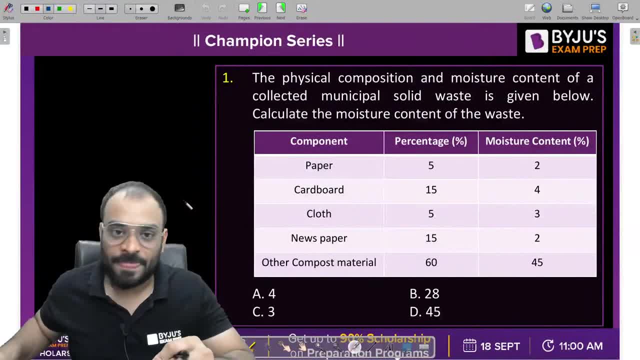 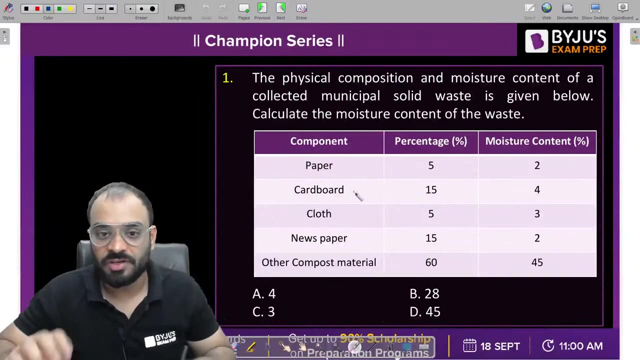 Thank you, Bhaskar. Thank you so much. Thank you so much. Okay, So this is the first question, guys, which is based upon the moisture content, Right? So we need to calculate what is the moisture content of the given sample and how we can estimate it. that we need to understand in this particular problem, Right? So let's understand, guys, how we can calculate the moisture content of the given sample. Now, guys, listen very carefully Whenever, whenever you. 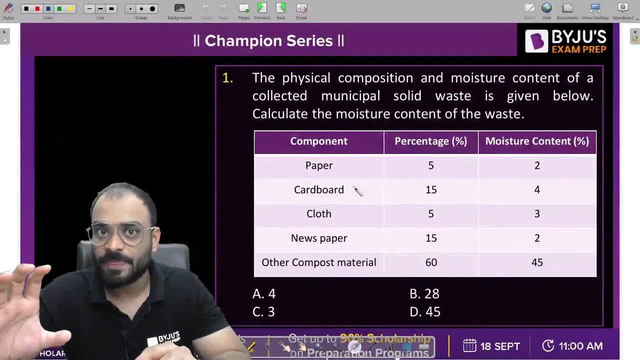 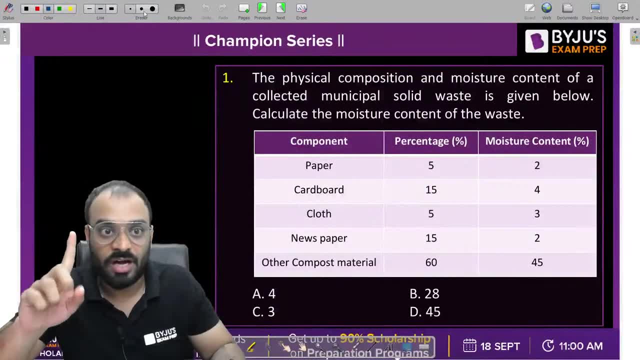 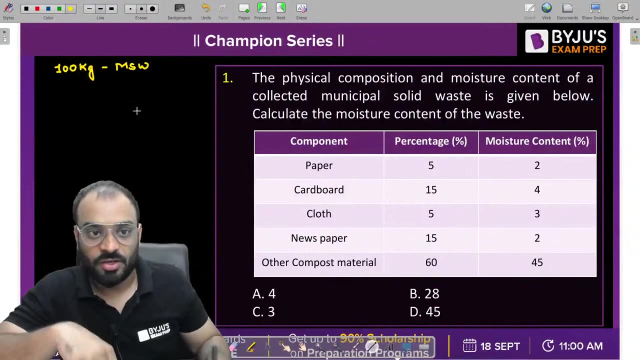 it is not mentioned, what is the sample size which we are taking in our solid waste? you need to consider it as a 100 kg. That is a standard one, Okay? If it is not mentioned, then you have to consider it. Okay, Then you have to consider it. So, if it is not mentioned in the question, what you can do, guys, you can take the 100 kg of a MSW sample, Right, But the question is, sir, how we can predict it? Okay, So there are two things, guys, which I want to explain over here. 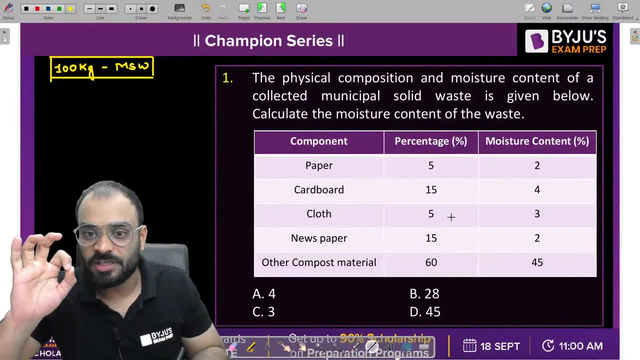 Let us suppose if the value which is written in this particular column it is in percentage, then you can take it as a 100 kg. But let us suppose the value or the weight, or you can say that the mass of the component is written over here. So you have to consider that particular weight, only Right. And if you add all the weight or all the masses you will get the total sample size. But right now they have mentioned the value in terms of percentage. So that's why you have to consider 100 kg. 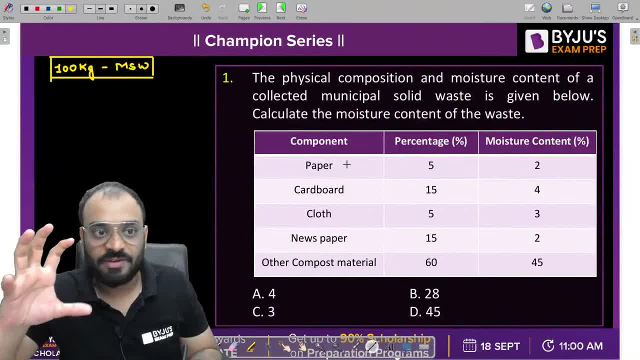 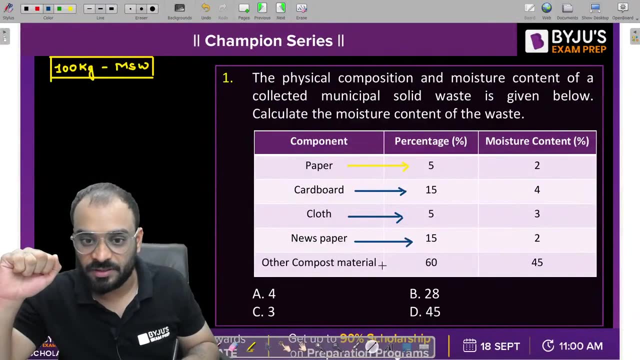 Clear. Now let's understand, guys. We are having a 100 kg of MSW sample in which paper is 5%, Then cardboard. Cardboard is 15%, Okay. Then we have cloth which is 5%, Newspaper, 15% And other composed material. that is basically 60%. Now, guys, if you add all the values, you will get 100% as answer. Correct, But you know that, guys, if it is in percentage, if you take the percentage of this person, 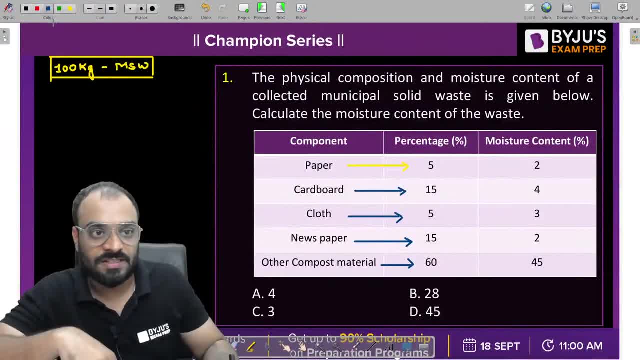 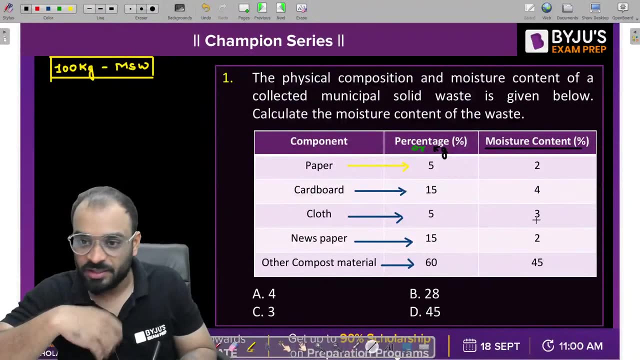 It will remain same in terms of kg also. So can I say that, guys, this value is nothing, as it is also kg. This value is nothing as it is kg also. Okay, The second thing which is written over here, guys, that is basically moisture content, which is in percentage. So 2%, 4%. Then we have 3%, 2% and 45%. Now our task is to find out the dry weight of, or dry mass of, each and every component. I am drawing over here, guys, 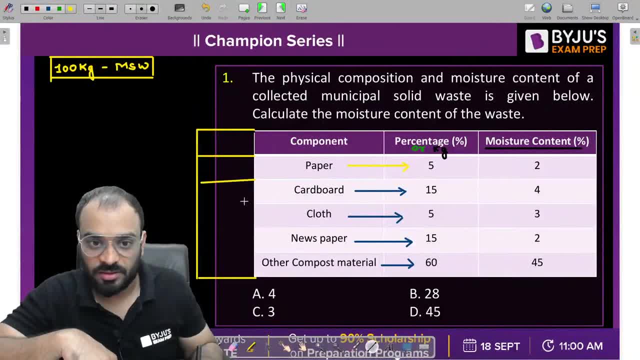 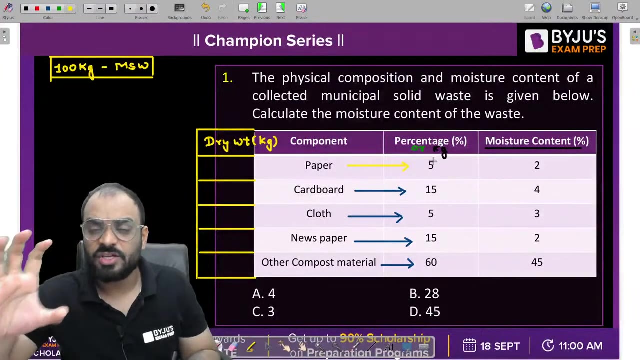 I am writing that particular dry weight in this particular column, The dry weight of each and every component we need to find out. Okay. So, guys, ready with your calculator and try to calculate it. Okay, I am explaining how we can calculate it. Dry weight, which is in kg. Okay, Now, guys, tell me the 5 kg of paper we are having. out of 5 kg, 2% is moisture. 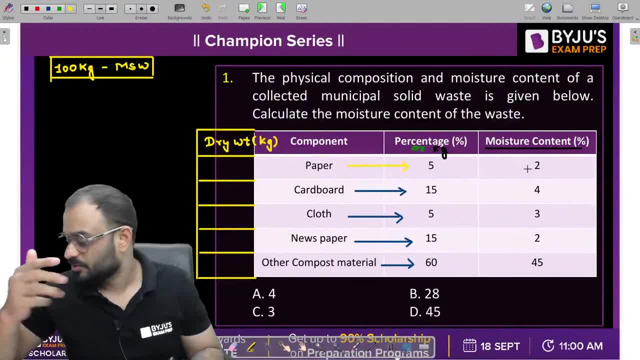 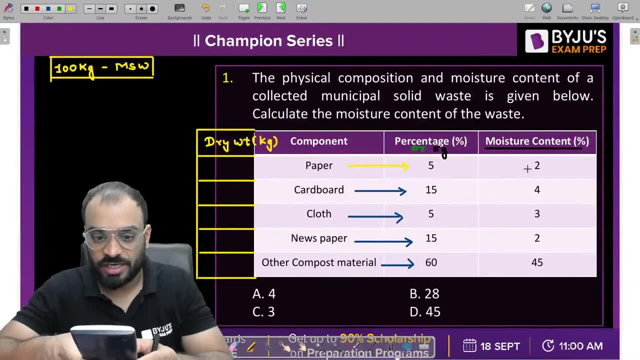 Dry weight is what? 98% is the dry weight. So you can write here 98, or you can write in this way also: 100-2 right: 100-moisture content divided by 100, then multiply by 5. So how much you are getting. 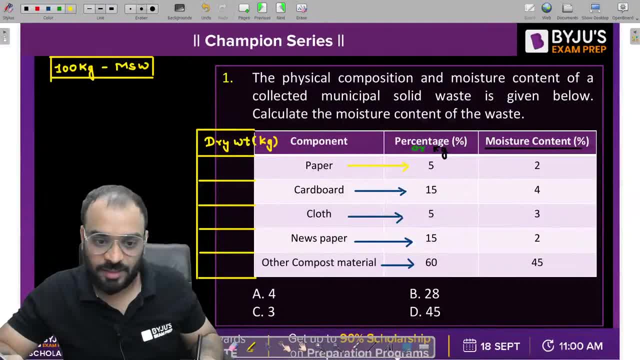 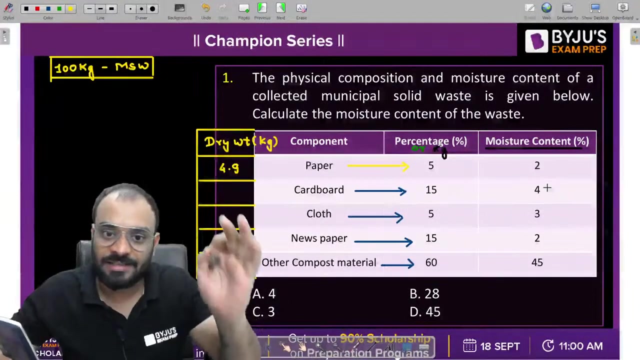 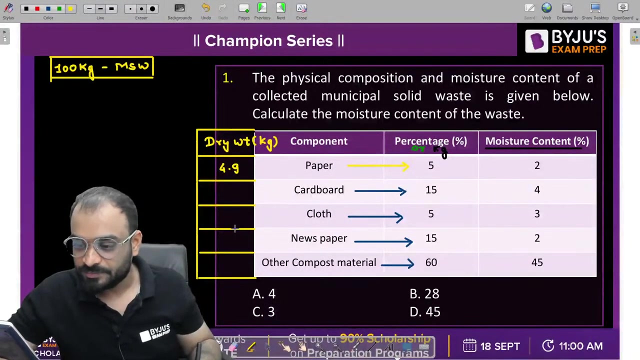 Okay, guys, I will also say in Hindi, but this channel is related to the English, But if you want to understand something in Hindi, I will explain, No issue, Okay, Okay. So let's understand, guys. the further thing: This is basically 4.9 kg Clear If we talk about cardboard. So in case of cardboard, we are having 4% as a moisture content, Right? So out of 15 kg, 4% is moisture. then I can say that 96% is what Your dry weight. So let's take 96% of 15 kg. How much it is 14.4.. 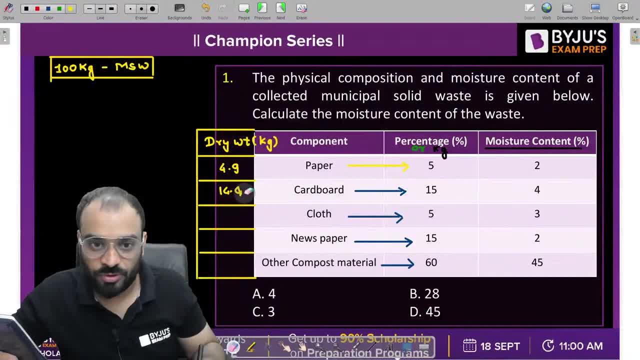 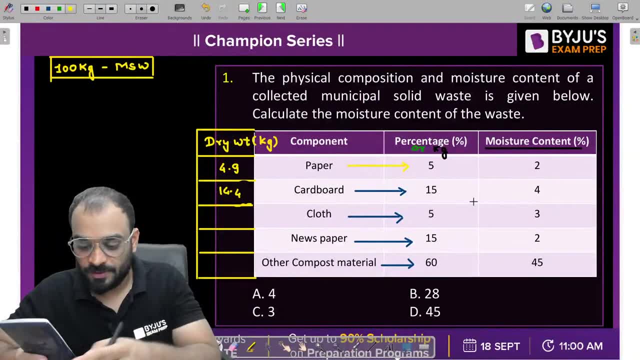 Okay, 14.4.. Okay, sir. Now what about cloth? 3% is moisture, So 97% is dry weight of 5 kg. It is equal to 4.85.. Then we have newspaper 0.98 multiplied by 15.. So we are getting a value of 14.7.. 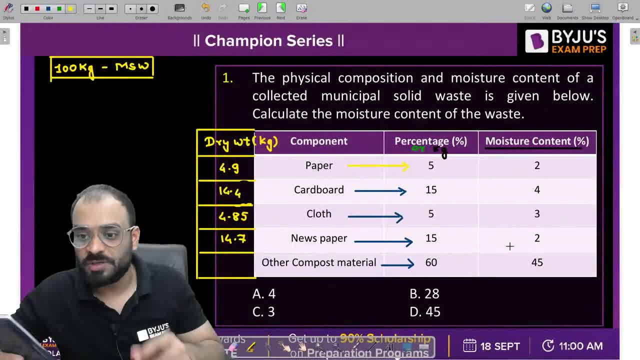 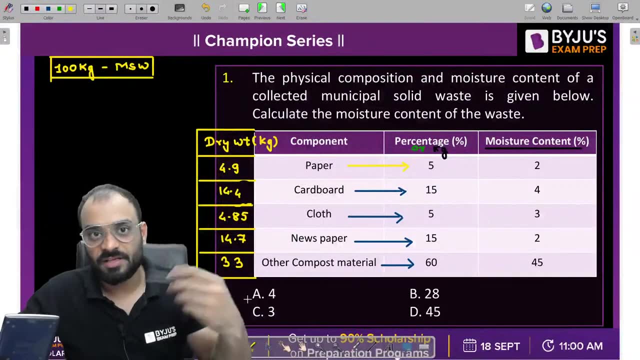 The next one is other composed material. So, guys, it is 55%, which is basically The dry weight of the 60 kg, So 33.. We are getting 33 over here Daily class chalega Pache kal aur hai Phir uske baad hamare paas. next time, jab bhi hoga, I will tell you about it, Okay. 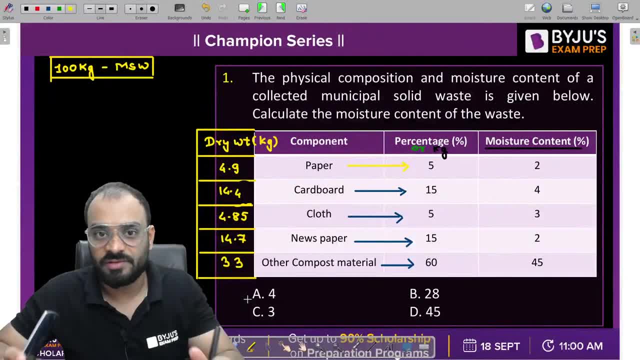 So just what you have to do? you have to just join the telegram channel in which I will share the link that you can get the information of the classes also Right. So in this particular series I am taking the RCC also as well as the structure analysis. So in those classes you will understand the complete structure as well as the RCC part. 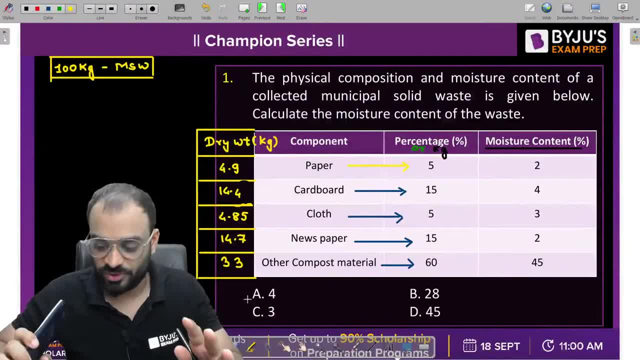 Whatever topics are important for your GATE examination I will discuss. Okay, Chali. So let's add all the value, guys, to calculate the dry weight: 4.9, SMS, 14.4th plus 4.85, Books plus 14.7.. Then we have 33.. 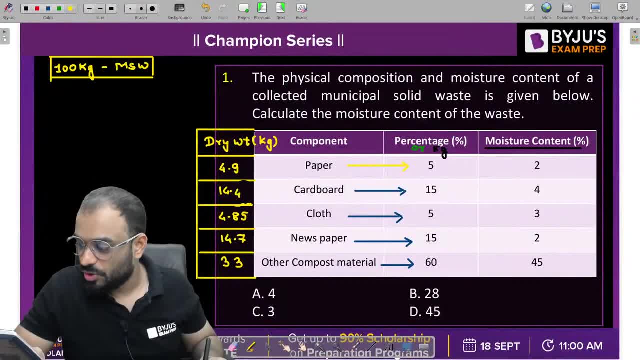 So right now we are getting the dry weight of the sample. it is equal to 71.85 kg. Ok, Now how you can calculate problem. So frequent analysis of Brother K. So you should have something like a number on these sites. They don't call it To himself time. sehr obSchnelle bu pass방. 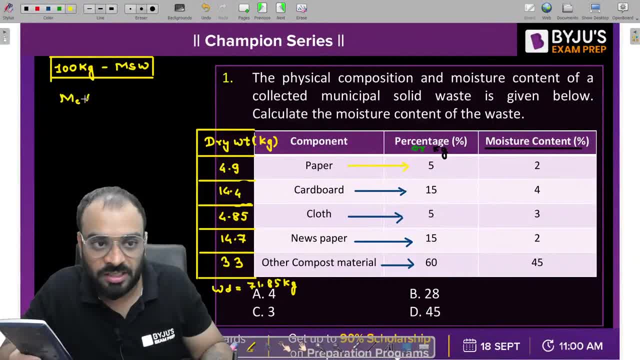 can calculate the moisture contain. moisture contain in terms of percentage can be written as wet weight minus dry weight divided by wet weight multiplied by 100. this is the formula which you have to use, right? what is WW? that is, the wet weight. or you can say that the normal weight of your sample. 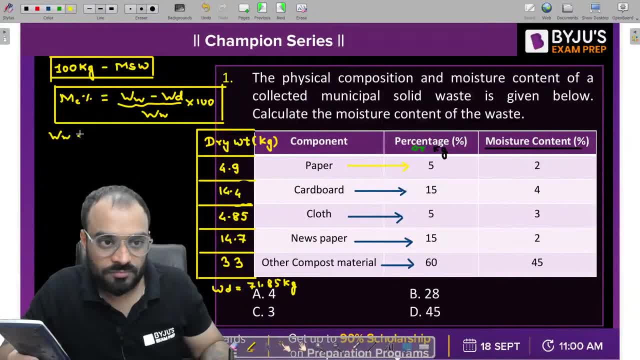 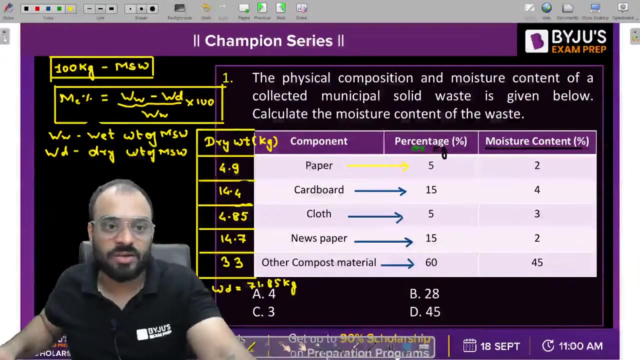 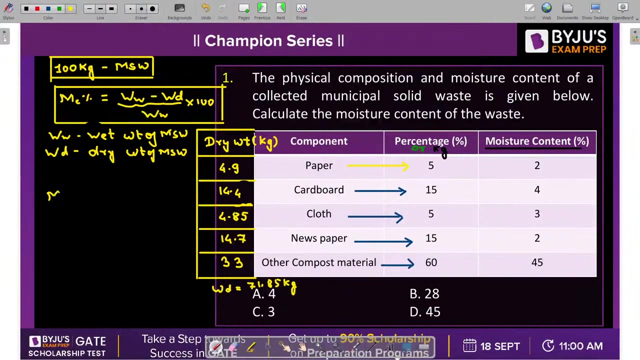 okay, of MSW. and then we have dry weight, which is basically WD, so you can write here dry weight of MSW, here now, guys, it is very easy to calculate the moisture contain. okay, let me hide myself. so moisture contain, which is in percentage, it is equal to. 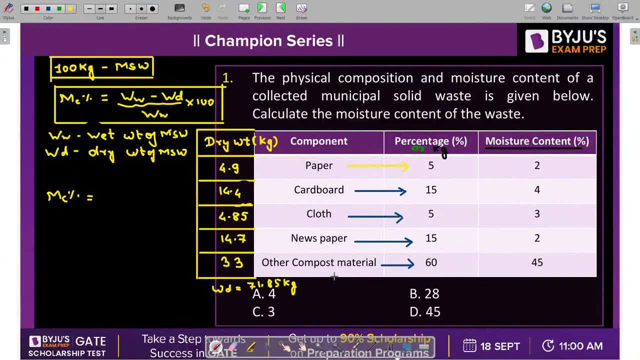 you it is equal to wet weight. wet weight is equal to how much it is 100 kg, correct? it is 100 kg minus dry weight. dry weight is equal to 71.85. then divided by 100 again and multiply by 100, you will get the result. to calculate it: 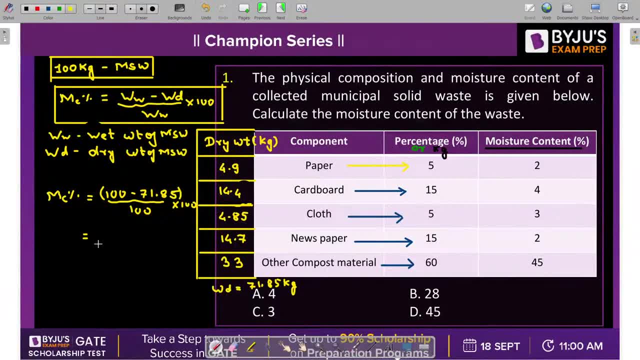 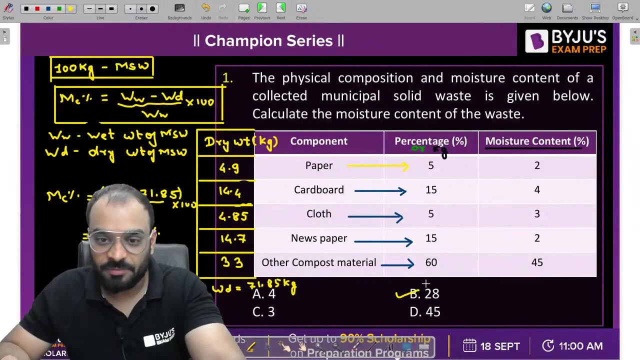 how much you are getting, please let me know. hundred minus 71.85. okay, so, guys, we are getting a value of 20. the third problem: if you are getting a result of work, what is the current answer for the problem? so, guys, we are getting a value of. 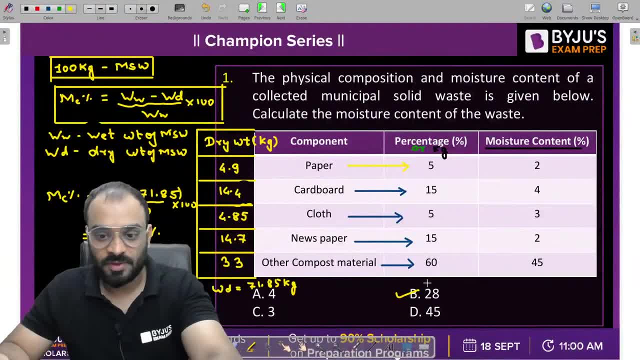 28, point one, five percent. now tell me which is the correct answer: jicker, very nice. these are the great answer. very nice. what about other students? please let me know. guys, between a shaker, so B is the correct answer for the problem. it is twenty eight percent, right. 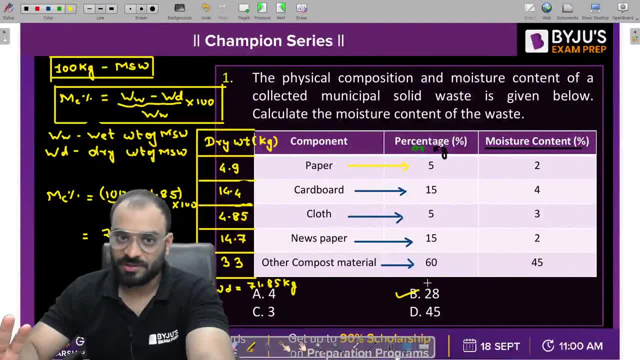 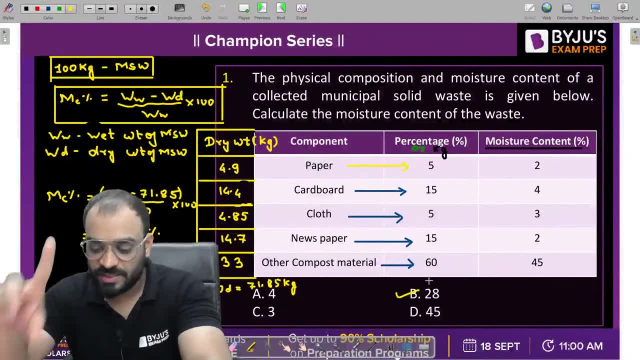 this is the only option which we can take over. here is the bad answer for the problem now. now, guys, the next question. it is related to one mark. now, this particular problem, which is question number one, which we have solved, it is basically two mark problem. now let's see the one mark. 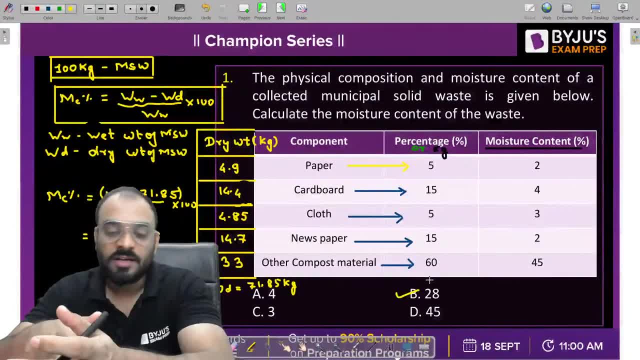 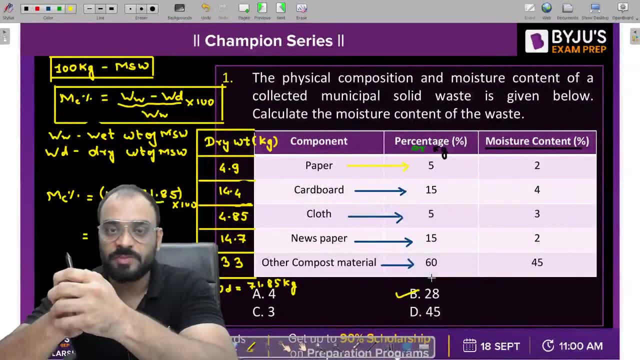 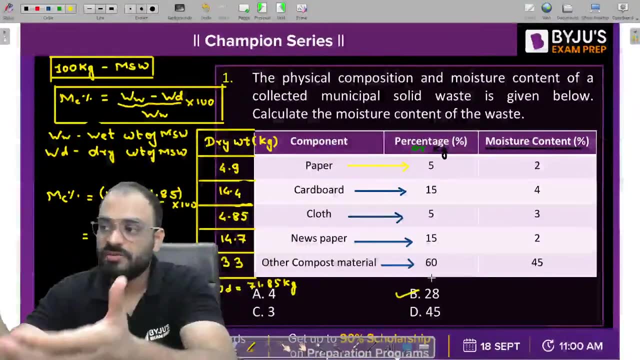 problem also. yes, raga, in case of soil mechanics the formula is different. i can understand, but in case of solid waste management, what you have to do, basically, you need to calculate the moisture contained with respect to the initial weight- of what initial weight? of your solid waste, right so? 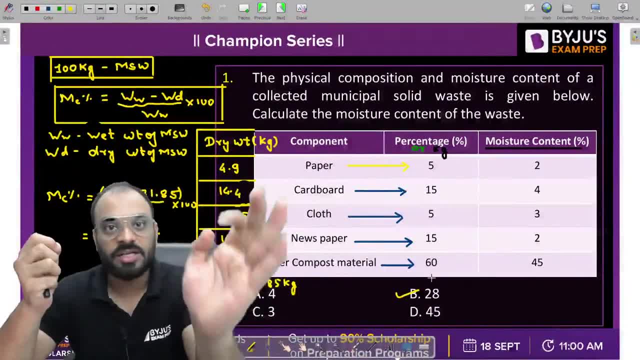 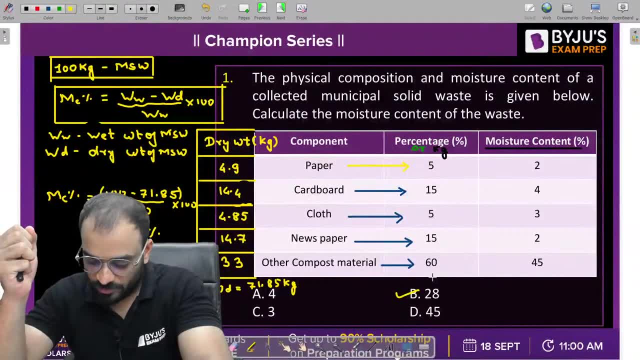 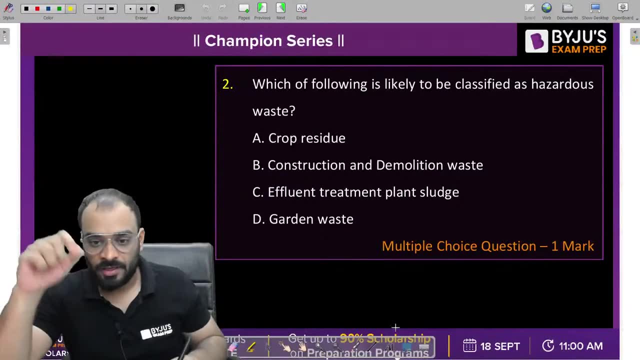 in this particular case, you have to use the wet weight in the denominator, always, not the dry weight. okay, very nice. next question, guys. in front of you this is basically one mark problem, right? you may also get one mark question from the solid waste management in the gate examination. so now tell me the correct answer for this particular problem, guys. 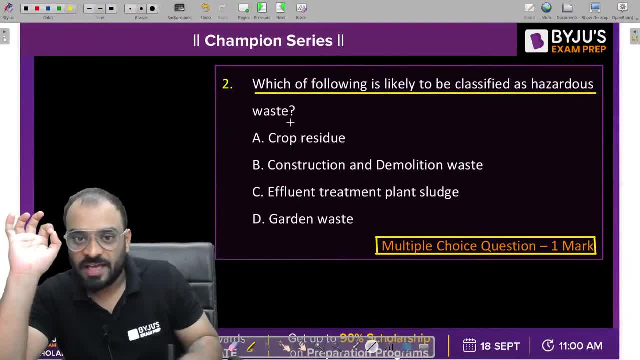 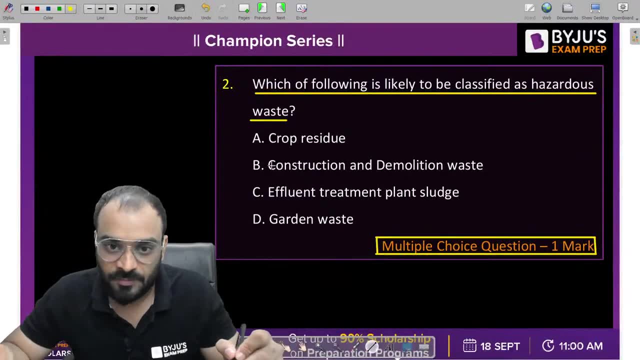 which of the following is likely to be classified as a hazardous waste? which particular waste you will consider as a hazardous? that is the question. whose concentration is harmful for us right now? tell me, guys, which particular waste is to be classified as a hazardous waste. that is the problem. 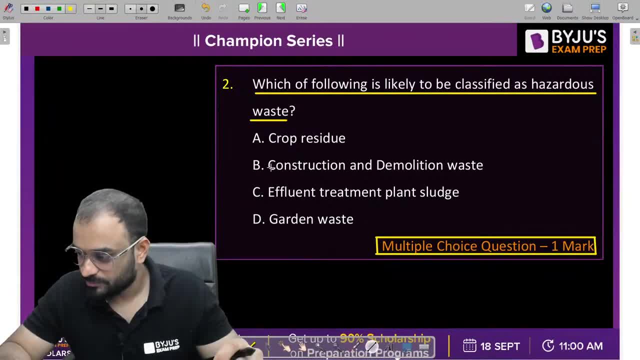 so the answer is c, very nice, c, haskar, guru, b, shakhar b. okay guys, hazardous means what? if the concentration of such type of waste is present in our solid waste, then it is dangerous, right, it is dangerous. right now, tell me guys, if you have a crop residue, then it is an organic matter there. 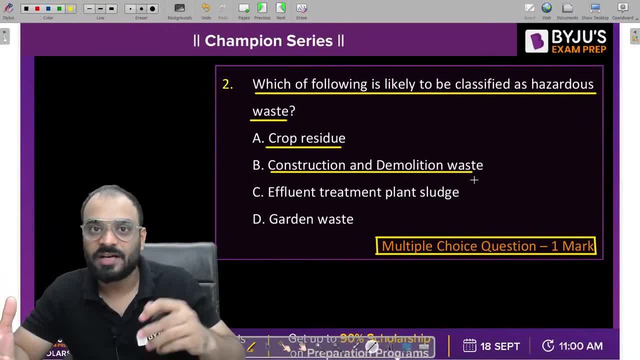 is no issue if it is a construction or demolition waste. that is nothing, as it cannot be getting, it cannot get degraded as well. as such type of waste is present, nearby to us also, guys, it will not give some harmful effect to us, right? so that is also not a hazardous one. but if we talk about 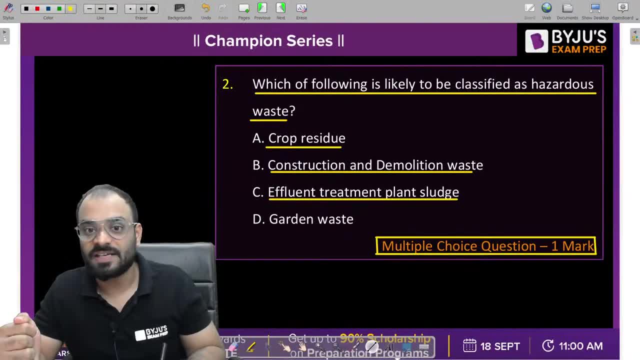 guys. affluent treatment plant, sludge what it is exactly. what is etp? etp is nothing, as it is the treatment plant which is trying to treat the industrial wastewater. this particular treatment plant is to be used for the treatment of the waste, which is the treatment of the waste, which is the 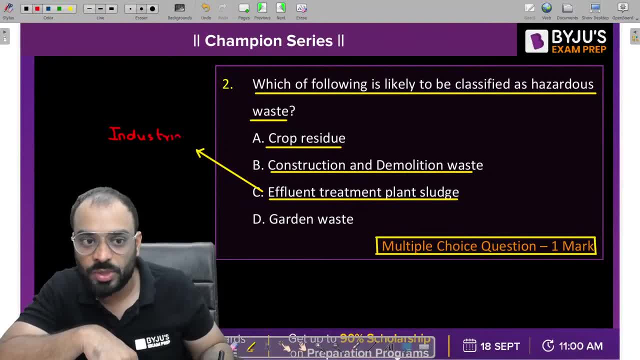 harmful when we are trying to treat the industrial wastewater. now, guys, industrial wastewater is carrying lot of chemical, yes or no, right? whatever wastewater we are having from the industry, it contain lot of chemicals. now, these chemical will also present in the sludge which is generated by the etp, right? so that's why, guys, such type of waste or such type of sludge is hazardous in. 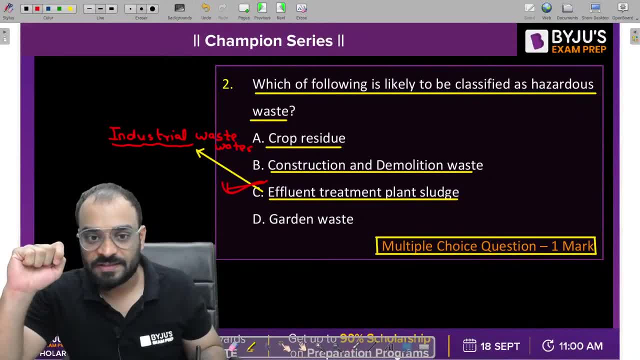 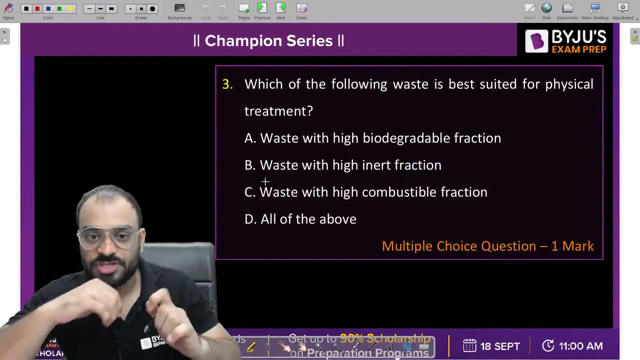 nature. that's why c is the correct answer. that's why c is the correct answer for the problem. clear, clear. so, guru shekhar mithun, all of you are able to understand, right? c is the correct answer for the problem. next question: again, it is a one mark problem- we are having some msq also, guys- which is basically two mark question. 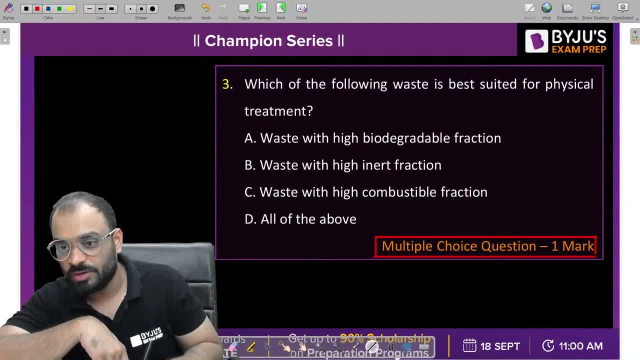 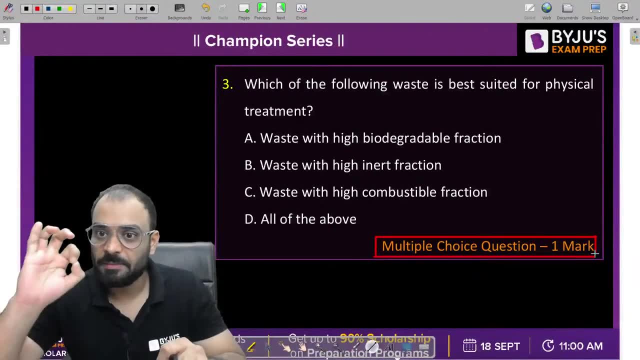 i will show you that also. mcq question: one mark. okay, tell me the answer of this one also. which of the following waste is the correct answer for the problem c? is the correct answer for the problem d is best suited for the physical treatment? which particular waste you can treat by the physical? 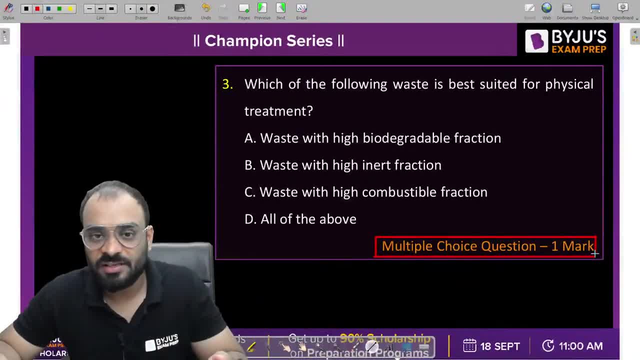 treatment process. that is the question now: what is physical? physical is nothing, as it is the process in which physical forces are dominating right, like sedimentation, gravity settling right. so these type of things are physical treatment based. okay, dinesh d, all of the above. okay, bhaskar b, very nice. 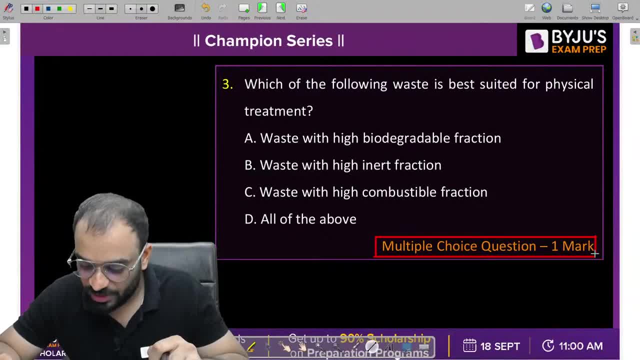 visheshwar d. okay, what about other student? please let me know the correct answer, guys, from your side. what about the student? please let me know, guys, which one is the correct answer. if you know the answer, please let me know. shekhar b. very nice, now tell me, guys, if we talk about. 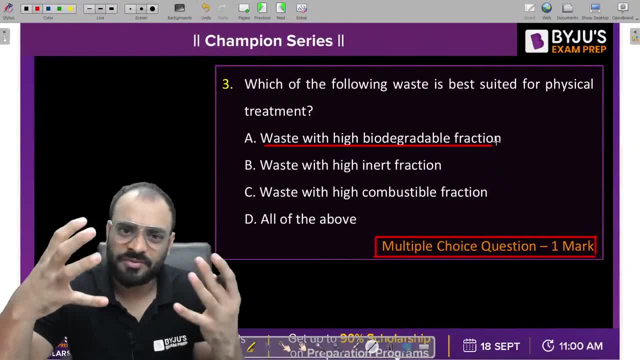 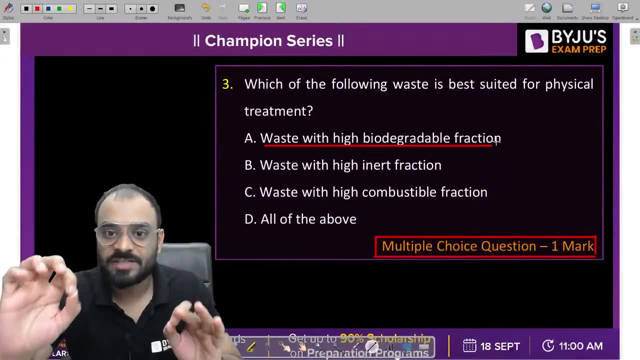 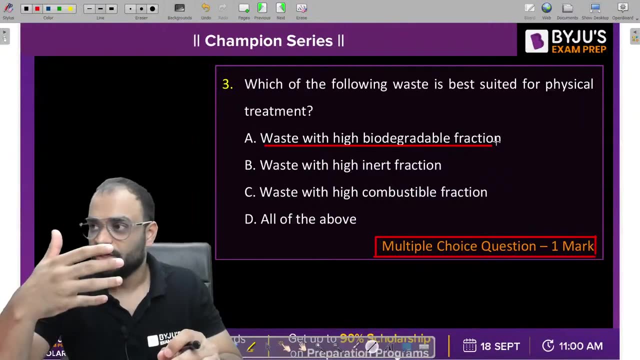 the biodegradable fraction. let us suppose if you have certain type of waste in which high concentration of biodegradable fraction is there, it is better to treat such type of waste by biological process, not the physical process. physical process means what you can separate it by the separation process. 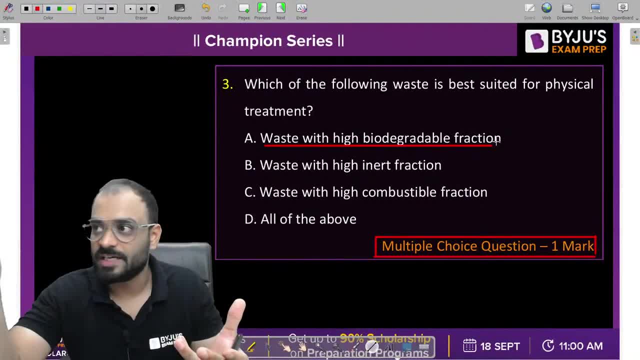 you can uh, separate it by gravity forces also, like sedimentation tank and etc. right. or you can reduce the size of the particle. that can be a physical treatment also right. but, guys, if we have the high biodegradable concentration in any kind of waste, in such 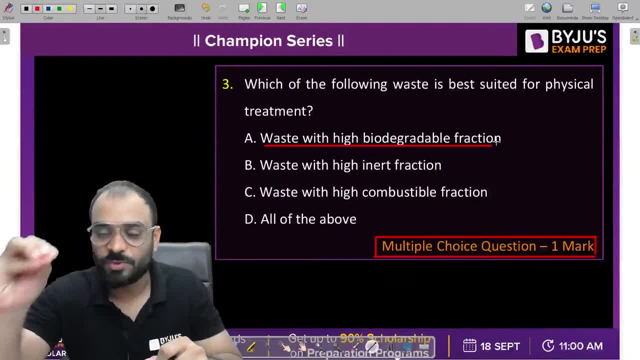 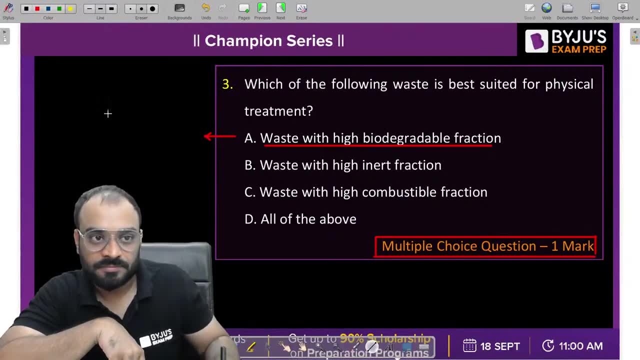 condition you are not able to use the physical treatment. that is not the best process for this particular concentration. we have to use the biological treatment, for the physical one can be treated by the biological treatment part. now, what is biological, sir, biological treatment? what it is exactly? basically, guys, in this particular case, if you have the plant, 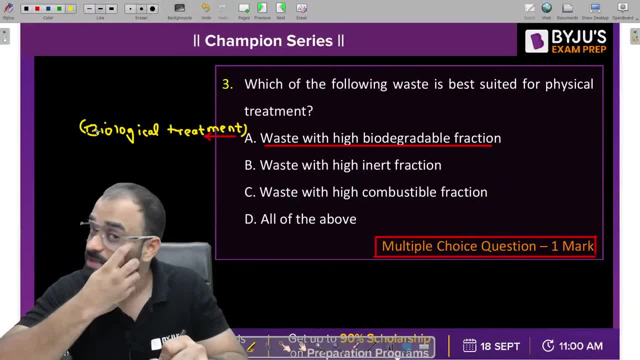 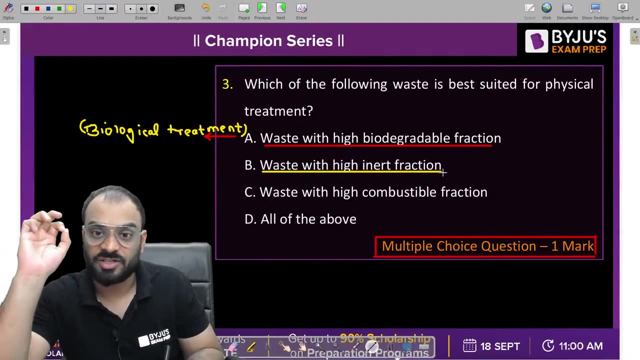 case we are trying to use some microorganism which is trying to consume such type of organic matter so that it can reduce in concentration as well as it can degrade in some other form. right, that is the first. now, guys, if we talk about the waste which is having high inert fraction, inert fraction means 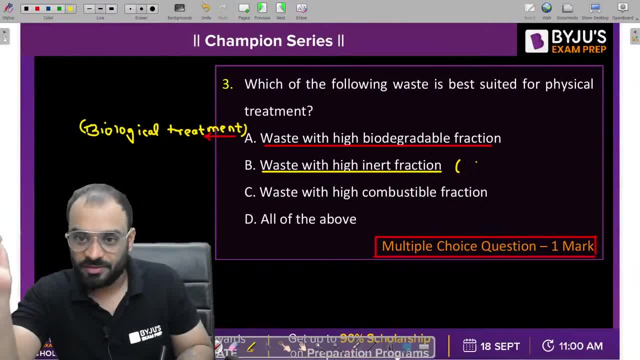 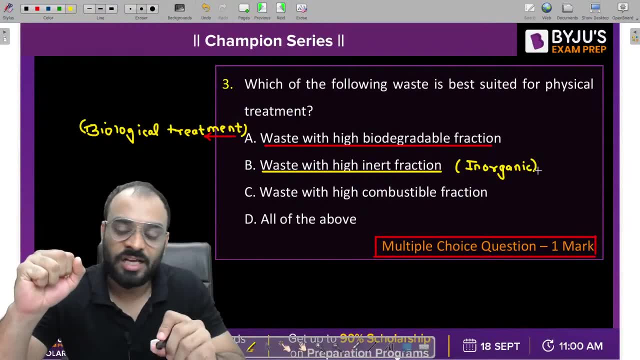 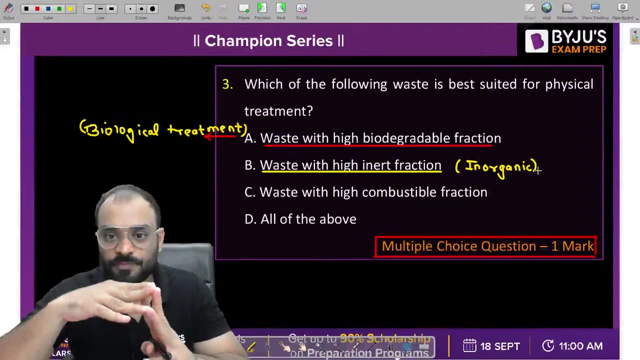 which is inorganic in nature, that cannot be degraded, right? which is basically inorganic in nature? now, if it is inorganic type of matter, now tell me guys, it cannot be degraded by any microorganism. yes, we are not able to reuse it. also, or let us suppose, guys, if we have inorganic or 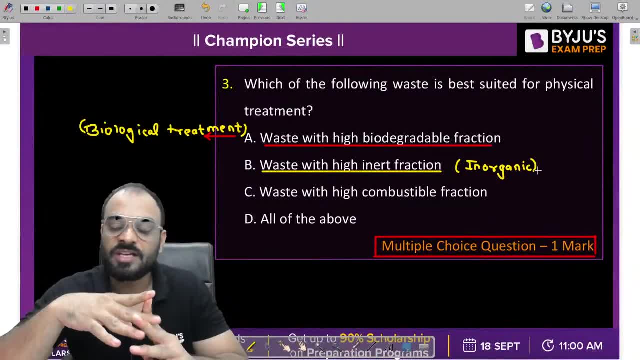 inert fraction, like sand, silt and etc. so such type of particle cannot be useful for our further manifracturing process. or you can say that we are not able to reuse it. we can dump it, right, we can dump it, but, guys, such type of impurity. 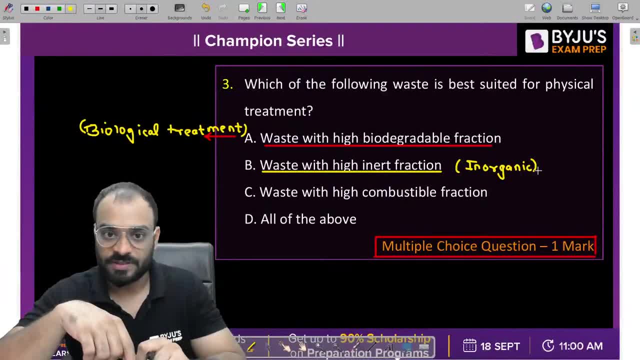 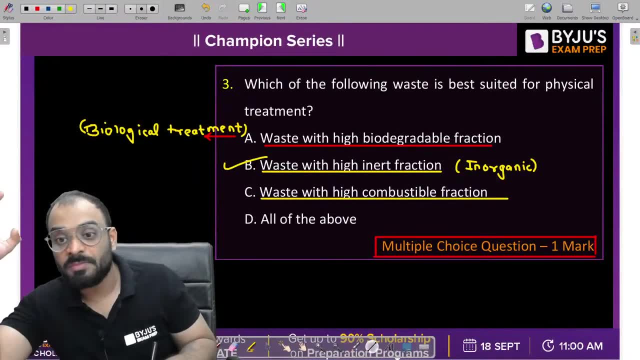 can be degraded by any microorganism. yes, we are not able to reuse it. we can dump it. right, we can be separated by using the physical treatment. that's why b is the correct answer for the problem. now tell me, guys, if you have a waste which is having high combustible fraction, like paper. 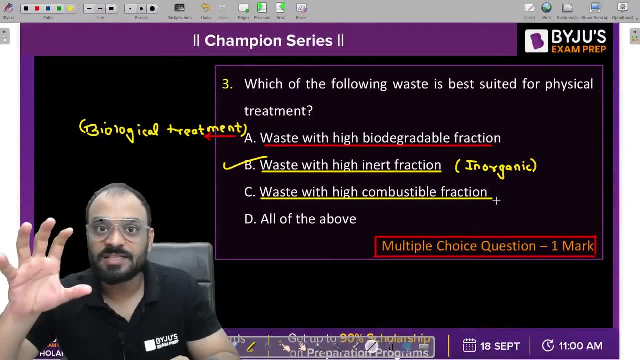 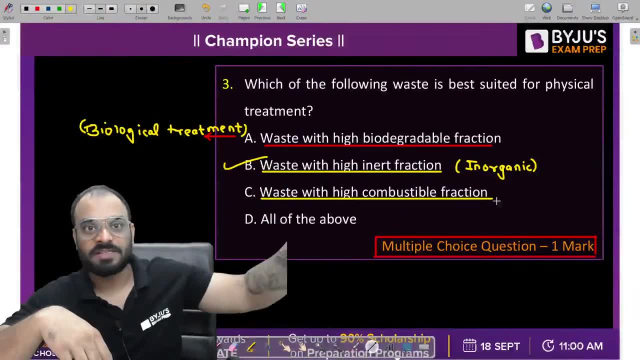 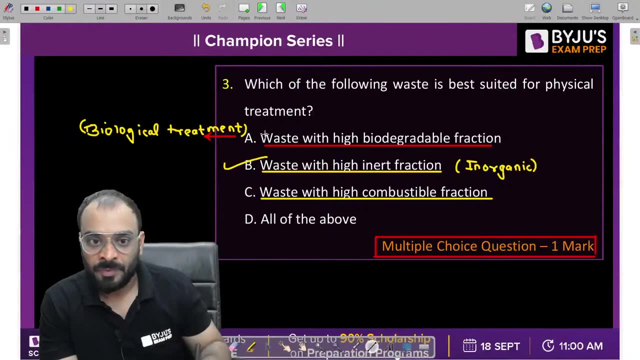 right, polythene, plastics and etc. so in such case you need to use the chemical process. chemical process means what we are trying to use- the fire over here, guys, the presence of oxygen. that is basically chemical process. so this particular waste can be treated by biological, this waste can be treated by the physical and this waste can be treated by the chemical. 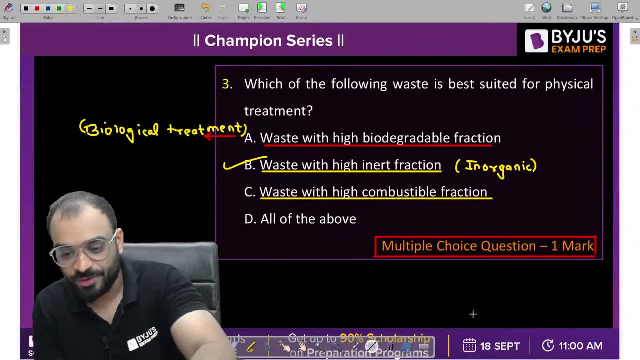 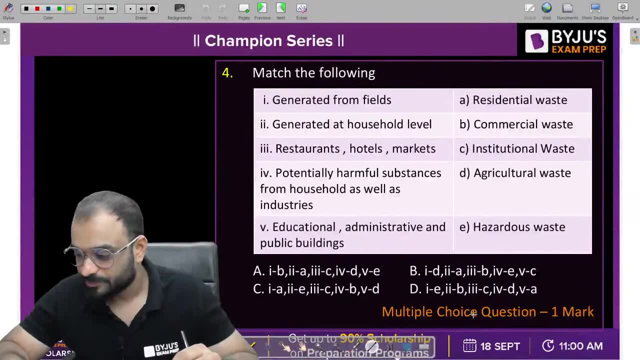 and that's why b is the answer for the problem. clear, okay, very nice. next question in front of you. please match the correct answer. match the correct answer. be careful, guys. okay, and let me know the correct answer for the problem. you just need to match the column number one and column number two. 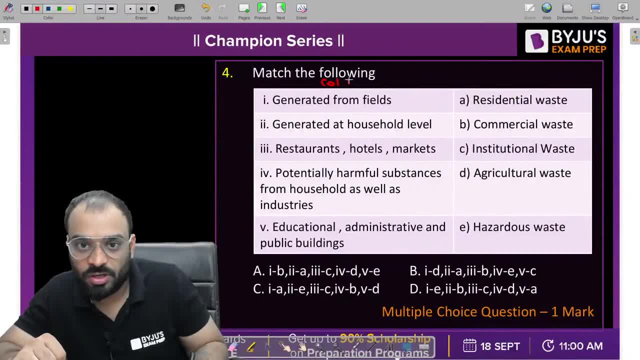 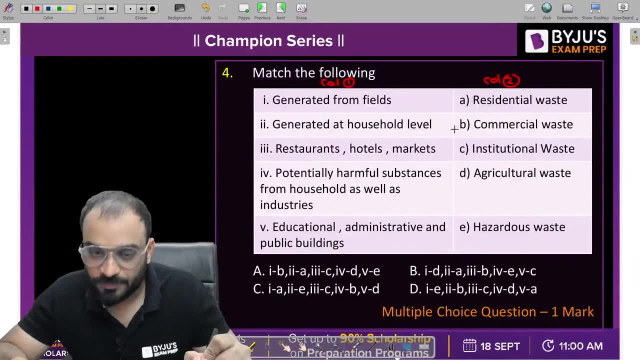 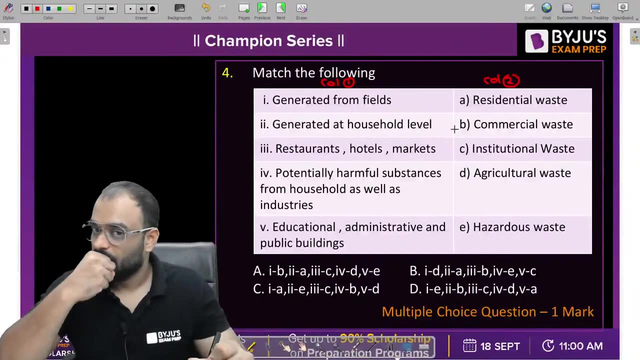 this is basically column number one and this is basically column number two. you have to match both the columns. tell me guys: b guru, b. okay. p is the correct option. okay, bhaskar, visheshwar- b. very nice. what about other students? what do you say, guys? please let me know the correct answer from your. 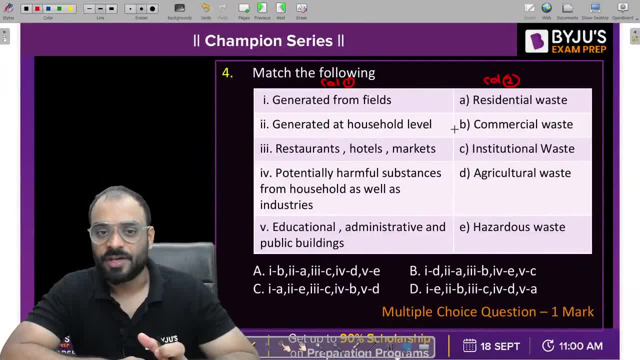 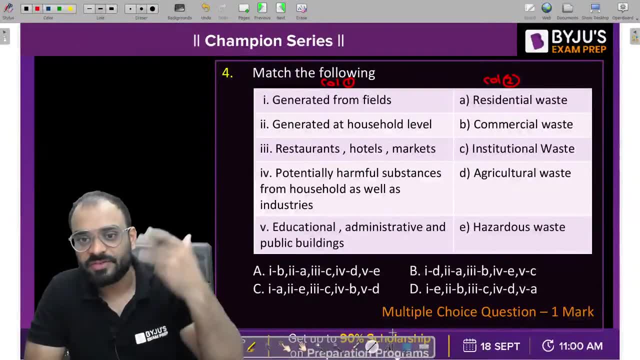 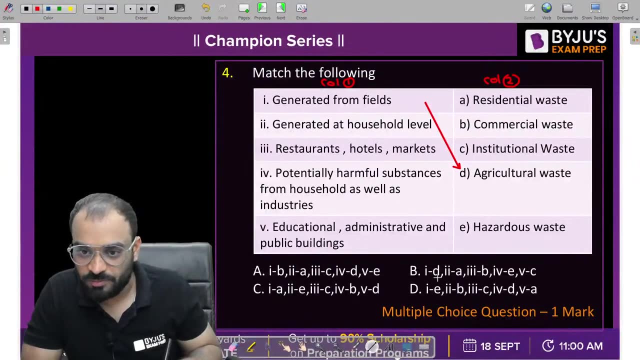 side. okay, now tell me guys what is basically field. field is nothing, as that is your agriculture land, right? so whatever waste which is generated from the field, it is a basically agriculture way. so for first it should be d, for first it should be b, so the only single option is there. 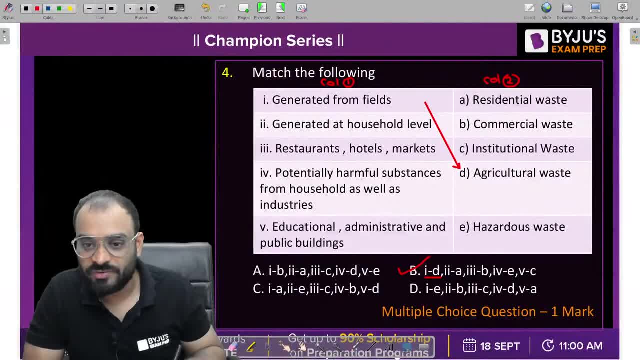 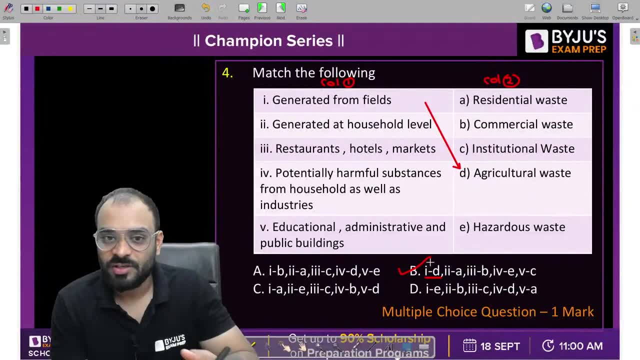 whose answer is for one, it is d, so that's why we will put the answer directly as d. you don't have to check other option right, because it is understood if you have only single option in which the for one it is given as d as a answer, so we can take that particular answer directly. 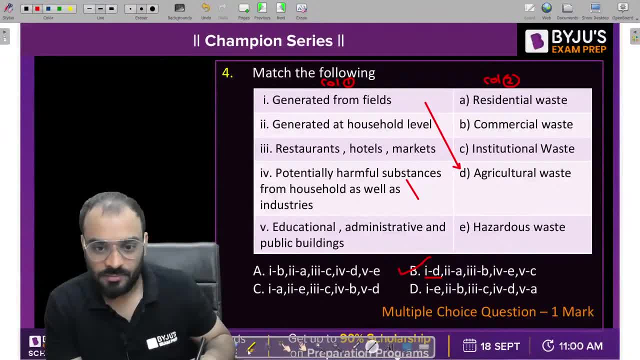 okay, but let's understand the rest of the thing also. let's understand the rest of the thing also. generated at household level, generated as a household level. so it is known as what residential waste for? second, it should be a restaurant, hotel and market restaurant, hotel and market commercial waste. 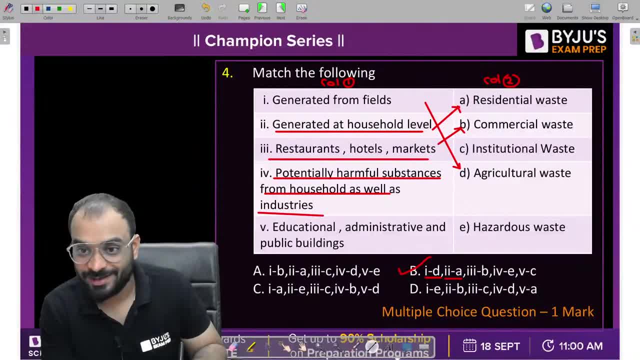 potential harmful substance from the household as well as the industry. so such type of waste is known as the household energy, as a household energy as as a household industry. so such type of waste is known as hazardous waste, educational, public building and etc. so for this it is institutional. 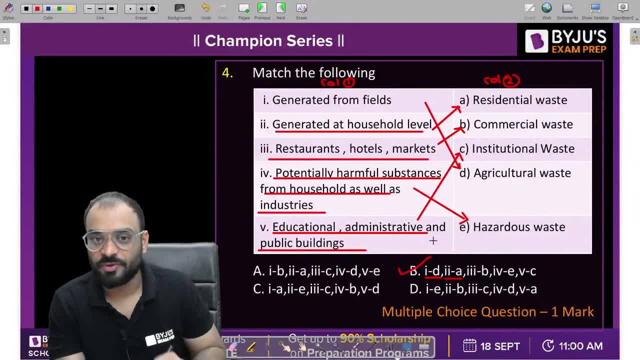 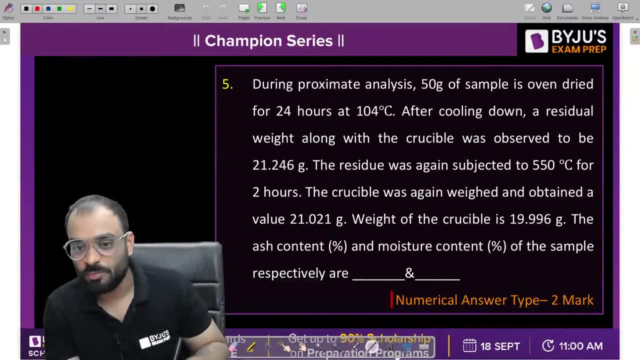 right. so that's why, guys, this is the correct answer for the problem. clear now. the next question is a not type question, which is basically numerical answer type problem in which you need to find out the two things: one is moisture contain and second is your ash contain. 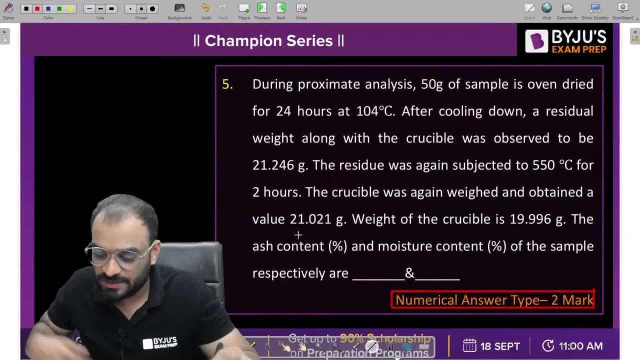 i think it is written as okay. first is ash contain and second is your moisture contain, which you have to find. okay, and the problem is given in front of you. guys, and this is a numerical answer type question, be careful while solving it. be careful, and it is my request, guys: if you enjoy the session, please share it to other student also. 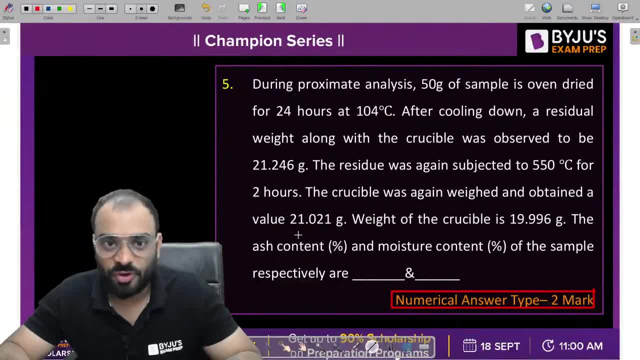 so that they can learn something over here. if it is useful for all of you guys, please share it. okay now, guys, this question is related to the two part. one is to calculate the ash contain and second is to calculate the moisture contain of the right. that is the problem which is given to us now. let's 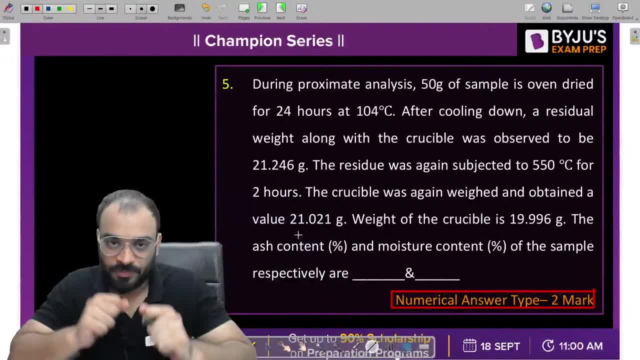 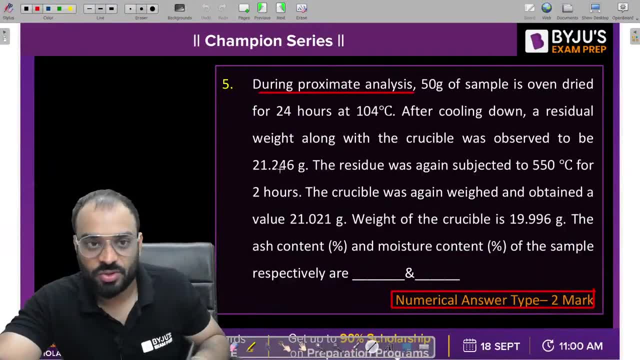 understand how we can solve it and what is the data which is written over here. now, during the proximate analysis, a 50 gram of sample is oven dried, okay. so let's draw a figure over here, guys, so that we can understand the data which is written over here. so let's draw a figure over here. 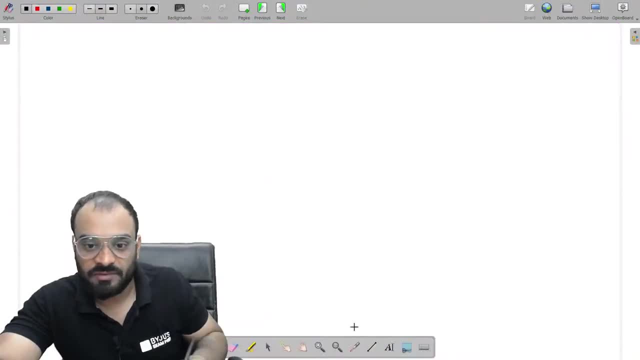 very well what they have given. we have a sample. we have a sample whose weight is equal to how much? whose weight is 50 gram. this weight is 50 gram and this particular sample is put it into the oven at a temperature of 1, 0, 4 degree centigrade here. so let us 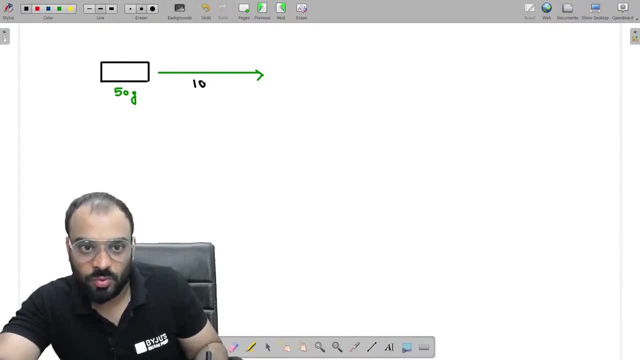 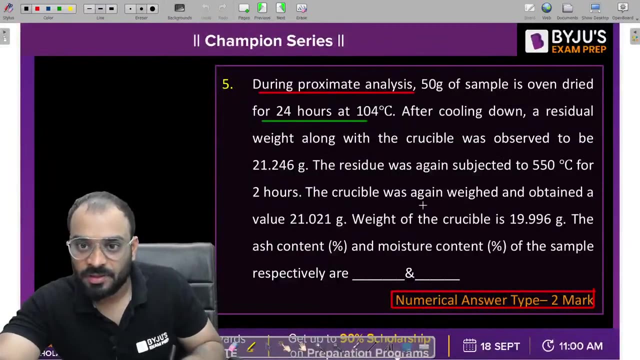 oppose. we have putted in this particular sample at 1 0, 4 degrees centigrade for 24 hours in the oven. now what will happen now after cooling down a residue weight? after cooling down, a residue weight along with the crucible was observed to be this: okay, can i say? 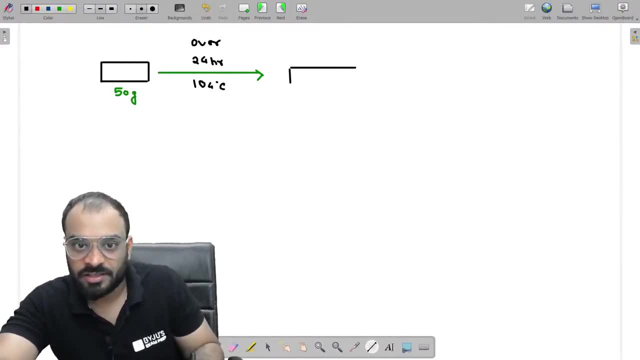 that, guys, the weight which we are getting after oven drying it, that is to be known as dry weight. that is basically dry weight, yes or no? this particular weight is equal to what dry weight? so this value is equal to 21.246 gram. can i say that, guys, this is basically dry weight. 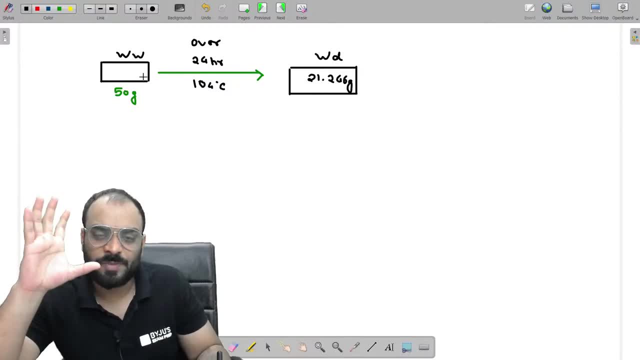 and the weight which you are having is a wet weight. now, in this particular problem, tell me, guys, the weight which you are having in initial, it is the addition of two things: one is the weight of crucible and the weight of sample and in this case, again, guys, we are having 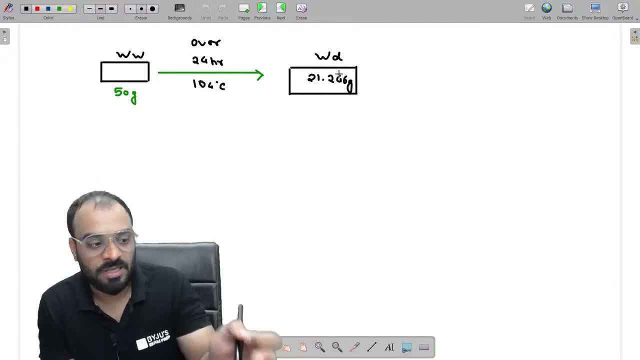 two thing. one is weight of sample, which is dry sample, just weight of crucible. so if i subtract both the value, i will get the direct moisture amount, or you can say that the amount of water which is present in the sample here. so what you have to do, guys, you can use the 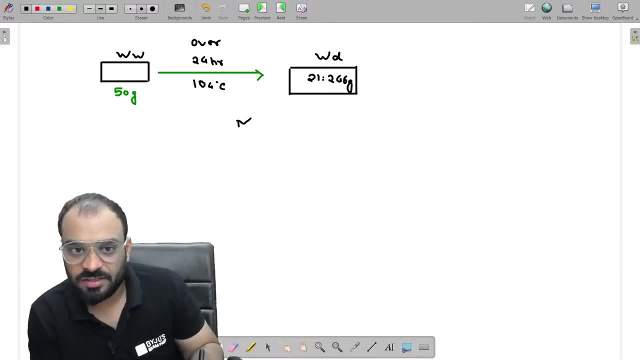 data directly. okay, so let's write the moisture contain over here. we can write here: it should be 50 minus 21, point two, four, six. okay, then divided by and divided by the initial weight, which is 50 and multiplied by 100. sir, assistant sanitary and waste management may be a sub question. 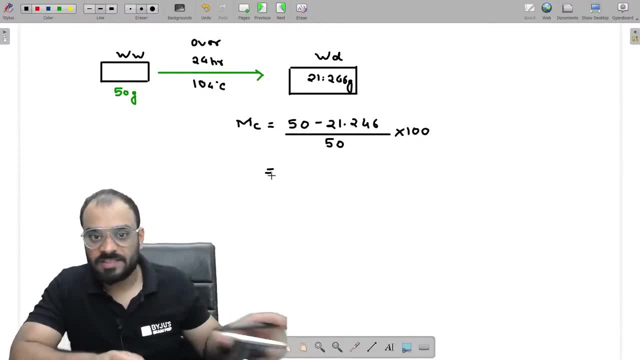 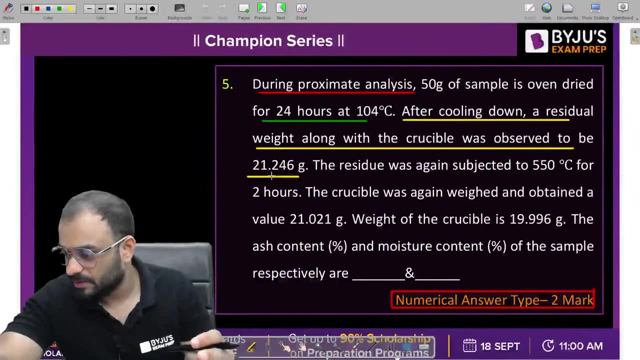 because it is related to the solid waste manager. so please calculate this particular value, how much you are getting, and let me know the answer. wait, uh, just a second, just a second, just a second, uh, just a second. let me check once again, guys, what is the data which is written over here? then we will calculate the further. 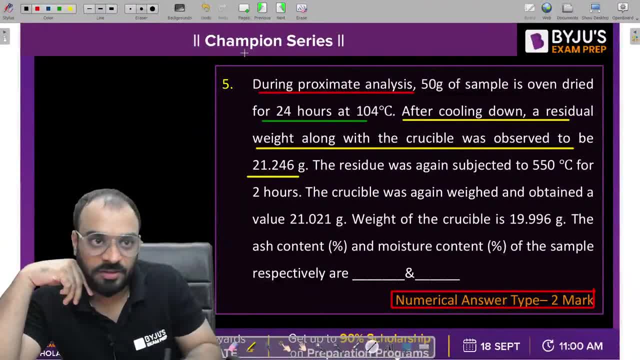 data during the proximate analysis. 50 gram of sample. okay, i think initially the they have given the weight of sample 50 gram. okay, after cooling down a residue weight along the crucible. okay, so, guys, this particular weight which they have written over here, that is basically the wet. 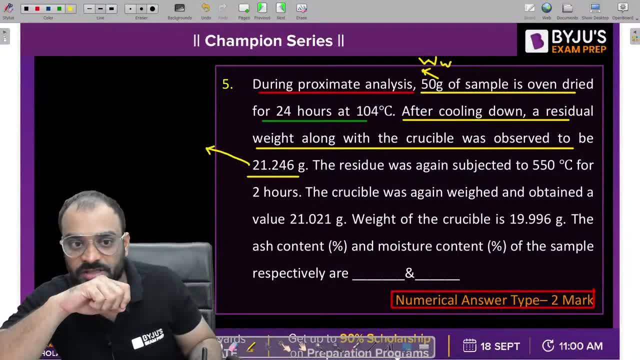 weight of the sample? okay, no problem, but the weight which is written over here, that is not the dry weight completely. you can consider: this particular weight is a dry weight plus weight of crucible, the weight of the crucible in the initial sample. okay, so we need to find out the weight of sample. 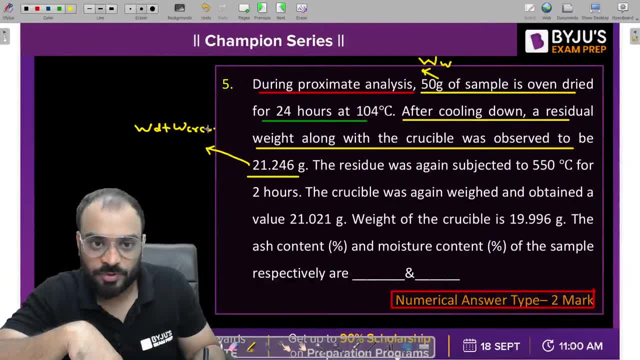 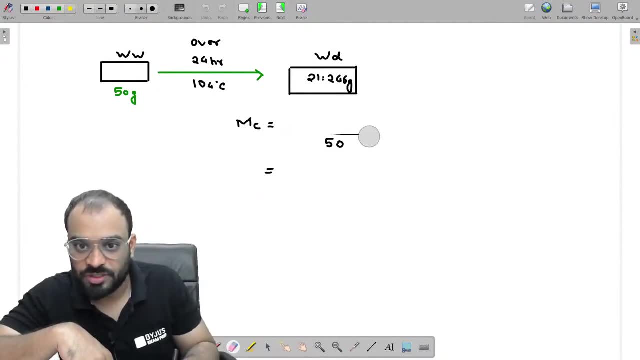 after drying. okay, we will find it out. let us suppose this is basically the weight of crucible plus weight of dry sample. so how much it is? it is 21.246 gram. okay, so, guys, just a second. we need to remove this particular calculation. we need to remove this particular value and this particular 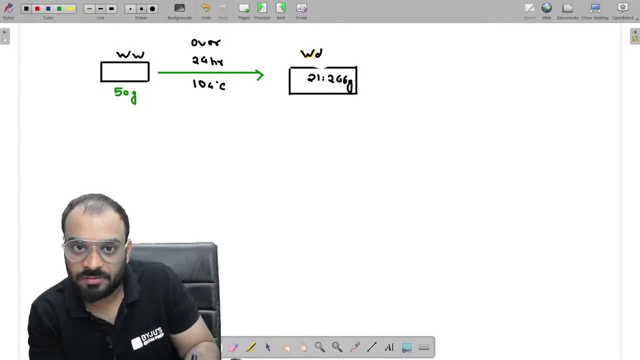 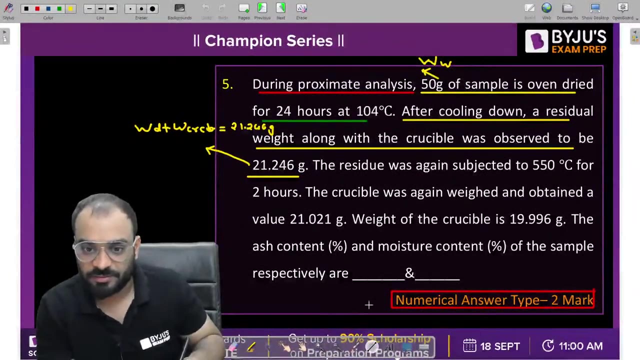 value is basically the dry weight of the sample plus weight of crucible. okay, and this is equal to 21.246 gram. now what you need to do, you need to put this particular value, which is basically the weight of crucible which they have given. weight of crucible: 19.996. so weight of crucible is. 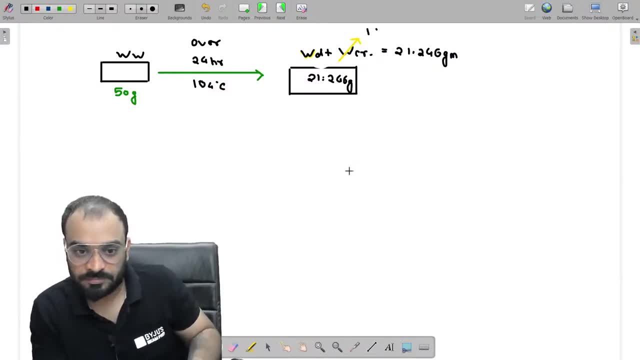 19.996. so what is the value of dry weight? please calculate it. what is the value of dry weight which you are getting? it is coming around 1.25, correct? 1.25 gram. now, guys, let us calculate the moisture contained: wet weight, which is 50, dry weight, which is 1.25 gram, and what is the value of dry weight. 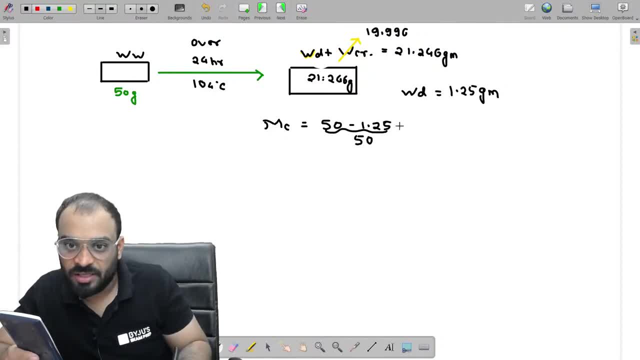 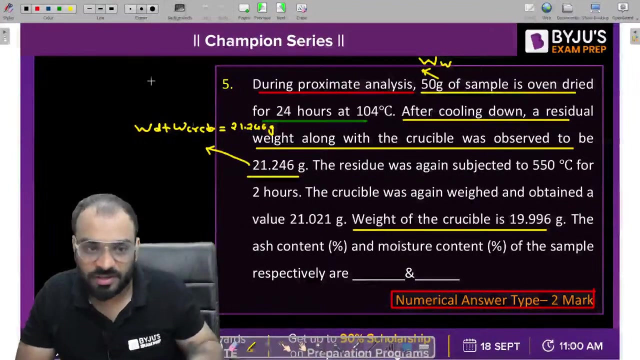 25 divided by wet weight, which is again 50, and multiply by 100, so we are getting a value of 97.5. all of you are getting this particular value. that means the moisture content is equal to how much 97.5 percent. so one of the value you are getting over here, guys, you have to write it in. 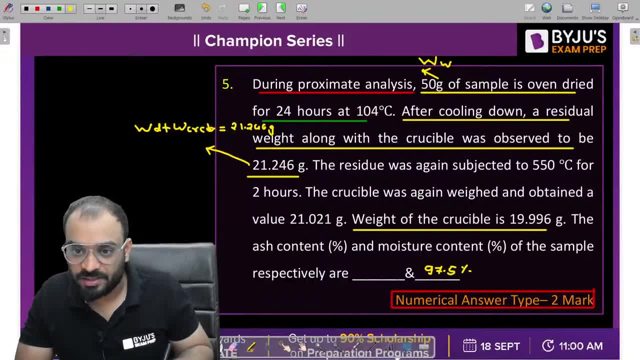 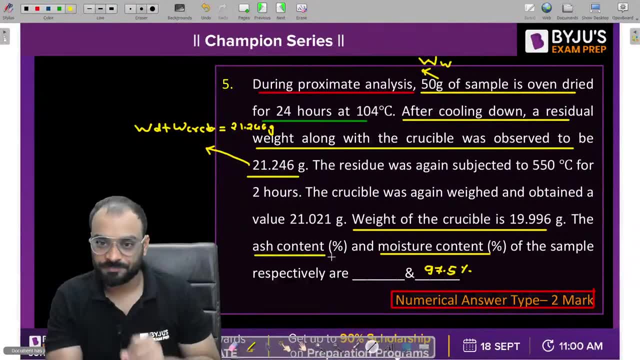 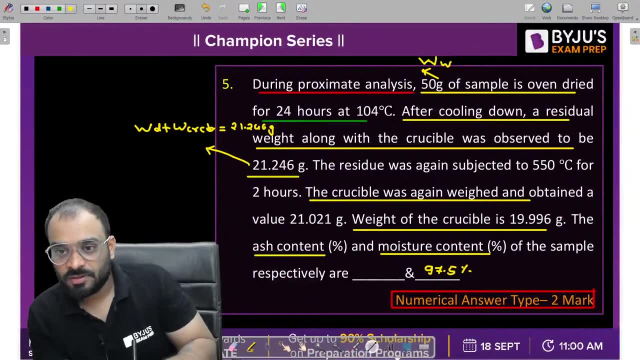 the option also. that is 97.5 percent, which is moisture country. okay, sir. now the question is: we need to calculate the percentage ash also. now let's understand how we can calculate it. now the crucible was again placed into the awful furnace, basically at a temperature of 550 degree. 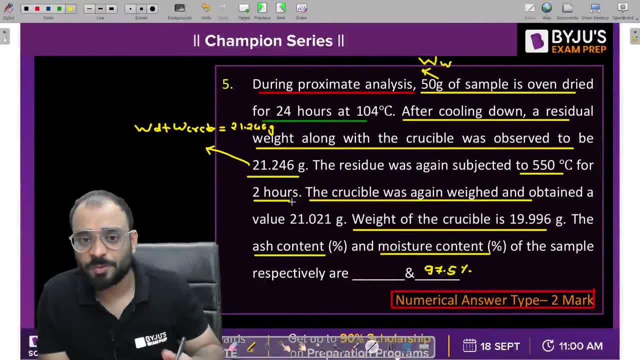 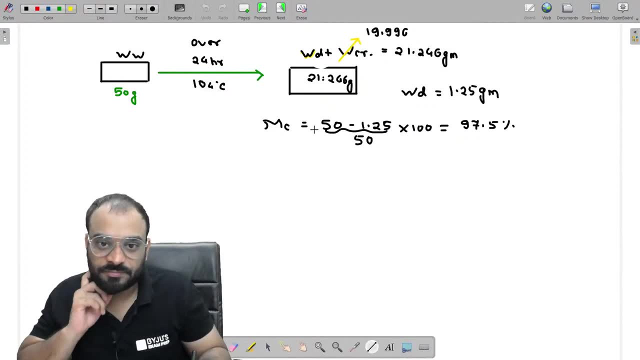 centigrade for two are, after this process, the weight of who, Sibyl and the sample is equal to twenty one point zero to one gram. our task is to find out the percentage ash. now, let's understand these. now, this sample, this sample which is already 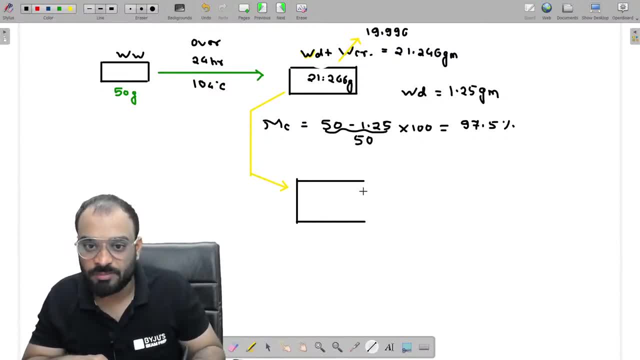 oven-dried. this particular sample is placed into the muffle furnace at a temperature of 550 degree centigrade for two hour, and the weight of the sample is equal to 21.021 gram. so this sample is placed into the muffle furnace at a temperature of 550 degree centigrade for two hours and the 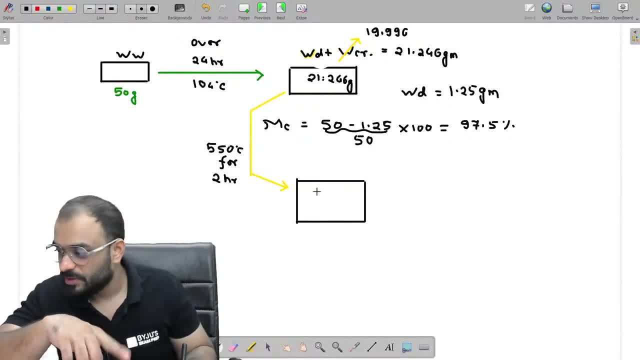 weight of this particular sample is equal to how much it is given to us. twenty one point zero to one gram. now tell me, guys, the weight which you are having after putting it into the muffle furnace. the remaining weight will be nothing, as it is your right so we can write here. this is basically weight. 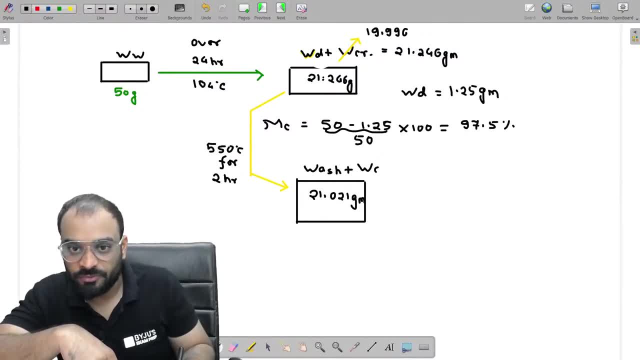 of ash plus weight of crucible and it is equal to twenty one point zero to one gram. so we can write here: this is basically weight of ash plus weight of crucible, and it is equal to twenty one point zero to one gram. so our task is to calculate the weight of ash over right. so weight of ash is equal. 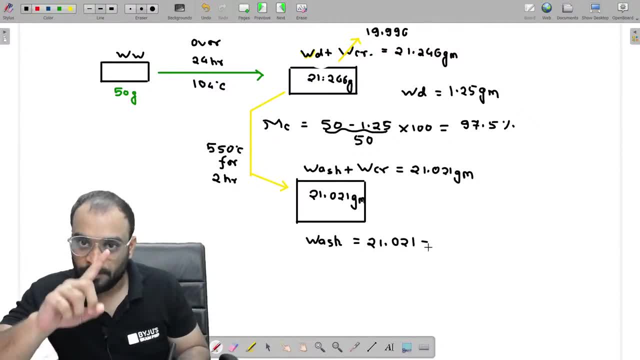 to twenty one point zero to one minus weight of crucible, which is nineteen point nine nine six. please calculate this value, how much you are getting. let me know how much you are getting. it is coming around one point zero to five gram. okay, now we can calculate the percentage ash also. percentage ash is equal to percentage ash is. 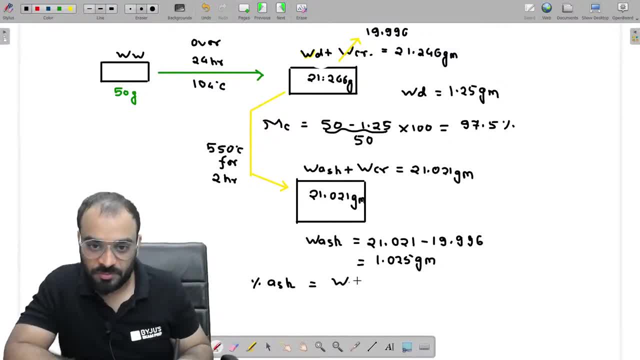 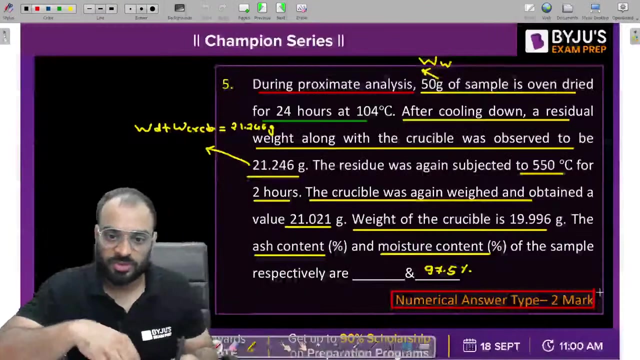 equal to weight of ash. weight of ash divided by total weight multiplied by hundred. so the weight of ash is equal to one point zero to five. total weight of the sample is fifty gram and multiplied by hundred. please calculate this value. so it is coming around: two point zero five percent. two point zero five percent. so that will be the 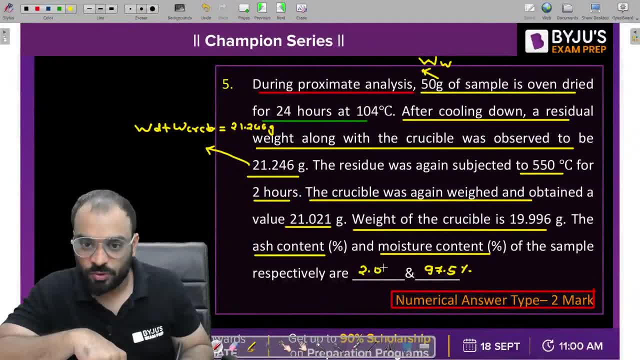 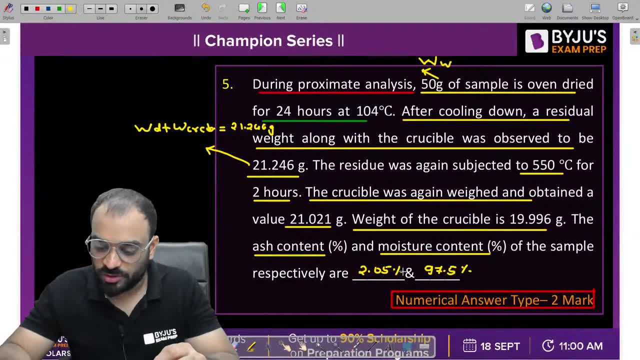 answer. you need to write it in the option. it is two point zero five percent as a percentage ash. now tell me guys, it is crystal clear how to solve such type of question. it is clear to all of you how to solve such type of problem in the examination. 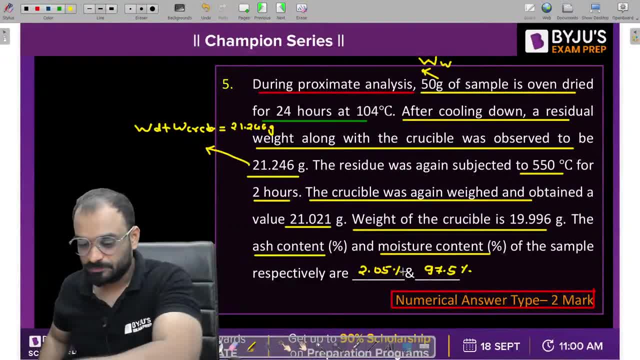 and this problem is going to be solved in the next class. so thank you for watching this video. we will consider this other answer also later and get back to you with an answer in the next class, in the next class. okay, bye guys. now let's understand the next question, which is basically one mark question. let's understand it. 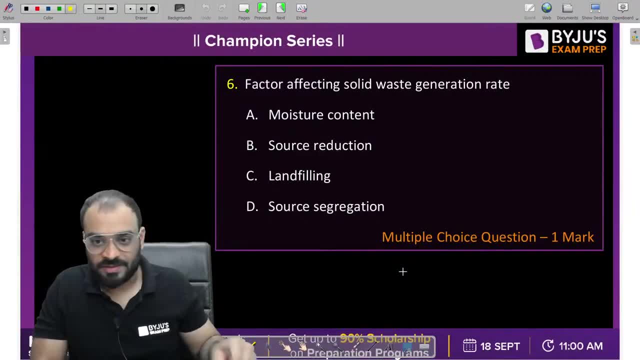 and please let me know the answer from your side. this is a mcq type of question. an mcq ever to. this is mcq one mark problem. you need to tell me, guys, what are the various factor which is affecting it's solid waste generation rate. what are the various factor? this is mcq type question, right, you need. 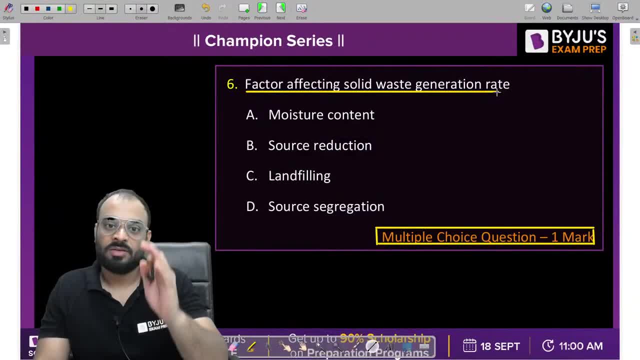 to tell me, guys, which particular factor will affect the solid waste generation rate? that is the question: factor affecting the solid waste generation rate. that is the question b. gudapati b okay. shekhar b. okay. what about other student source reduction? very nice source reduction, some logical question, right? 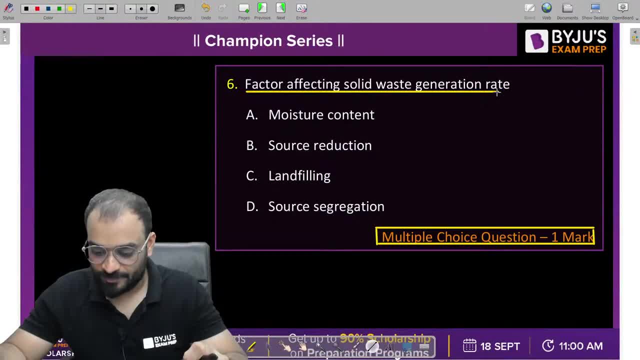 what other student says? the factor which is affecting the solid waste generation rate? b dinesh, b very nice mitun, d okay. source segregation. i will explain each and every option in now. listen, guys. in this particular case, you need to understand what is the question. basically, what are the various factor which can affect the solid waste generation rate? 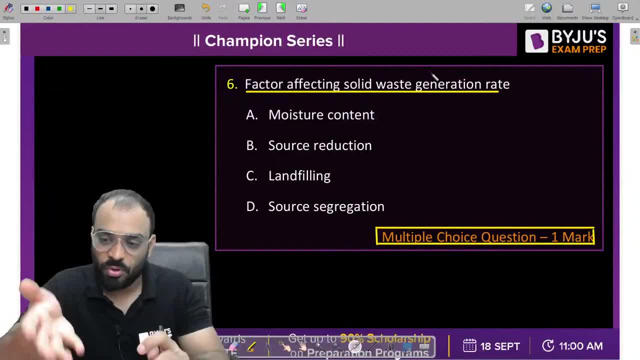 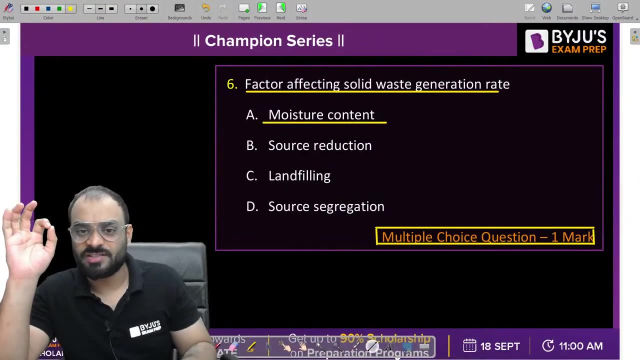 so tell me, guys, whether you want more solid waste generation rate or less solid waste generation. it should be lesser, right? we want to reduce the concentration of solid waste in our environment. that is our main right now. tell me guys, whatever moisture content is there, it doesn't matter, right? 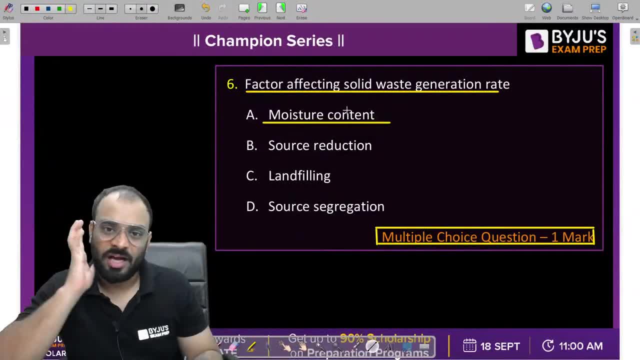 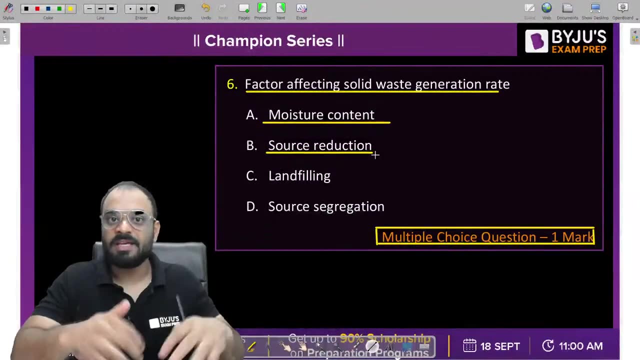 whatever moisture content is there in the solid waste, it doesn't matter and it will not affect the solid waste generation rate. but if we talk about, guys, the source reduction, what is source reduction? the place where the solid waste is generated, we are trying to reduce it by making 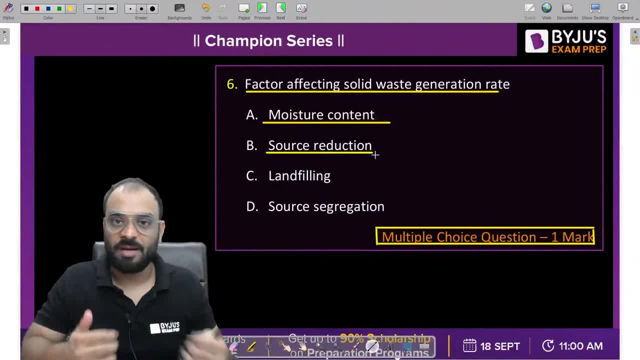 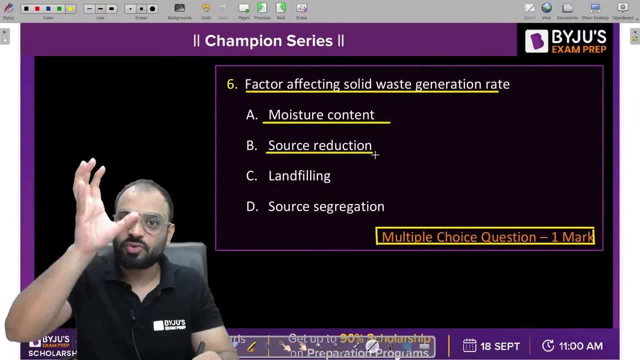 some changes, right? let us suppose, guys, if i make some habit, so like if i don't waste some paper or if i don't use the polythene, that means it is a source reduction, right? so the source where the solid waste can be generated, at that particular source we are 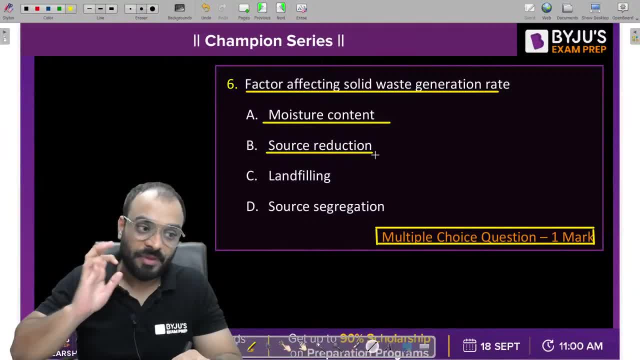 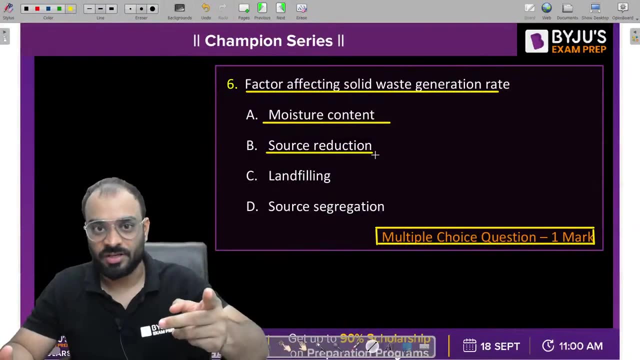 trying to reduce the concern, reduce the application of it. so you know that, guys, government of india and some other state government has also applied this particular condition. we don't have to use the polythene. yes or no. that means it is the type of source reduction if we are trying to reduce the 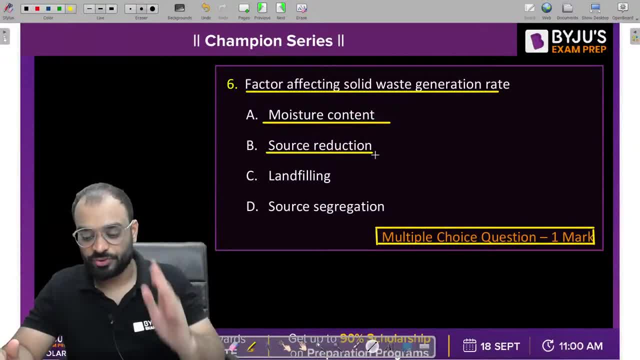 source, then ultimately the solid waste generation will also get reduced, yes or no. so that's why b is the correct answer for the problem. but if we talk about landfill, it is the process to treat the solid waste right. source segregation. that means you are trying to accumulate more and more amount. 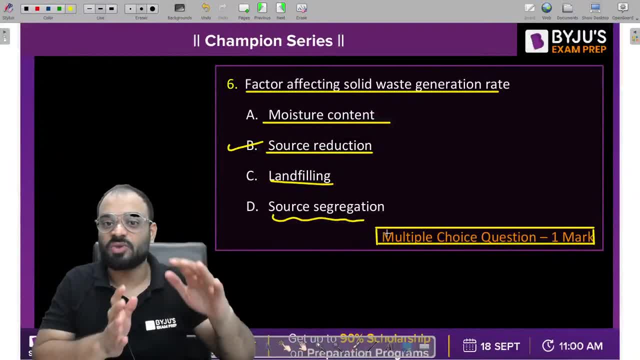 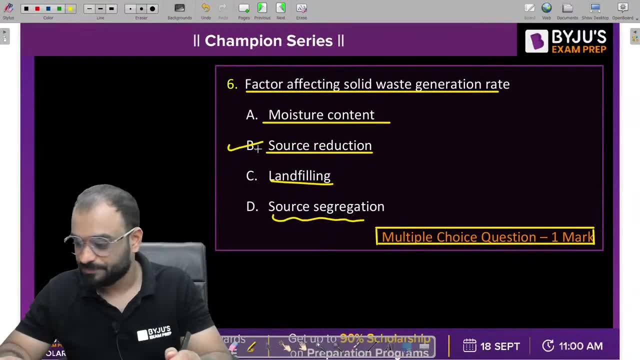 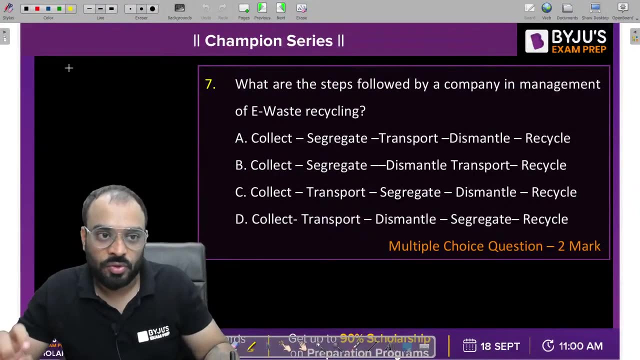 of solid waste. so that is nothing that will not affect the solid waste generation rate. basically it will increase, right? so that's why b is the correct answer for the problem. b is the answer for the problem. guys. let me tell you one thing over here again tomorrow. we are having again class tomorrow at 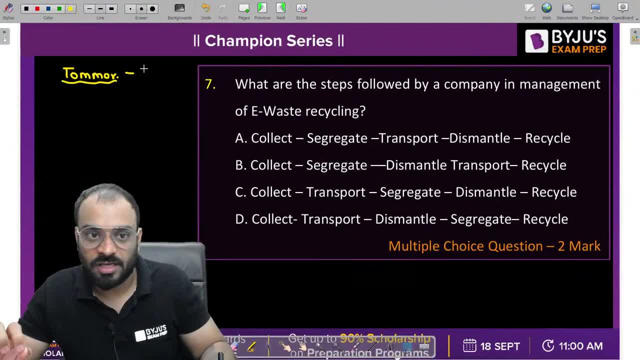 the same timing right tomorrow we are having the class for air pollution. air pollution- another important topic for your examination, and i will cover all the main part of the air pollution by the question right, so you can practice this particular session. also, guys, on our by juice exam prep youtube channel at 5 pm. so tomorrow again. 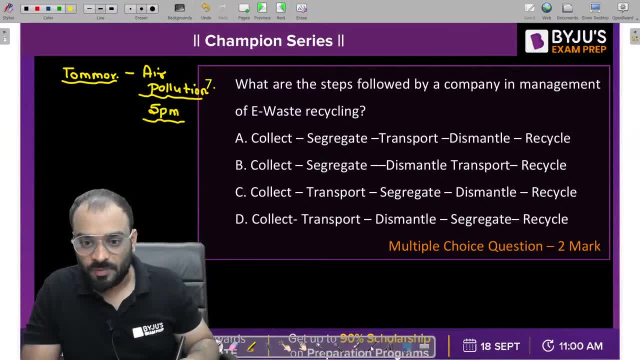 the same timing will be okay. next question, guys, please read it very carefully and this is mcq type question, but it is a two mark problem, not a one mark problem. two mark problem because it is. it is little bit logical, okay. what are the steps followed by a company in the management of e-waste recycling? 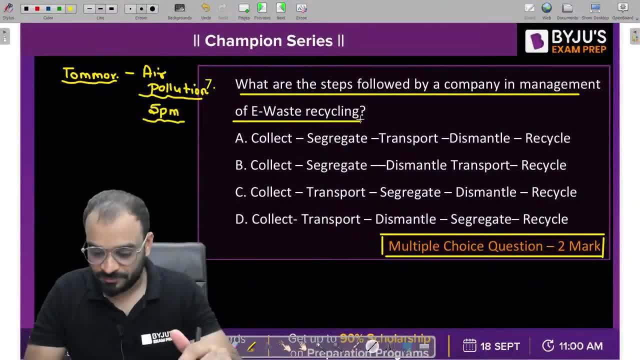 e-waste recycling. we need to recycle it. shakar c, shakar c. okay, what about other students? what do you say, guys? what are the various steps which you have to follow to manage the e-waste recycling through? c? very nice, a gajendra, a shian's a. 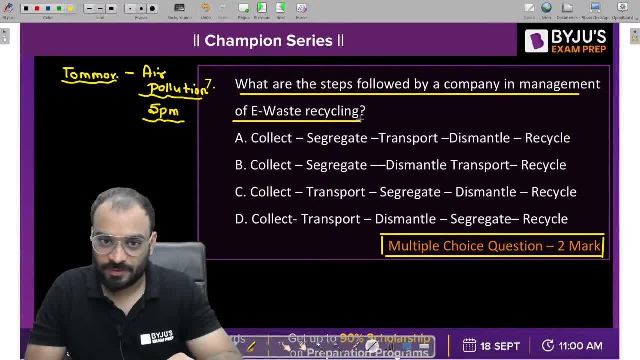 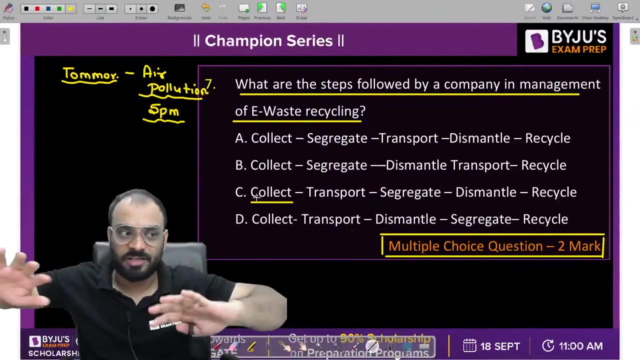 you guys. it is very simple to understand. let me explain first what is the process we need to collect. it is understood to all of you, right after collecting, how it is possible to segregate it. segregate means to separate the e-waste right like plastic material is different or like your iron. 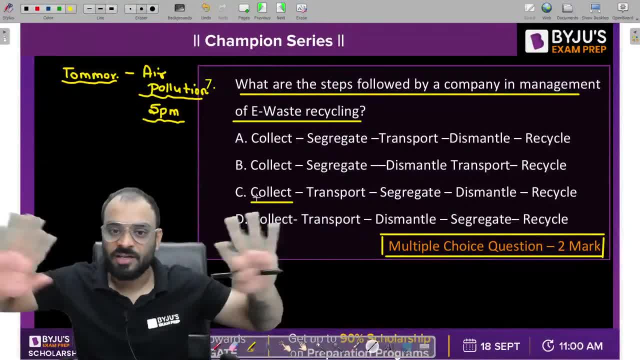 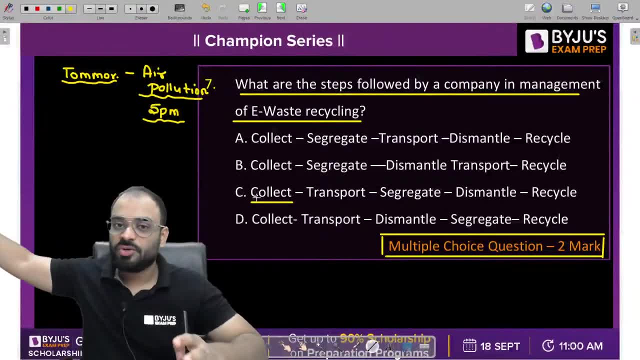 material is different, some other metal you are having, like copper and etc. so, guys, it is very difficult to segregate. so, guys, how you can segregate in initial stage it is not possible. if you are collecting it, you need to transport it to some place where we can do the segregation part. 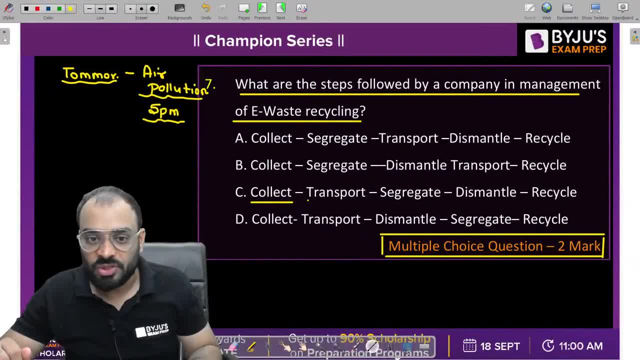 so that is why, guys, you need to understand: after collection, you need to transport it to some place where you can do the segregation, where you can do the segregation. now, after segregating it, guys, whatever part is there, remaining portion is there, you can dismantle it and ultimately, the portion 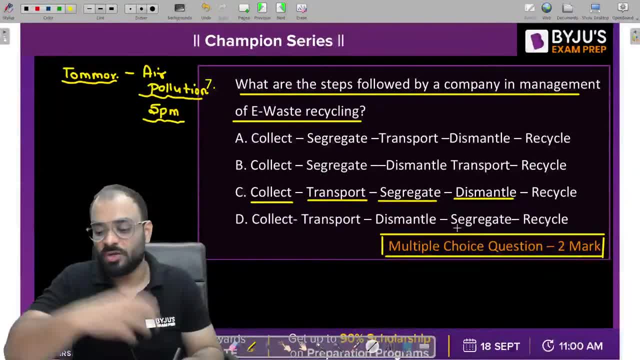 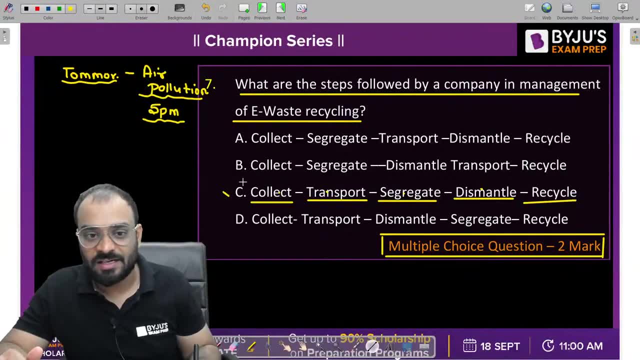 which is which can be useful for your recycling process is when you are collecting it. you are, you can do it right. so that's why, guys, collection, transport segregation, dismantle and recycle. that's why c is the correct answer for the problem. c is the correct answer for the problem. clear, very nice. 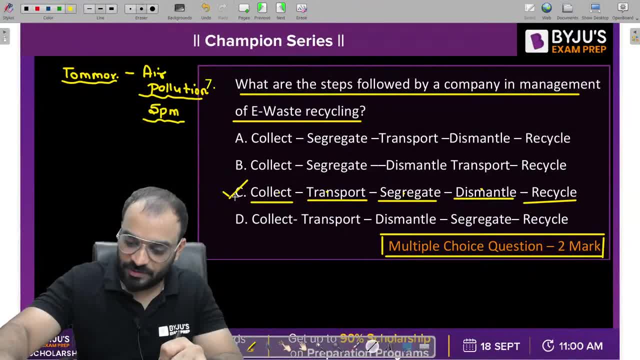 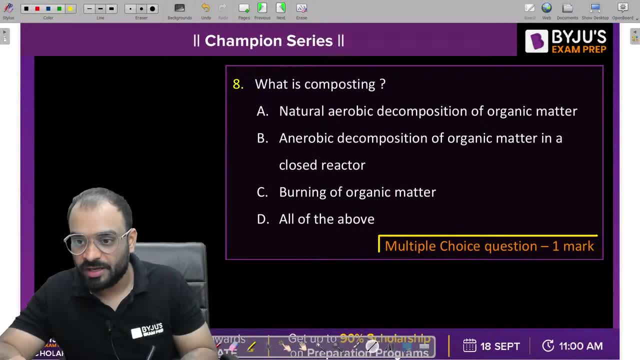 very nice. next question in front of you: what is composting? what do you mean by composting process? that is the question. what do you mean by composting process? quickly, let me know the answer, guys. what do you mean by composting process? a okay, dinesh, all of the above? no, we are very nice. 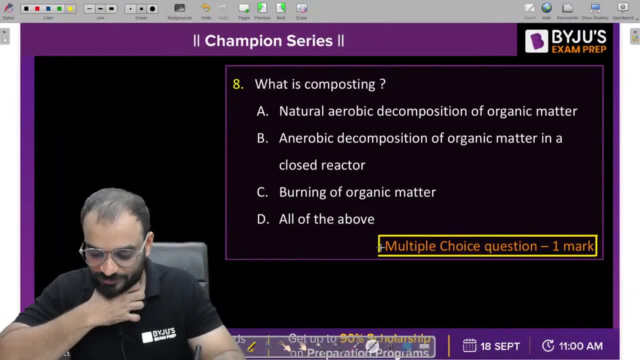 dinesh, please check your answer. composting is the process which is basically a biological process. composting is a biological process, right. it is a biological process in which we are trying to use the aerobic decomposition of organic matter. right, and that particular aerobic process should be. 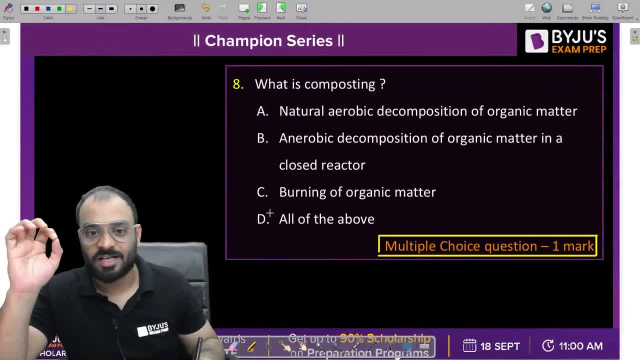 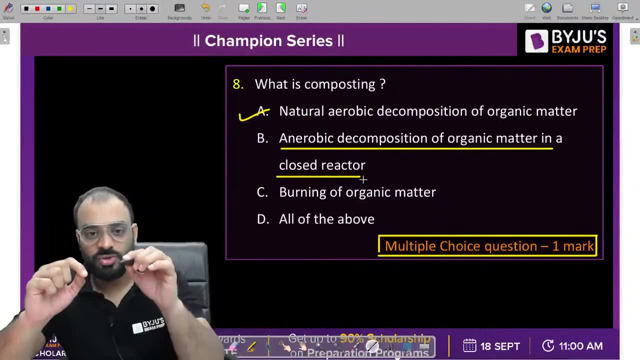 a natural one, right? so that's why, guys, a is the correct answer for the problem. a is the correct answer. but if we talk about anaerobic decomposition of organic matter in a closed reactor, that is not a natural one, right? and we are not doing in a natural way, right? so such type of process is not. 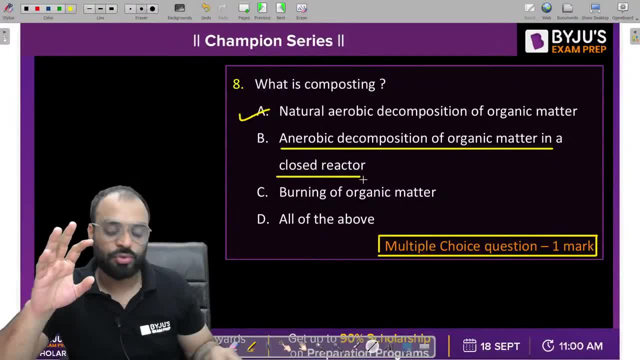 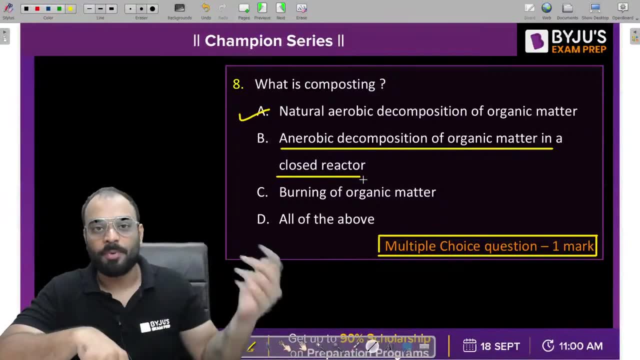 to be called as a composting. but guys, listen carefully. if you want to do the composting by anaerobic condition, you can do it. right, that is known as anaerobic composting also. but that anaerobic composting should be done into the some pit or some. you can say that, guys, a pit is to be. 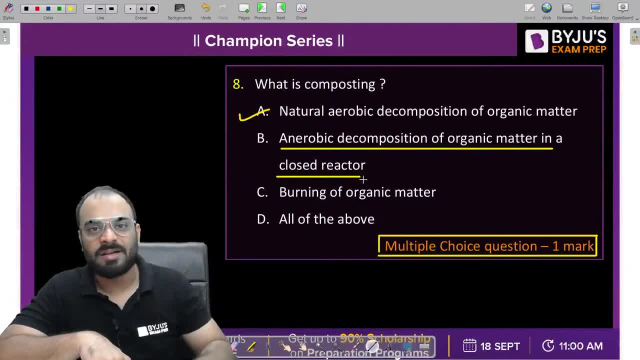 there in which you need to put the organic matter as well as night soil and mix it and ultimately you have to cover it right. that is the process of anaerobic compost. so that's why a is the correct answer for the question. a is the correct answer because we are able to choose any of the above. 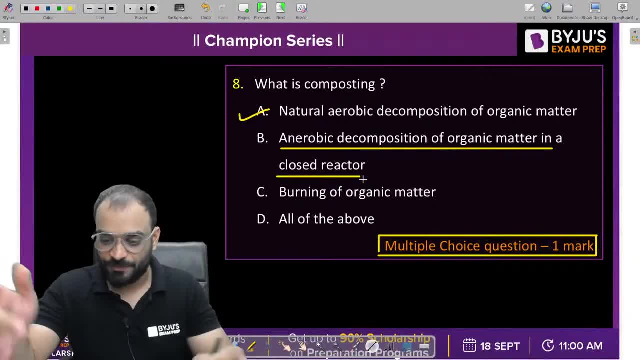 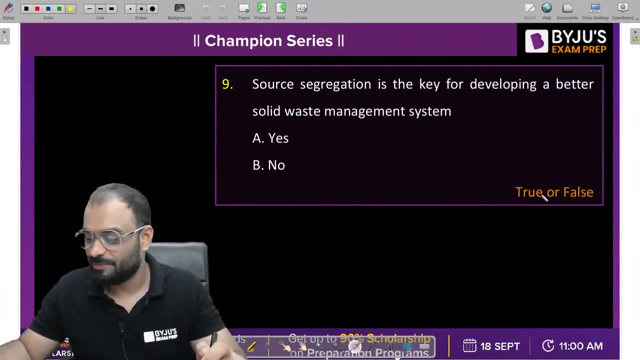 right. burning of organic matter is not possible. you know that now, guys, this question is basically a true and false, just a change in the pattern of question. I'm trying to put a such type of question also in my session. please let me know, guys, whether it is. 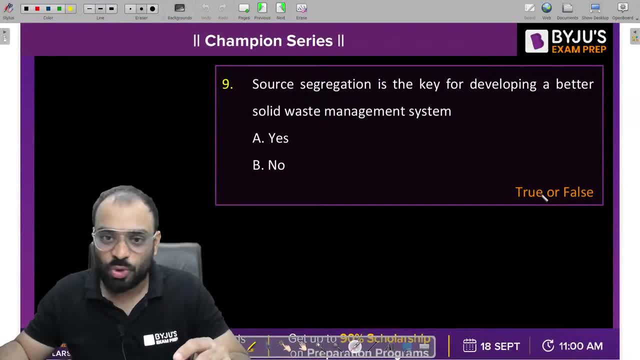 true or false? that is the problem. source segregation is the key for developing a better, solid waste management system. very nice statement. please let me know, guys, whether this statement is true or false at the source. if you try to segregate- segregate means separate the waste- then it will give us a better, solid waste management system, or not. 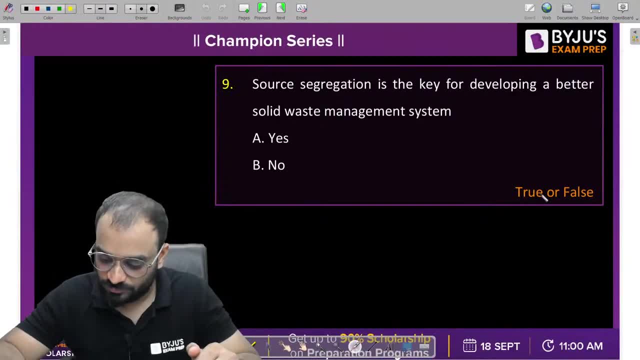 yes, yes, so it is true, 100 true. that's why government of india is also implementing such type of condition that you have to separate the dry waste and the west weight, wet weight, separately, right? so that's why, guys, that is nothing, as that is basically on. 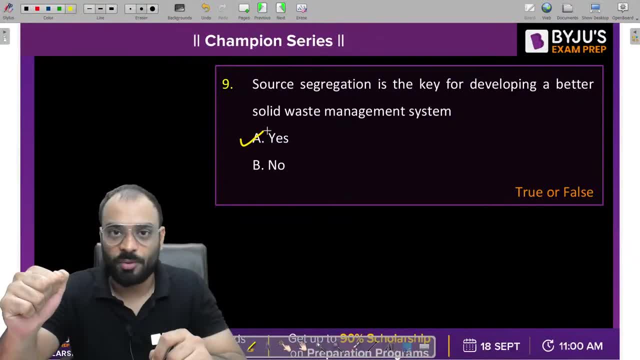 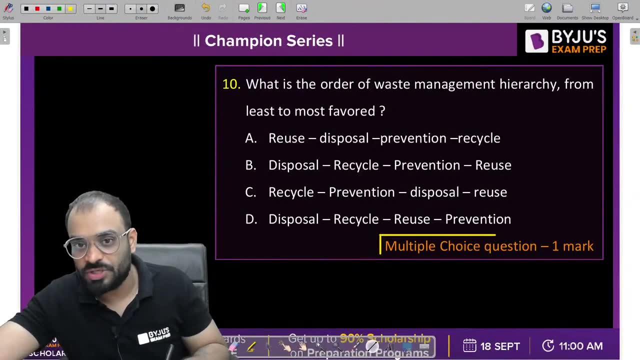 source segregation only. so a is the correct answer for the problem. next question, which is mcq type question: guys, one more question again in front of you: what is the order? what is the order of waste management? hirachi, from the least to most favored system? very, 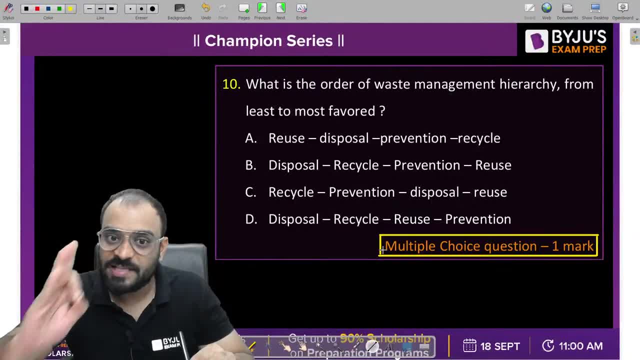 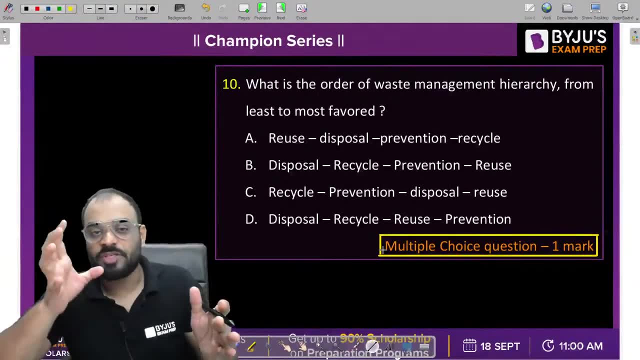 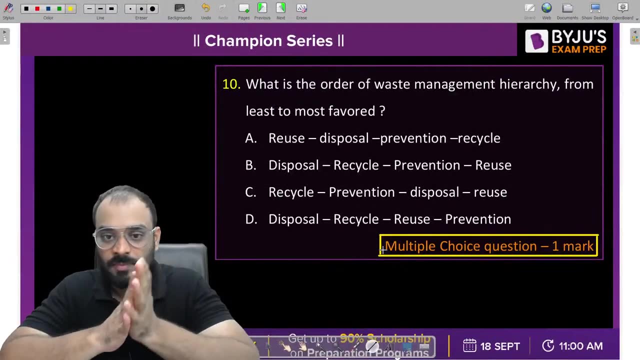 good question, guys, very good question: least to most favored right. you need to tell me, guys, which particular option you will prefer least and which particular option you will prefer more. d shian's d very nice. shian's any other student? d dinesh d very nice. 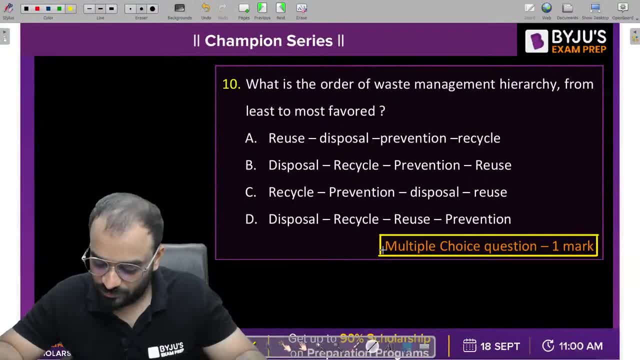 t, komal d. very nice. visheswar d, guru b. okay, now let's understand, guys. we need to mark a hirachi which is least to most favored option. you know that, guys. the first option which we will prefer in our solid waste management is prevention. right, we don't want to generate more. 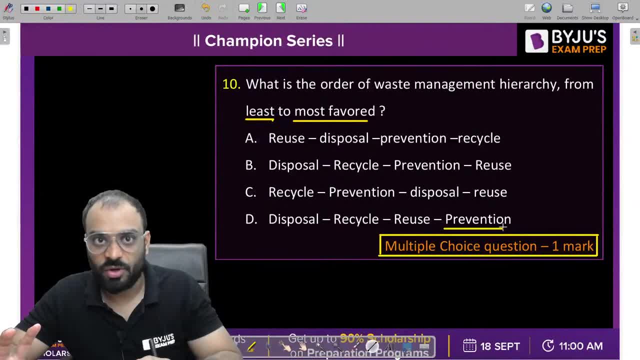 amount of solid waste. that's why you need to prevent it or reduce the concentration or reduce the generation of solid waste by prevention, right, that's why this is the most preferred. then, if it is generated, then prefer reuse concept. let us suppose at the source itself i have generated some amount. let us suppose this is my solid waste right now. okay, just consider. 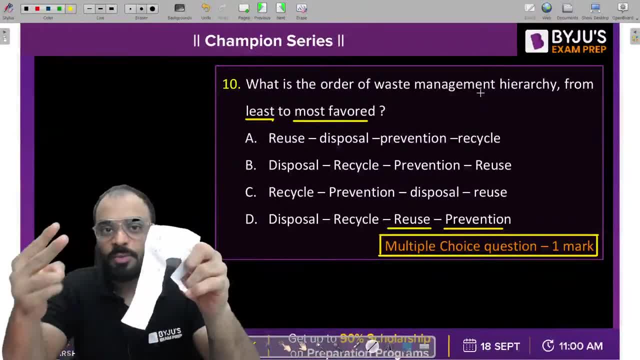 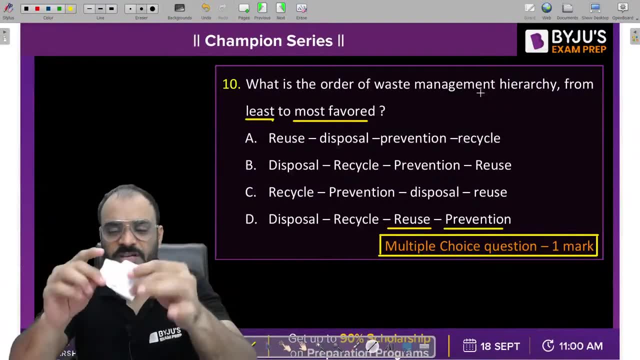 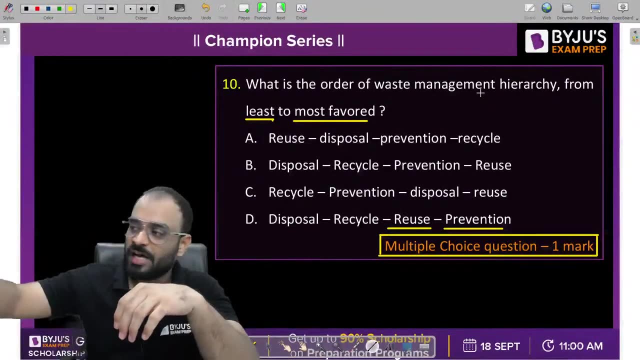 this is the solid waste which is generated right now. so the second option is reuse it. i have to reuse this particular paper by any way, if it is possible, so that is called reuse. if it is not reuse, then recycle it. you have to throw it and ultimately some industry will purchase such type. 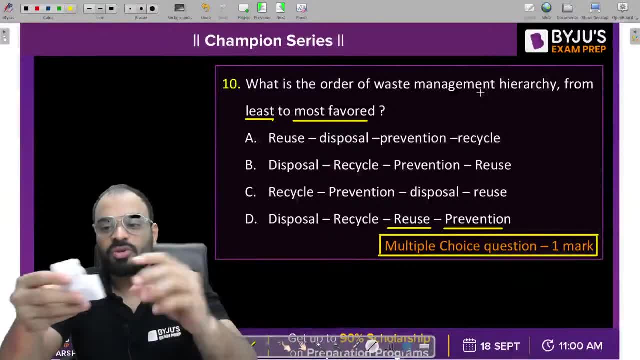 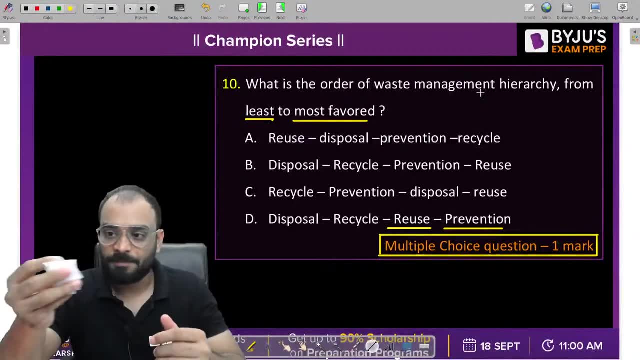 of waste and ultimately they are trying to recycle it so that they can form this particular paper in other way. let us suppose they can make this particular paper into some copy and etc. right? so that's why, guys, this option will be recycled. then the last option, or the last. 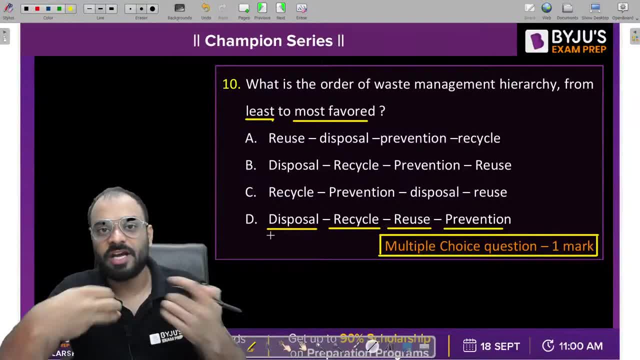 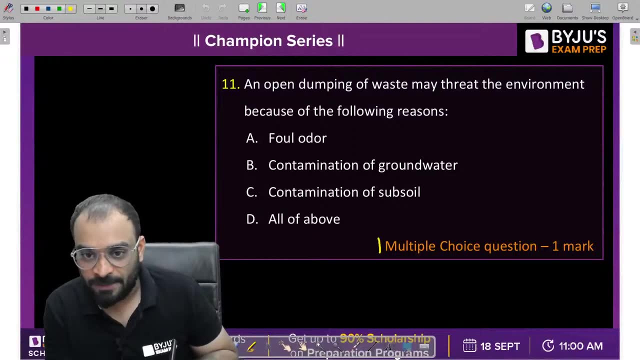 preference goes to the disposal right. if you don't have any kind of option, whether it is reuse or recycle, so we will go with the disposal process. so that is called least preferred. okay, t is the correct answer for the question. next question in front of you: mcq, mcq, mcq, one mark question. then we have the last one is msq, which is two mark, which you have. 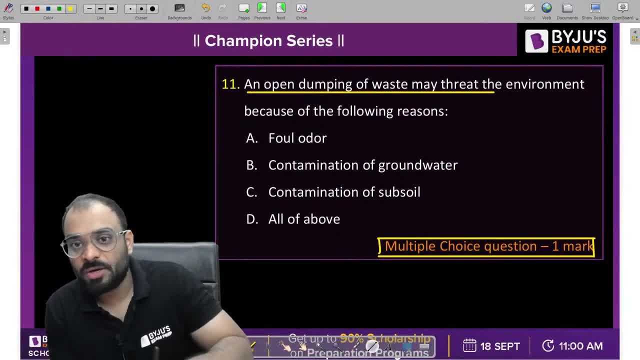 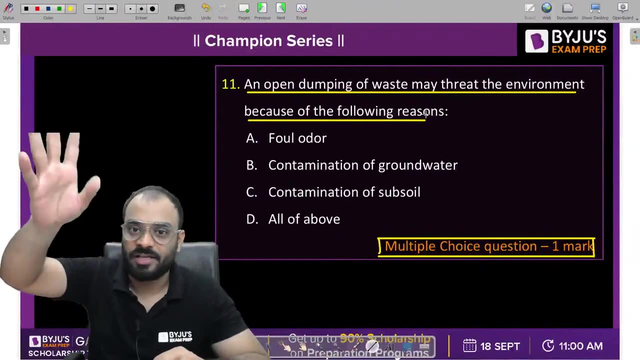 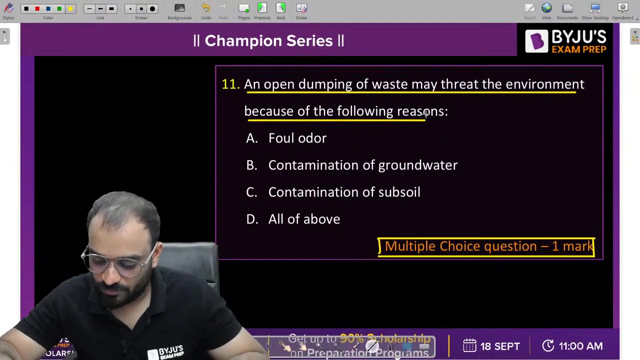 to solve in detail. an open dumping of waste may be treated the environment because of the following reason: open dumping. open dumping means just you have to take the waste and throw it in a open land area that is called open dumping gathering. you are set. the adopting is going to occur in some stream. all we are doing is 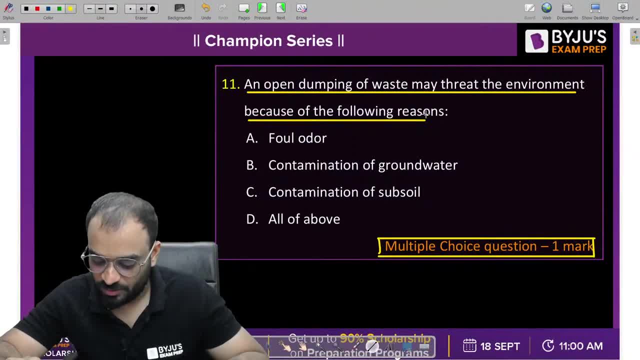 taking the secondchn of the Administrative Reservice, that is, the taking that out of our labor and talked that, which is taking all the material that is coming out of our food and common waste. the remaining, Julio, control on the three parts, bringing the on the three parts, collecting the organic waste and having 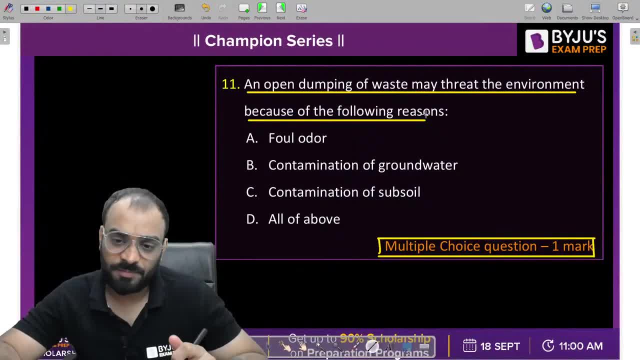 the surface of själ a and a a. so they have to take the full supply of the organic waste into the primary and the secondary system. To solve that you have to take the full supply of the organic waste. so it means WE have this triangle in the death line which I told last class in the last class in brazil b, and it will take. 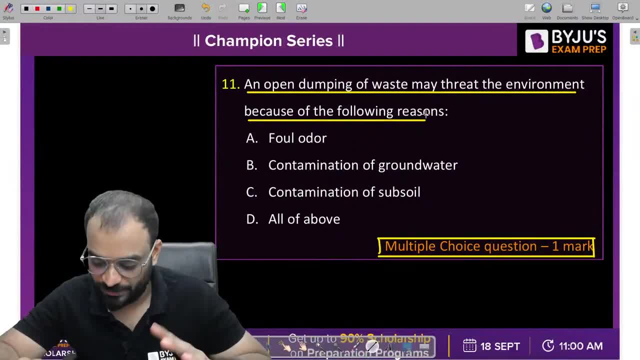 of course the other side: three four, three. so you need toращly Goldman Sachin, need to reach the mcq type question. you need to choose a single option only. okay, d. she answered d. now listen, guys. yes, it is d. d is the correct answer for the problem. now let me. 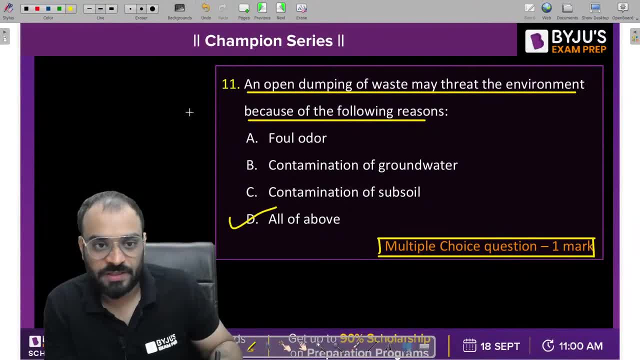 explain how it is possible. the first one is: let us suppose, guys, this is an open land area in which we have thrown some waste. now what will happen? it will produce some foul order or foul guesses. right, it will produce some foul guesses. by the degradation of it, you may have some foul guesses. 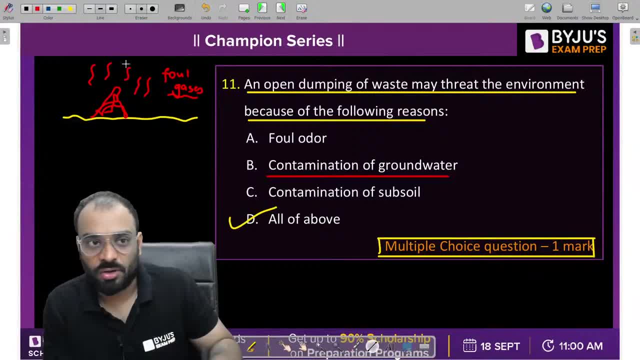 the second thing is it contaminate the groundwater also. what will happen, guys? let us suppose if some rainfall will occur, if some rainfall will occur and the liquid form of waste which is present in this particular solid waste may be get collected with the rainwater and that rainwater may go into 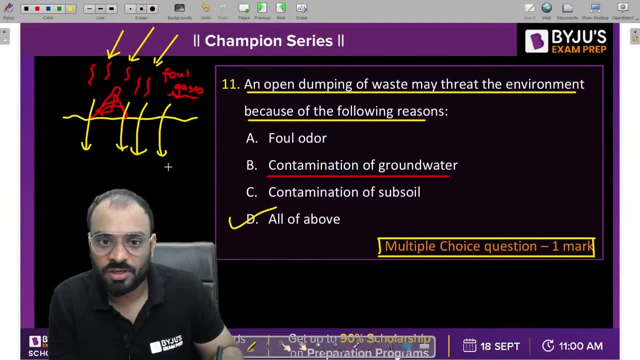 the groundwater also. so it may also cause some foul gases. right, it will produce some foul gases, contaminate the groundwater. that can also happen. so a is correct, B is correct. what about contamination of subsoil? yes, if this particular water which is contaminate, it is passing through the soil area. so definitely is also. 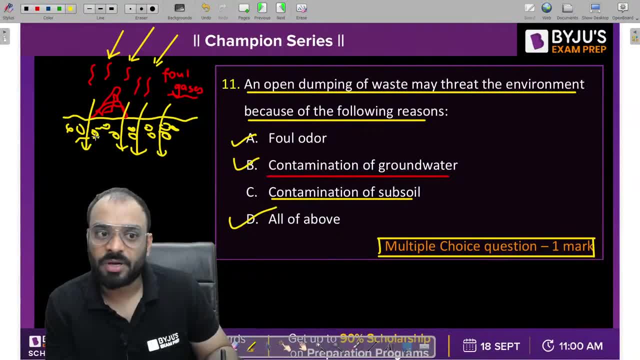 contaminating the subsoil also right, because it may be possible, guys. some of the impurity may get present or may get entrapped between the soil particle, so it may get contaminated, right. that's why C is also correct. so a, B, C is the correct answer. that means D is the correct answer for the problem. 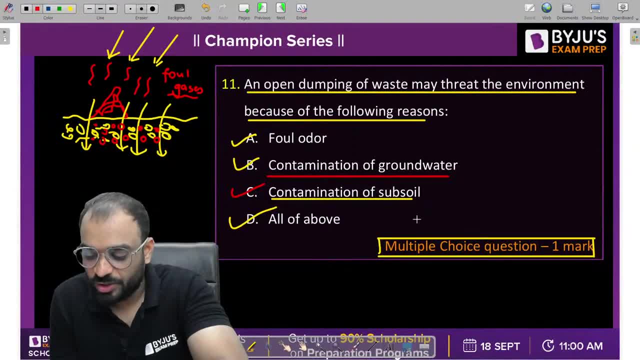 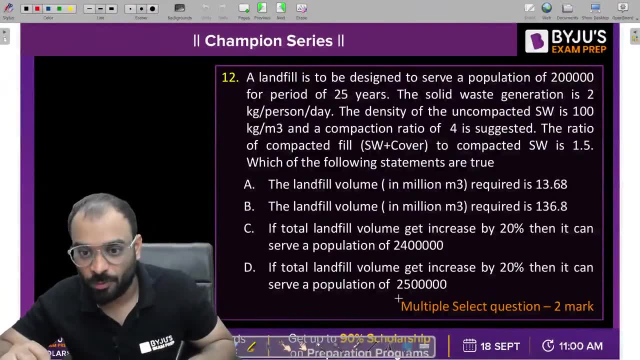 okay, now the last question in front of you for the of the session. let's understand the last question. this is MSQ type of problem. MSQ- be careful guys, it is two mark question: MSQ- what is given to us and what we have to find. let's read it in detail. 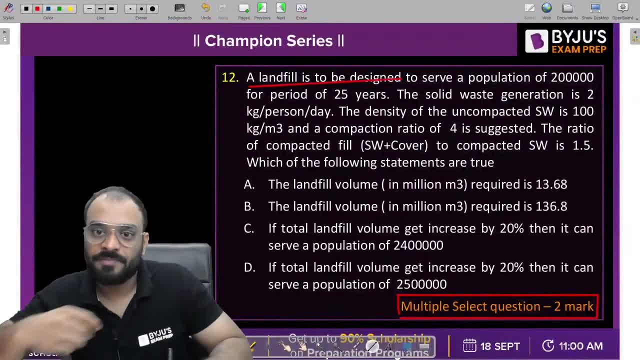 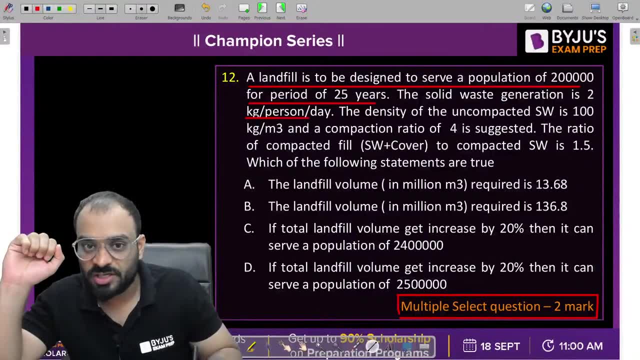 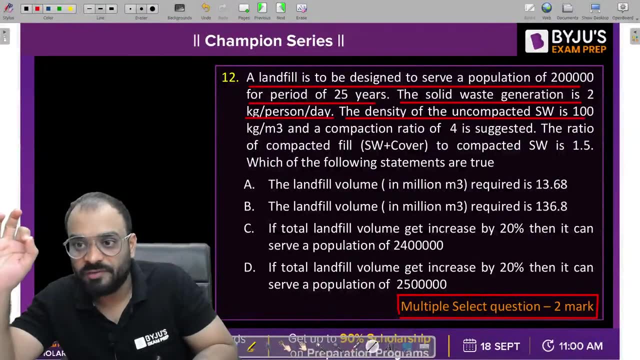 last question of the session. a landfill is to be designed to serve a population of 2 lakh for a period of 25 year. the solid waste generation rate is 2 kg per day per person. okay, the density of uncompacted solid waste is 100 kg per. 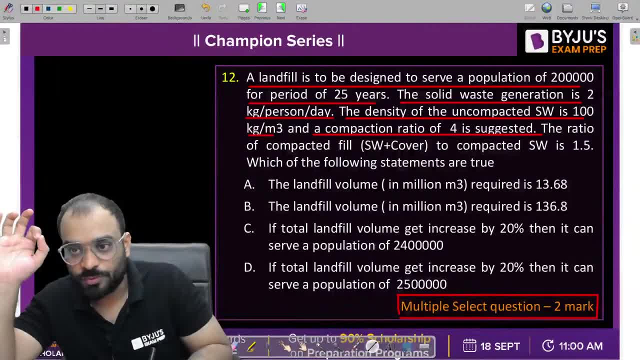 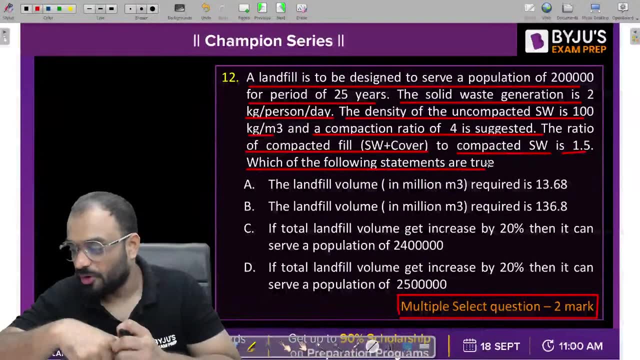 meter cube and the compaction ratio is 4. the ratio of compacted fill, which means solid waste plus cover, to the compacted solid waste is 1.5. now, which of the following statement are true? that is the question. which of the following statement are true? that is the question. 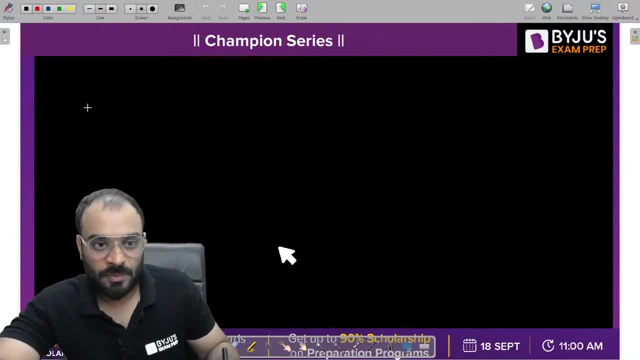 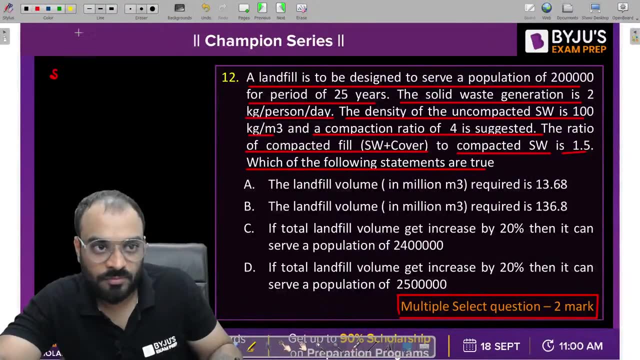 let's understand. so, guys, the first thing which we need to calculate is the solid waste generation. this solid waste which is generated is 25 all it raised and ratio, and 25 air and 25 we are. how much amount of solid waste will get done break? that is the first question. so we can write you, guys, it is the 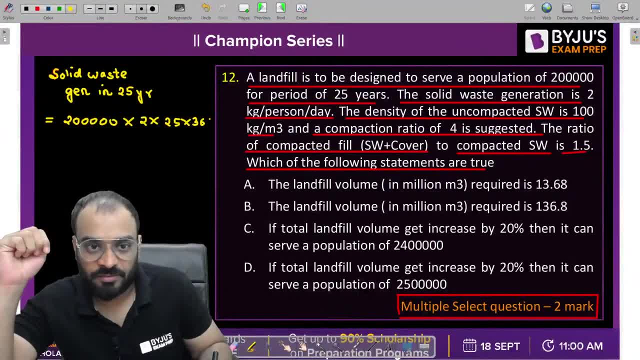 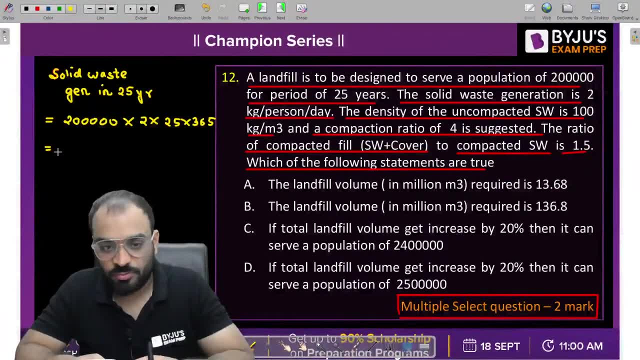 population is 2 lakh, then we have a rate of the solid regeneration. it is 2 kg per%. So 25 multiplied by 360.. You will get your answer in terms of kg. Tell me, guys, how much it is: 2 lakh multiplied by 2, multiplied by 25, multiplied by 360. 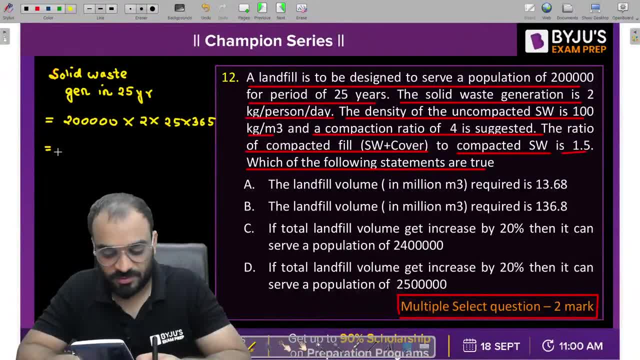 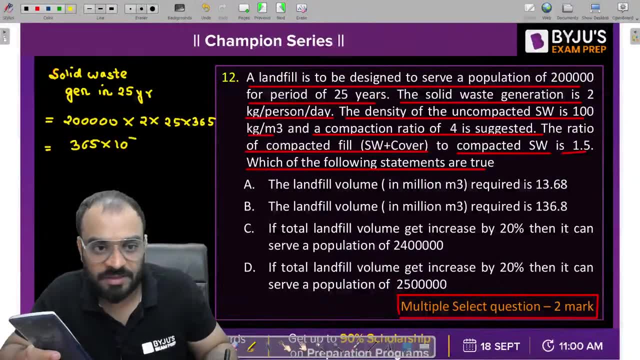 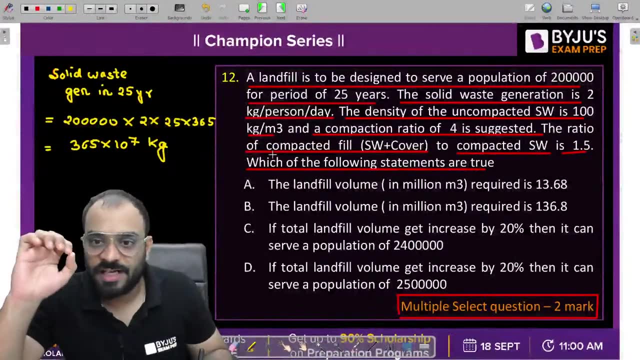 And divided by, let's suppose, 10 raised to power, So we are getting a value of 365 into 10 raised to power, 7 kg. So this is the amount of solid waste which will get generated. Okay, Now what is the density of uncompacted solid waste? 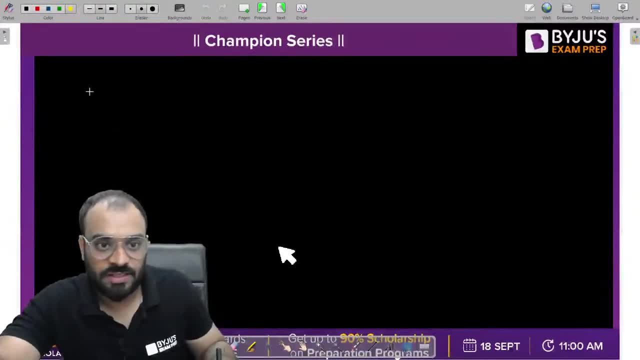 This particular solid waste is uncompacted right now. So can I say that, guys, Volume of uncompacted solid waste is equal to mass of solid waste, which is 365 into 10 raised to power 7.. Divided by density of the solid waste which is uncompacted, 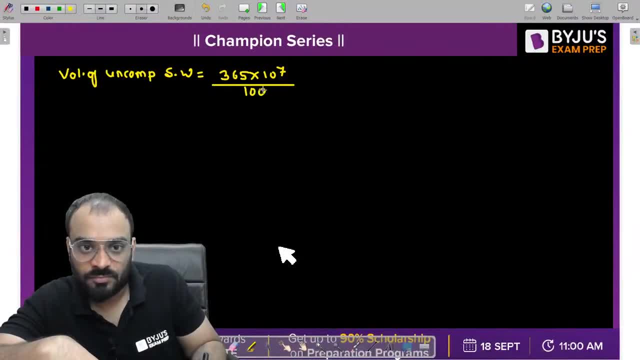 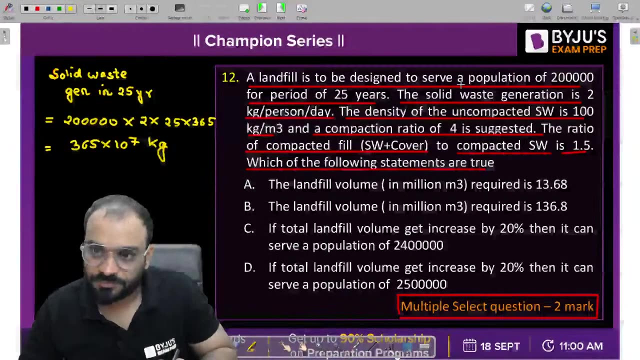 And the value is 100. If you put it, you will get 365 multiplied by 10, raised to power, 5 meter cube per day as a volume of uncompacted solid waste. Clear Now, guys, what they have written. You need to consider the compaction ratio as a 4.. 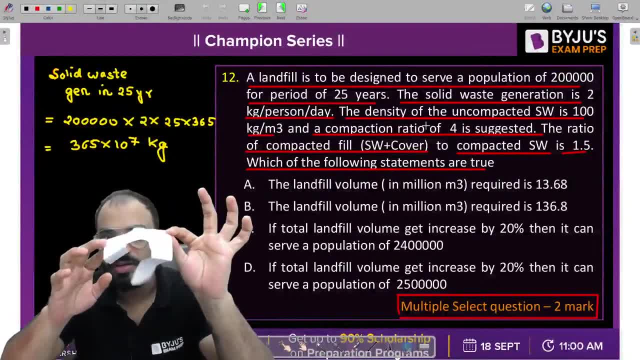 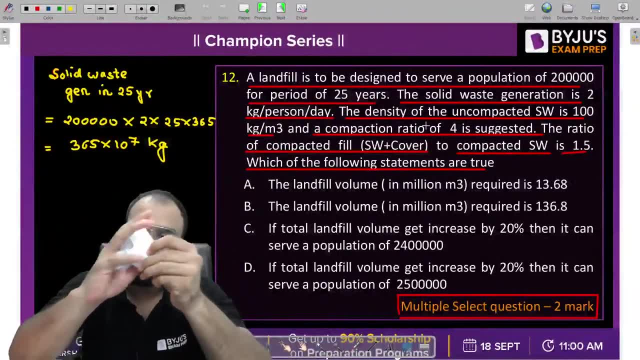 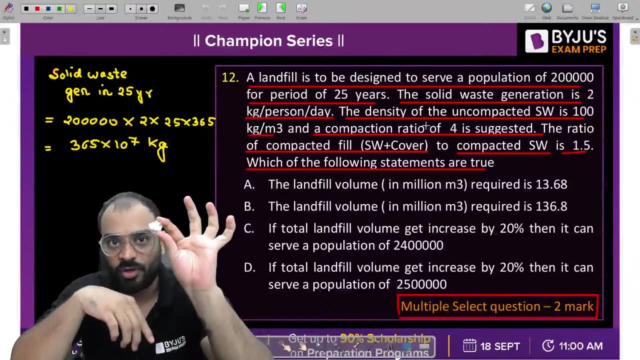 What is compaction ratio? basically, Let us suppose this is your solid waste which is uncompacted right now. You can see, guys, the volume of this solid waste is very high, Right, But if I Compact it Now, you can see here, guys, the same amount of solid waste is present in a small volume. 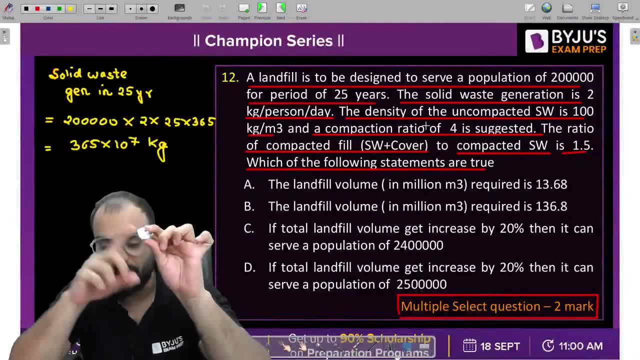 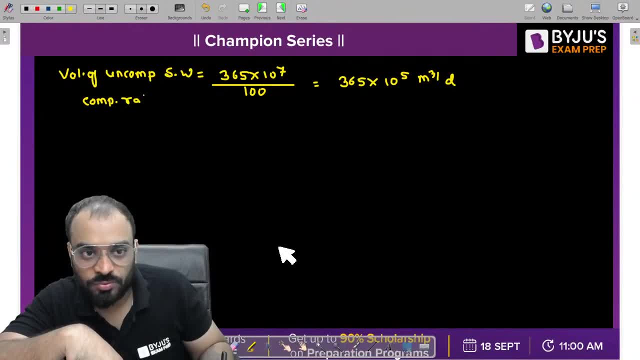 So this particular volume is known as what Compacted volume, Clear, So you can write here compaction ratio. Compaction ratio is nothing, as it is the volume of uncompacted divided by volume of compacted, So this value is given to us. 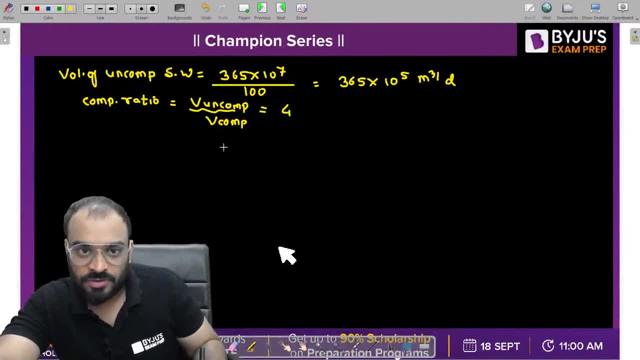 How much it is. It is 4.. So we can calculate the volume of compacted solid waste. also, It is uncompacted Divided by 4.. So this value is 365 multiplied by 10, raised to power, 5 divided by 4.. 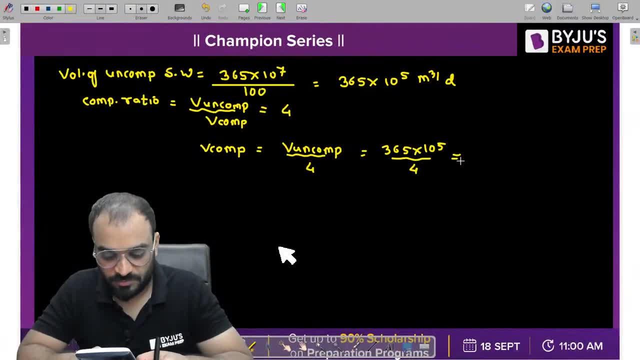 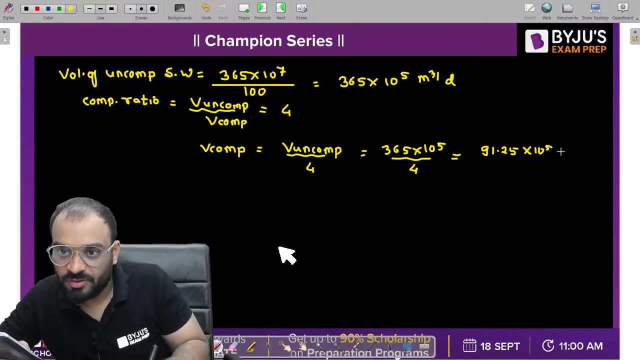 Let us calculate it How much it is. So we are getting a value of 91.25 into 10 raised to power 5. Meter cube. Ok, Do not write meter cube per day, It is meter cube Clear. 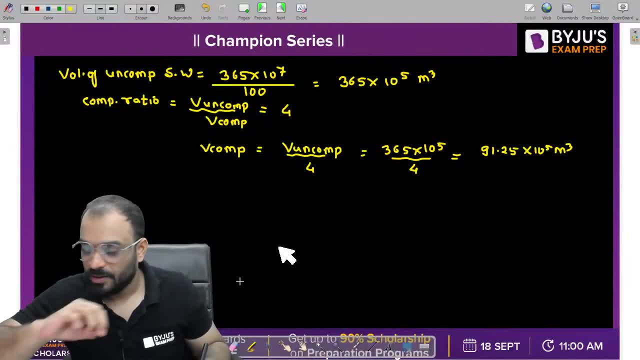 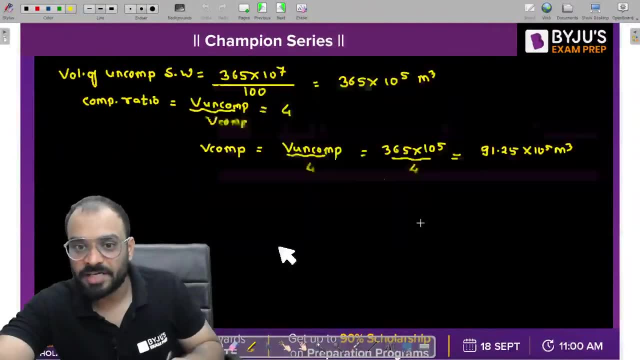 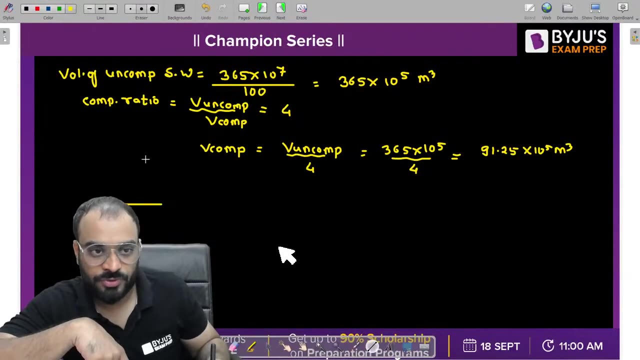 Meter cube Clear. Ok, Now, guys, let us understand the remaining thing: The ratio of compacted film plus compacted solid waste. Now you know that, guys, there are two things basically in your solid waste. Let us suppose. Let us suppose. 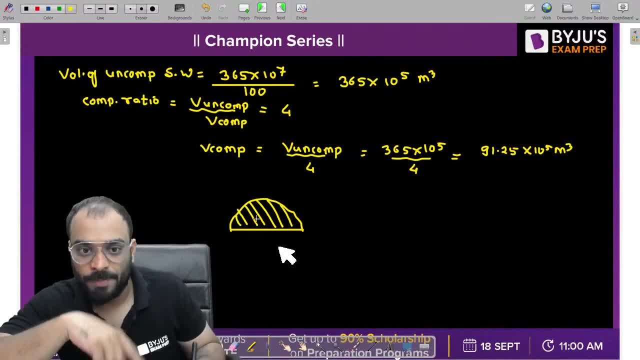 This is the solid waste room right, which is basically compacted solid way. this one is volume of compacted solid waste. now let us suppose, guys, if I am having the volume of compacted solid waste and along with it, I am having the cover also here. so this is basically cover. 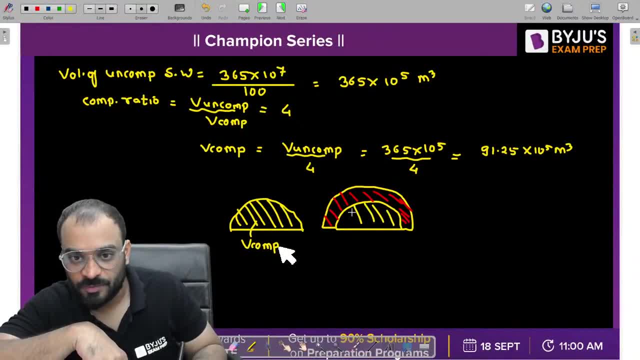 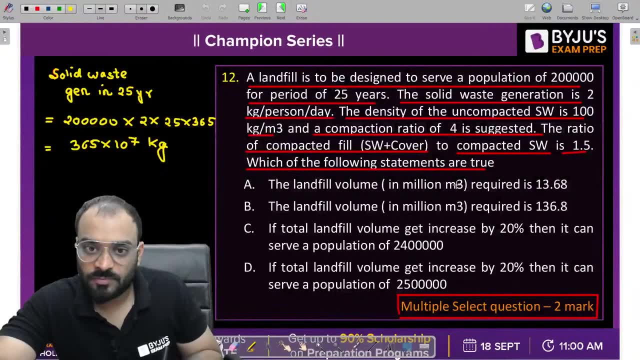 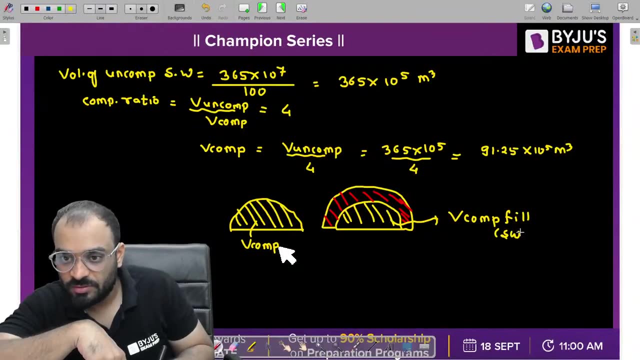 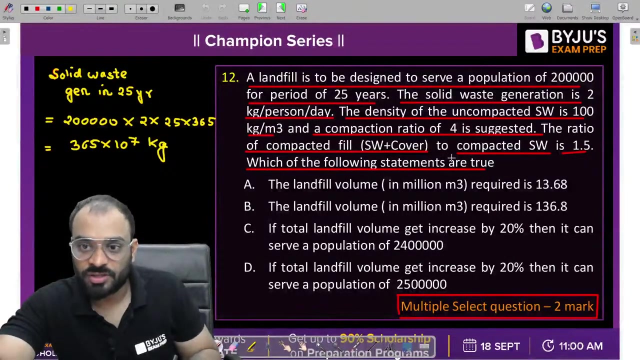 this is cover and this is our solid waste. so can I say that this total volume is nothing as volume of compacted fill will means what it is: solid waste plus cover. and this value is written over here. how much it is, it is a. okay, they have given the ratio I need to. 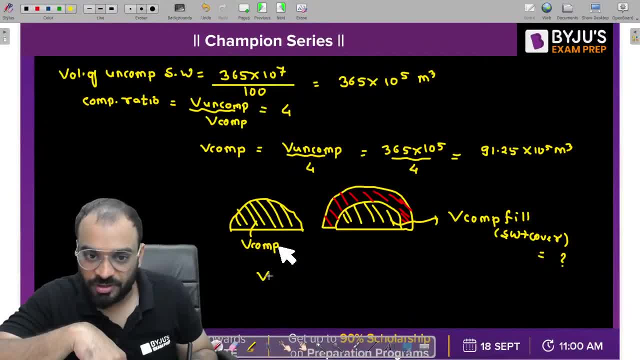 find out this value first. okay, so what is the ratio of it? compacted film divided by volume of compacted, this value is equal to 1.5. now you need to put this particular value how much it is. it is 91.25 x 10 raised to power 5, please. 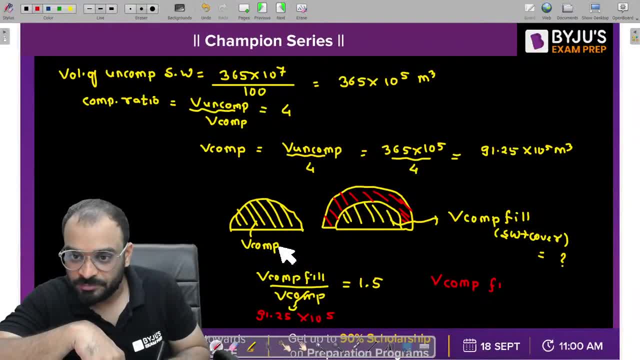 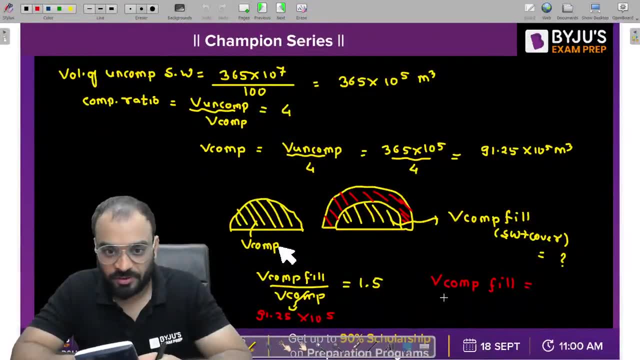 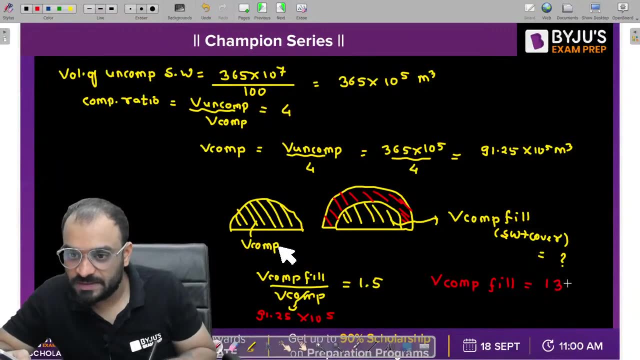 calculate what is the volume of compacted film, how much you are getting volume of compacted film. so we are getting a value of 1, 3, 6, 8, 7, 5, double 0 meter cube. or you can write it: 13.68 x 10, rest to power: 6 meter cube. here guys, kindly check it. which one is the correct? 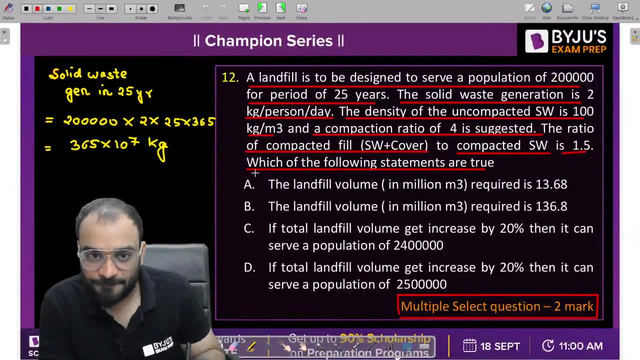 answer a or B pants. a is the correct answer. the landfill volume should be acquired is equal to 13.68 clear. So B option is wrong, It is not 136.8.. Now, guys, if the total landfill volume get increased by 20%, 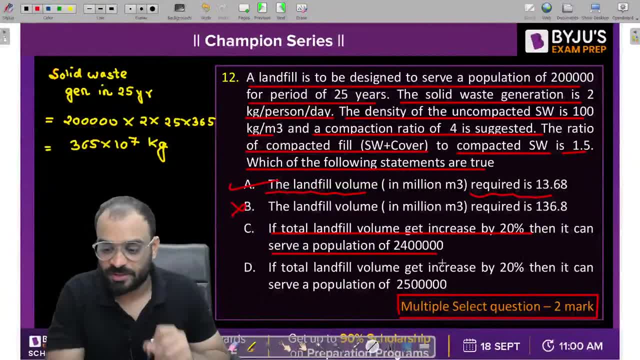 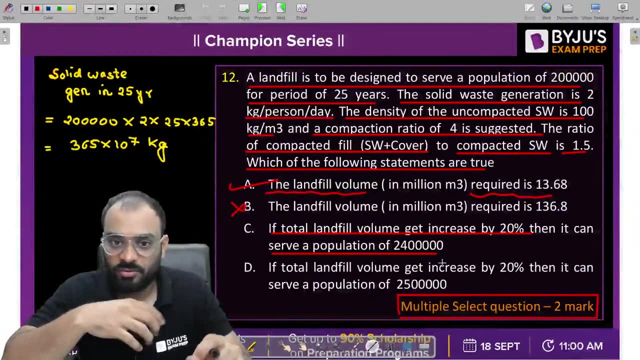 then it can serve a population of this much. We need to check it. We need to check it. If we increase this particular volume, if we increase this particular volume by how much- 20%- Then for how many people, or for how many people that particular landfill can serve? 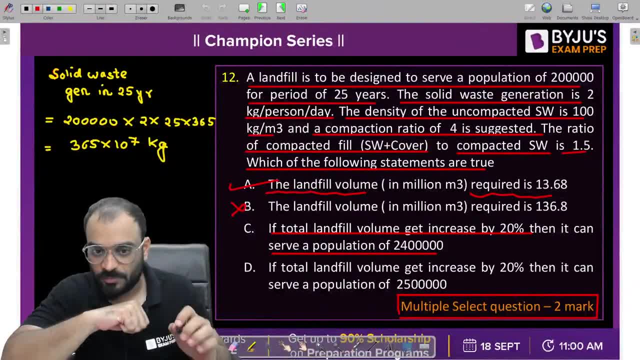 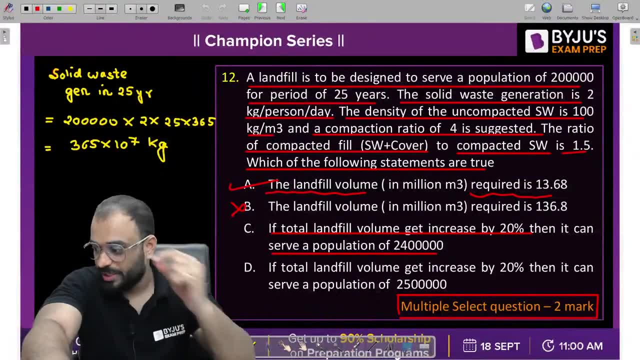 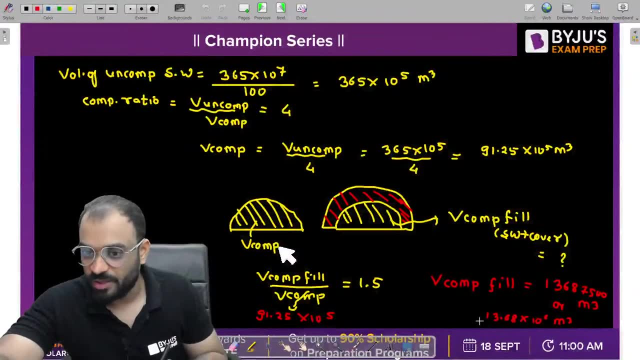 That is the question, Clear, Okay. So first of all, what we can do over here, guys, We need to calculate the volume. Okay, Let us suppose right now you are having a volume of 13.6875 into 10 to the power 6.. 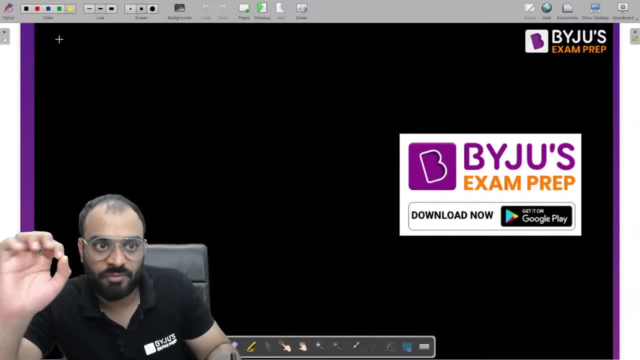 Okay, So what we can do, guys. First, I will increase the volume by 20%. Volume of compacted fill should be increased by 20%. That means we need to write 1.2 times, 1.2 times of what 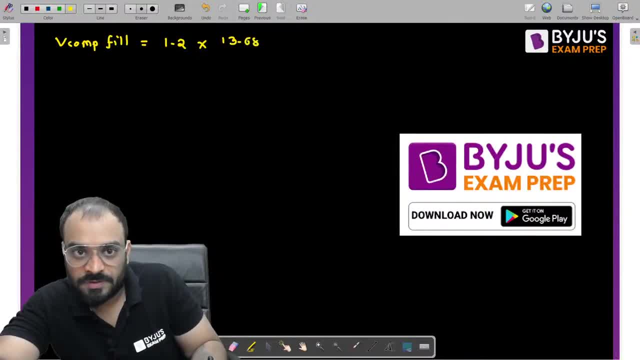 The volume which we are getting, which is 13.6875 multiplied by 10 to the power 6.. Please calculate this volume first. So we are getting a value. So we are getting a value of 16.425 into 10 to the power 6 meter cube. 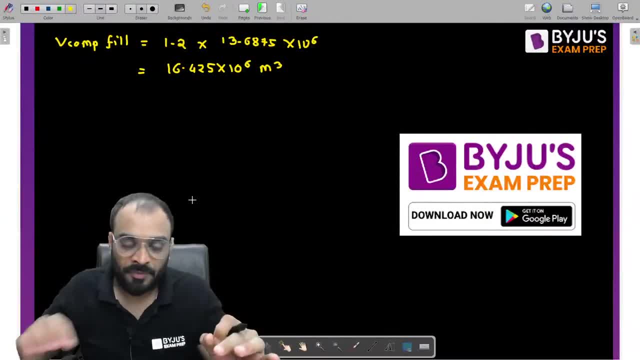 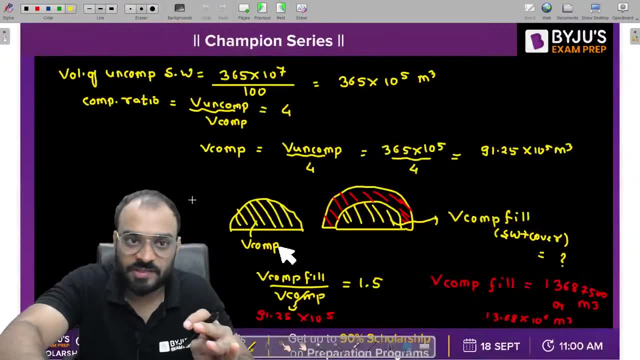 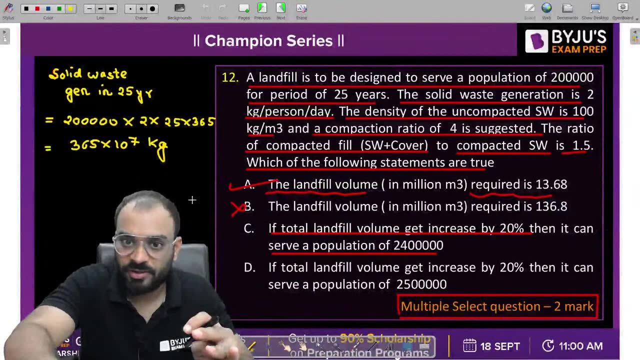 Clear Now, guys. the question is the solid waste. how much solid waste is there? Right, We need to calculate. how much solid waste is there Uncompacted, Compacted? Okay, We need to calculate what is the volume of compacted solid waste. 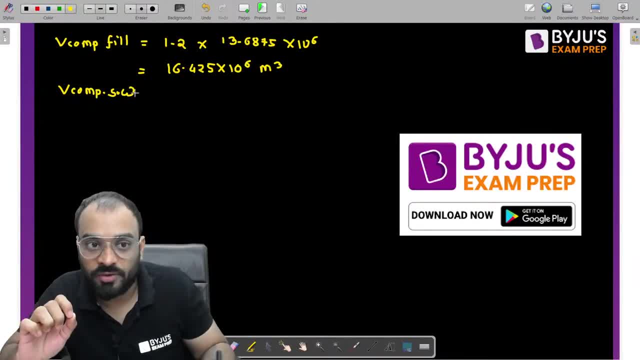 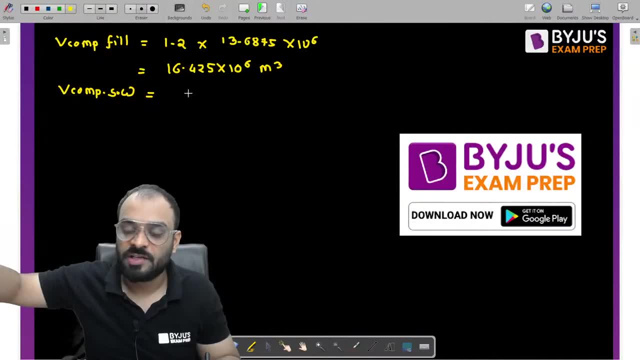 Not fill, It should be compacted solid waste. So we can write here, guys, the volume of compacted fill upon volume of compacted solid waste. This ratio is already given to us, which is equal to 1.5.. So can I write here? 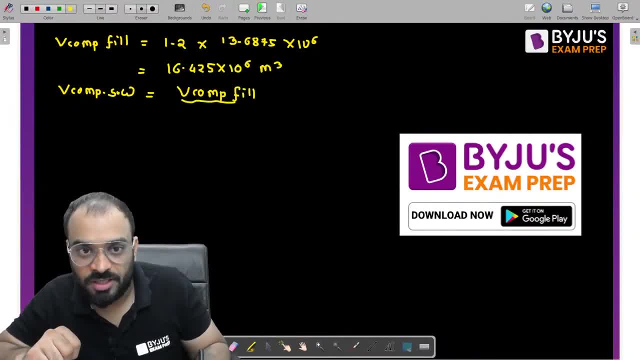 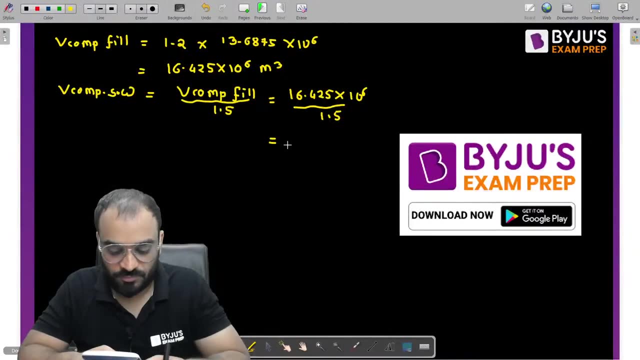 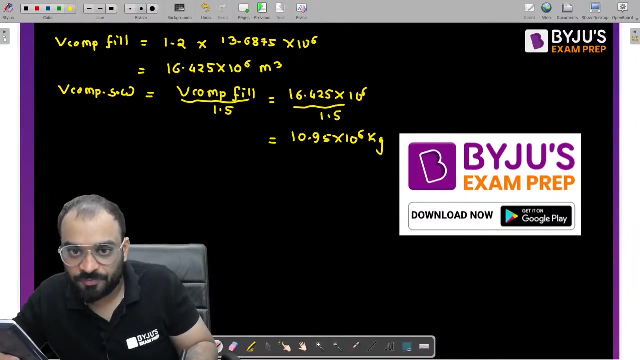 Volume of compacted fill divided by 1.5 will get the volume of solid waste which is compacted. Please calculate this. We are getting a value of 10.95 into 10 to the power 6. Kg. Okay, Are you getting it? 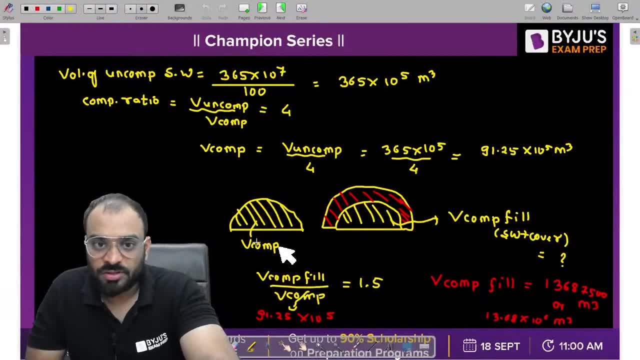 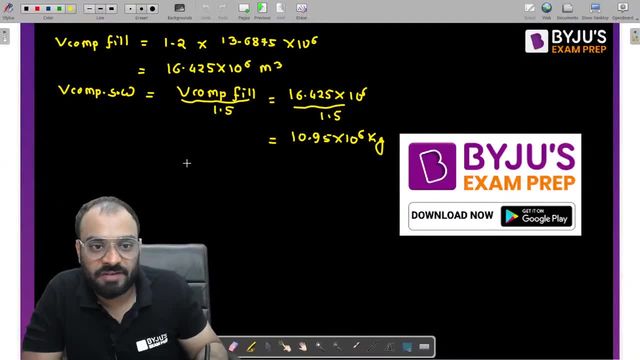 Okay, Now, guys, again you need to find out the volume of uncompacted solid waste. Volume of uncompacted solid waste. So do you remember, guys? They have given the ratio of compacted solid waste Right, Right, Right. 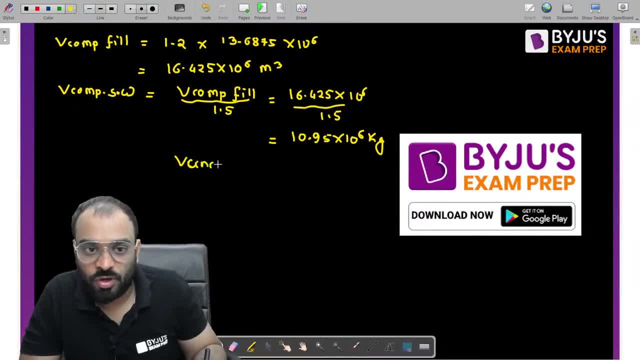 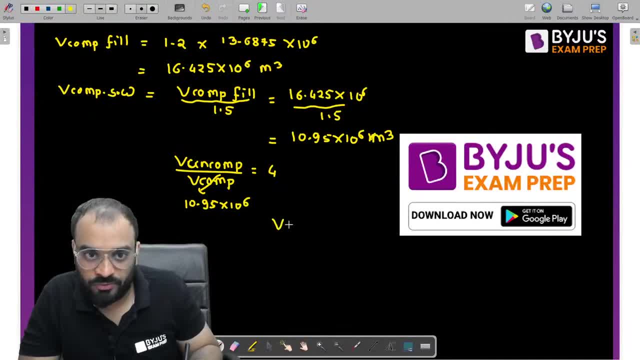 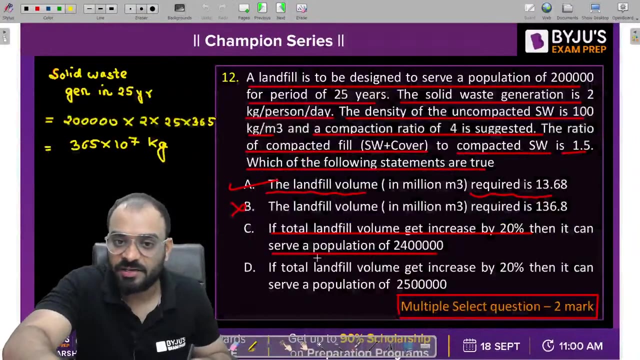 meter cube as a volume, the volume of uncompacted is equal to 4 times this value. so we are getting a value of 43.8 into 10 to the power 6 meter cube, correct, okay, now can we calculate, guys, how much mass of solid waste it can generate? how we can do it? we know the 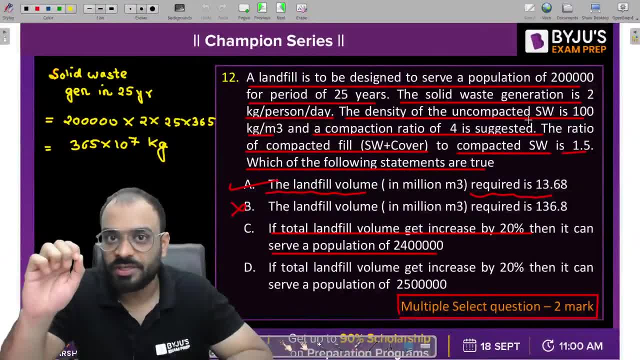 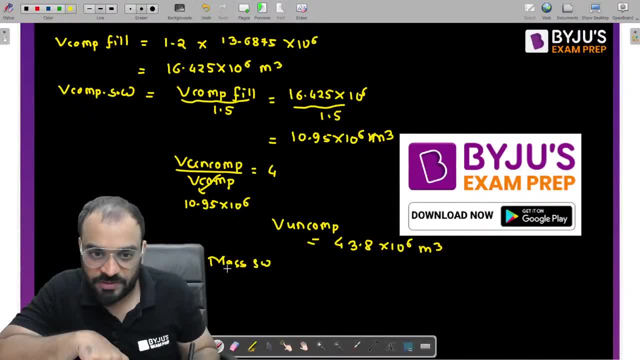 density of uncompacted is equal to 4 times this value. so we are getting a value of 43.8 compacted solid waste. can we calculate the mass? yes, we can do it. so mass of solid waste divided by a volume of uncompacted solid waste is equal to density of uncompacted. this value is already. 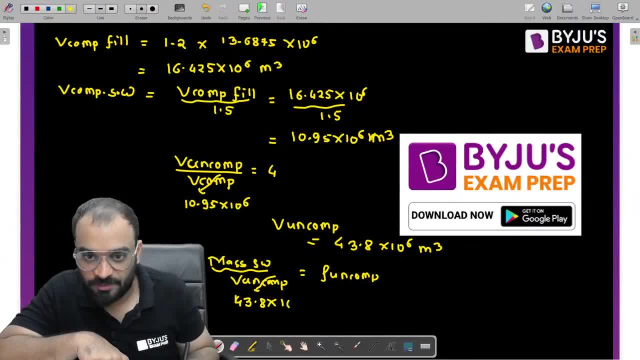 known to us: 43.8 into 10 to the power 6. this value is already known to us, which is 100 here 100. so can we calculate the mass of uncompacted solid waste. can we calculate the mass of uncompacted solid waste? also, mass of solid waste which is equal to how much you can write here, 43.8 into 10 to the power. 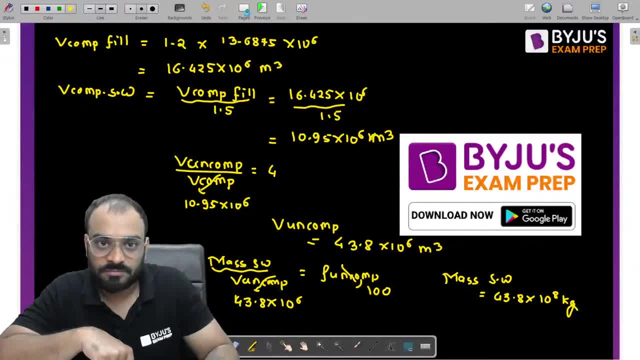 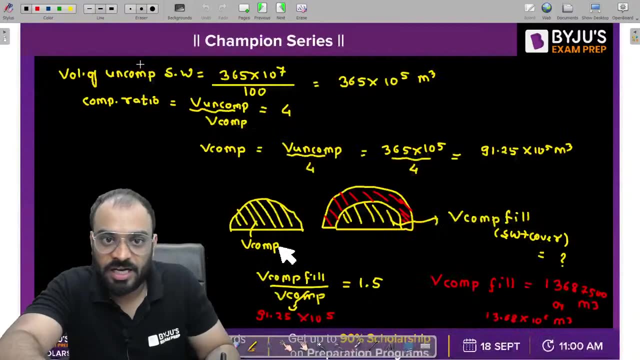 8 kg. okay, okay, sir. now, guys, the last step which we have to do. this value is known to us: 43.8 into 10, to the power: 8 kg. can i say that, guys? let us suppose the population is p, the rate of generation. 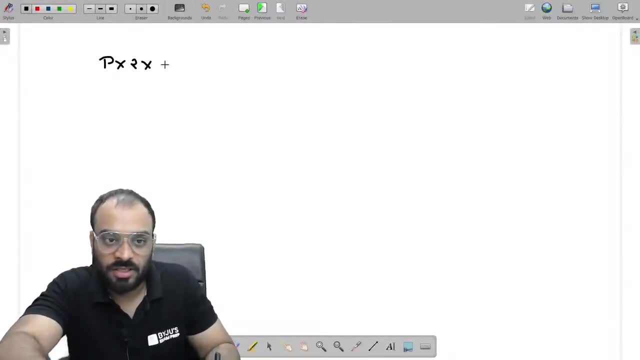 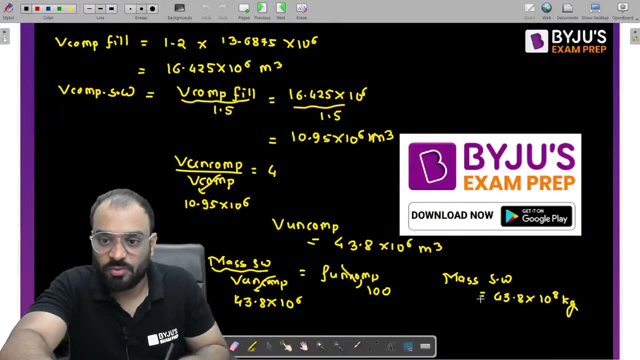 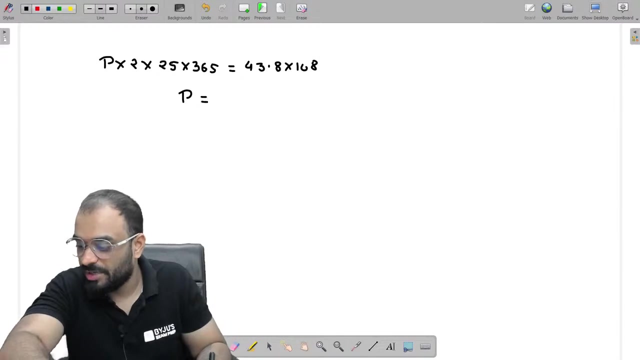 is 2 kg per day. the duration is 25 year multiplied by 365. now it can be equal to how much? it can be equal to 43.8 into 10, to the power 8. now calculate for how many person this particular mass can be generated. 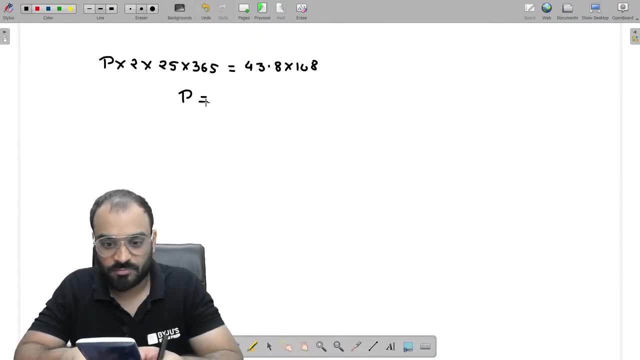 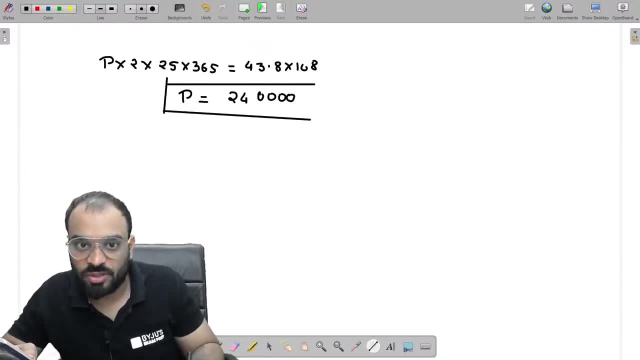 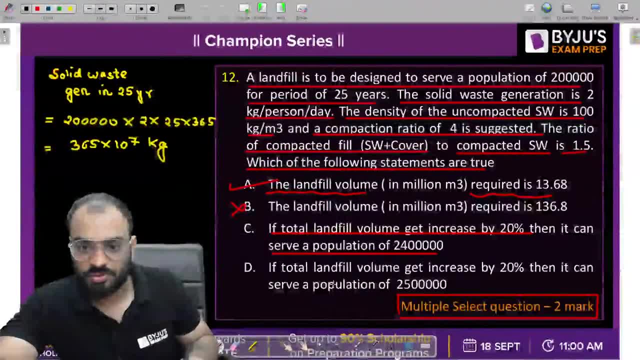 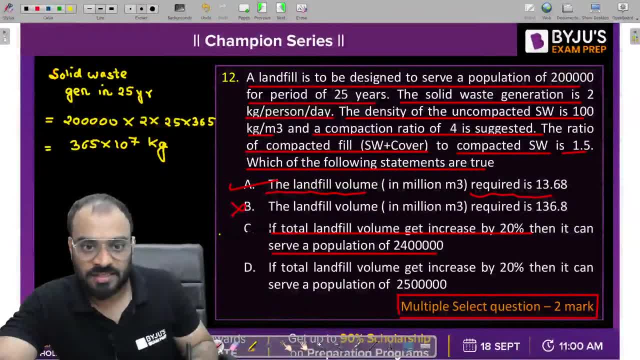 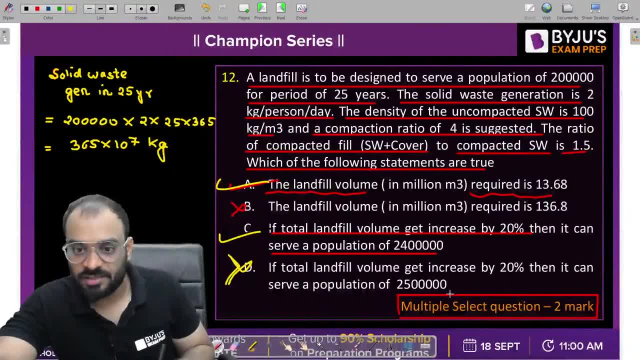 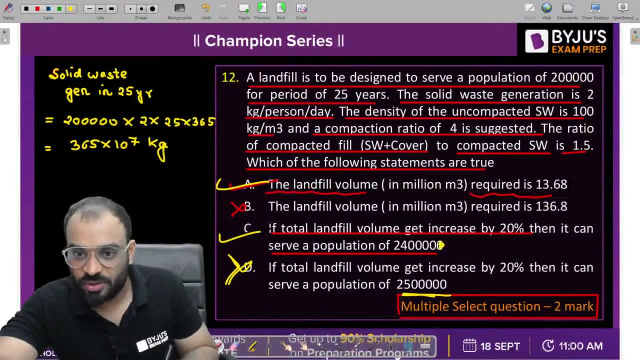 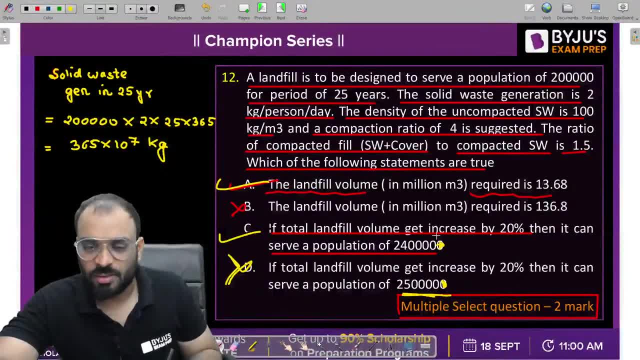 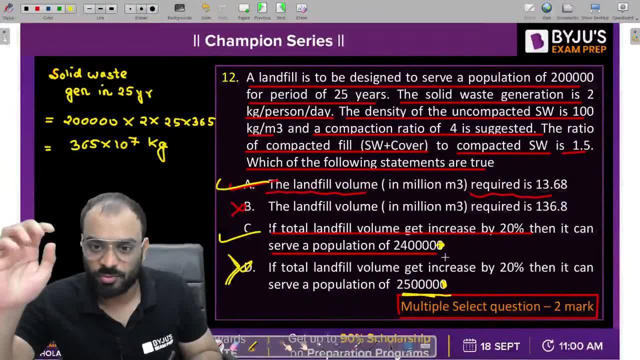 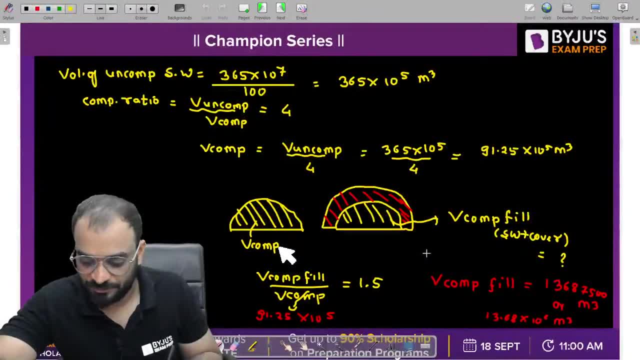 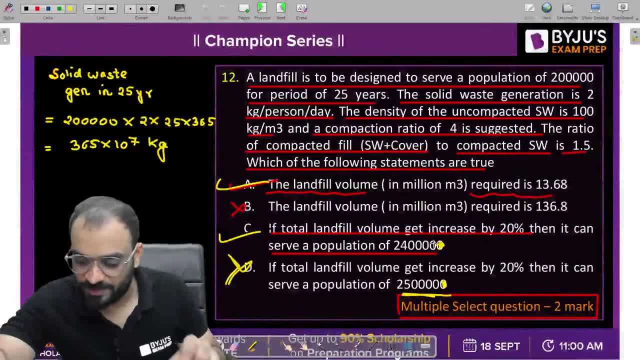 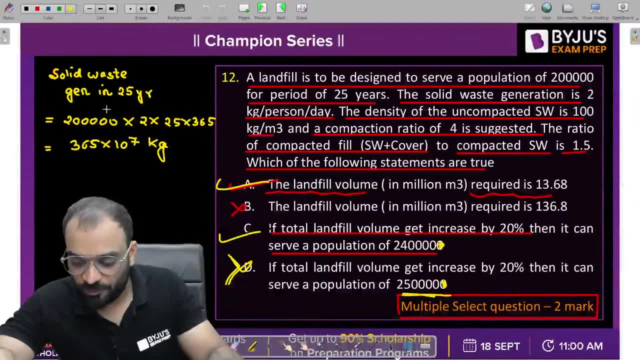 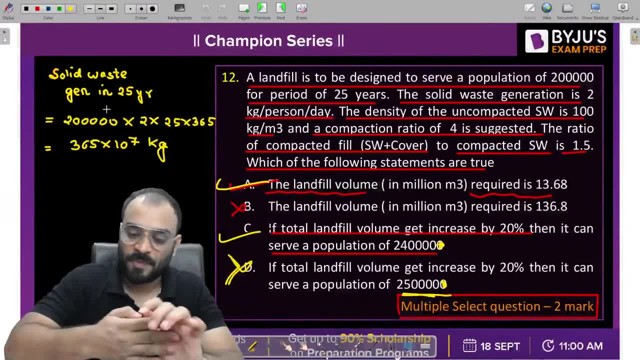 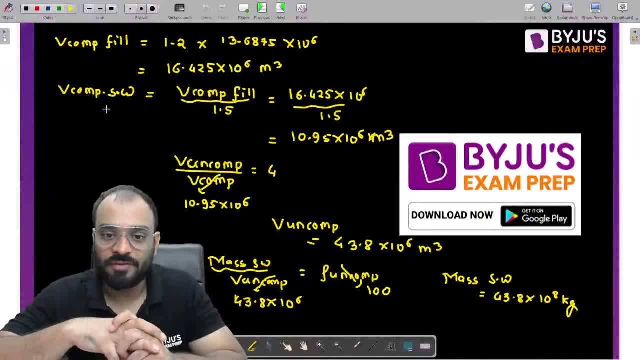 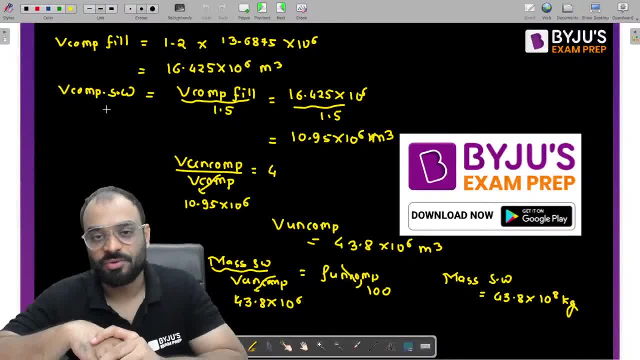 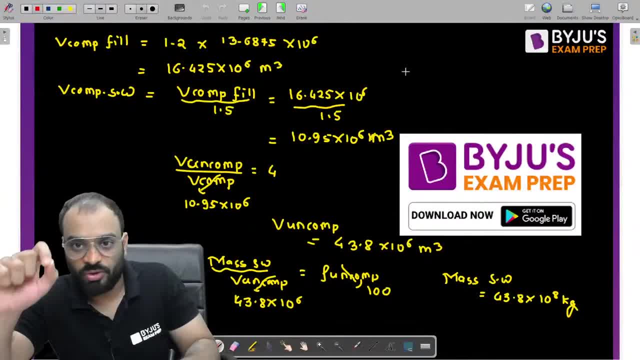 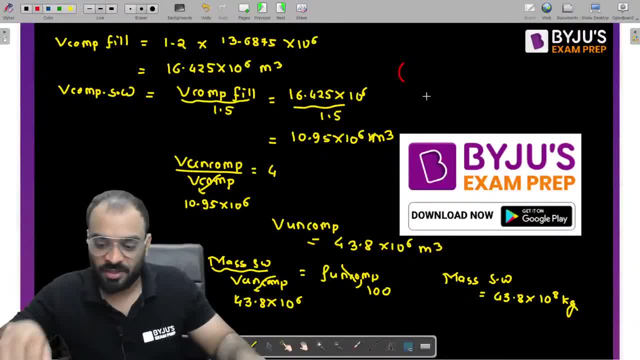 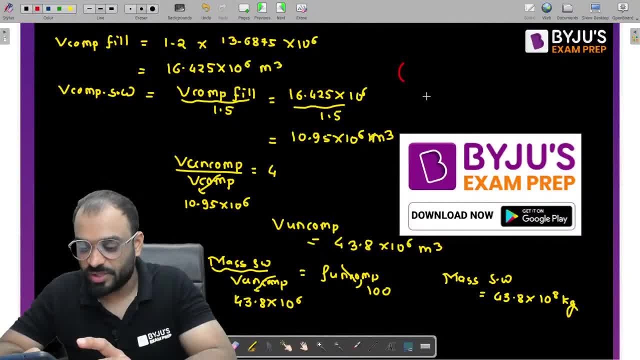 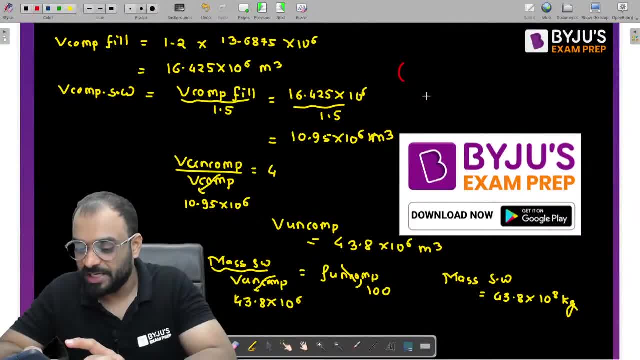 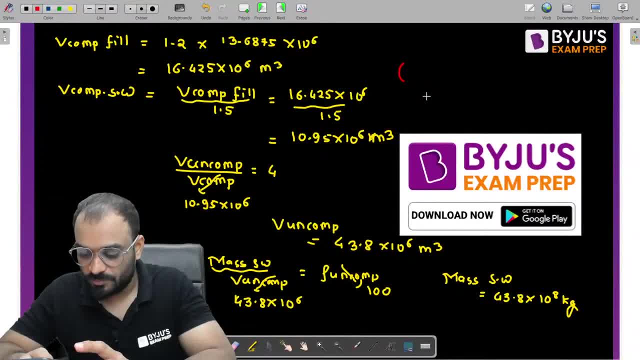 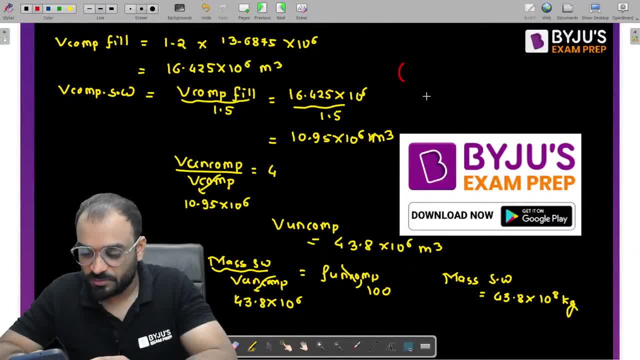 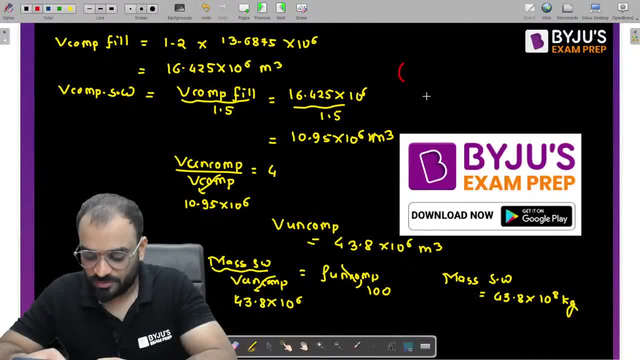 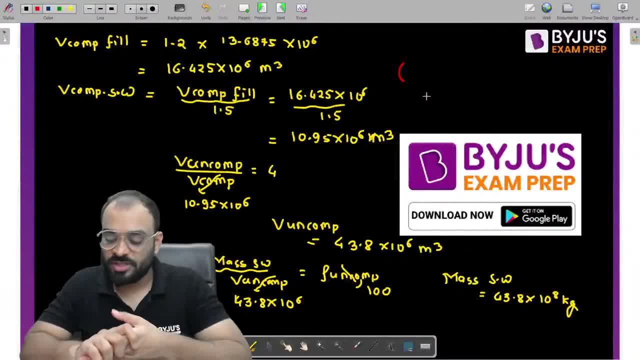 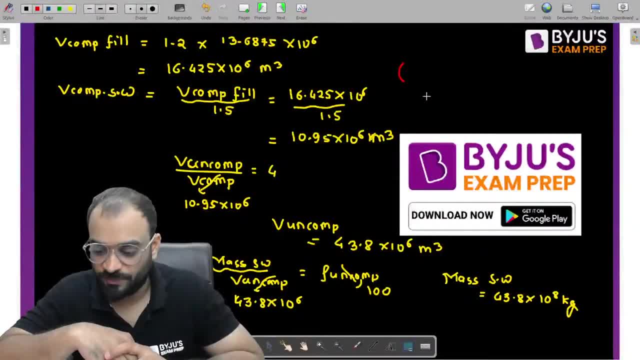 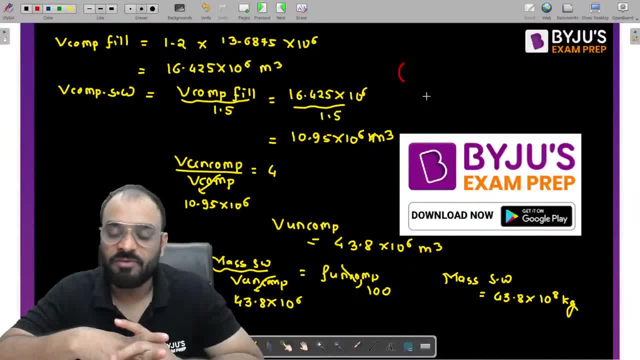 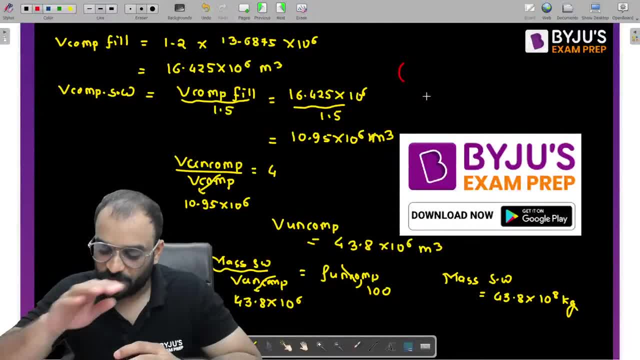 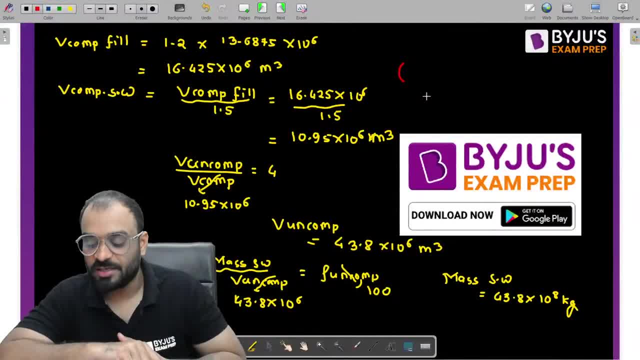 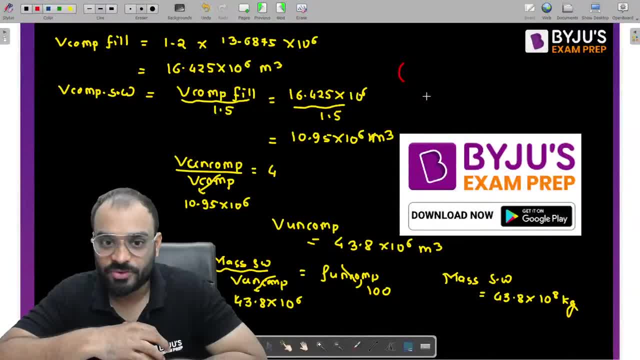 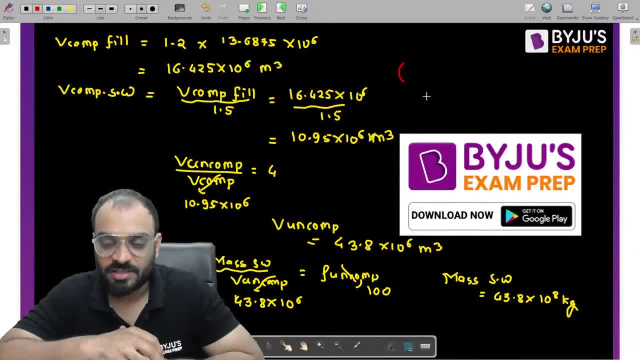 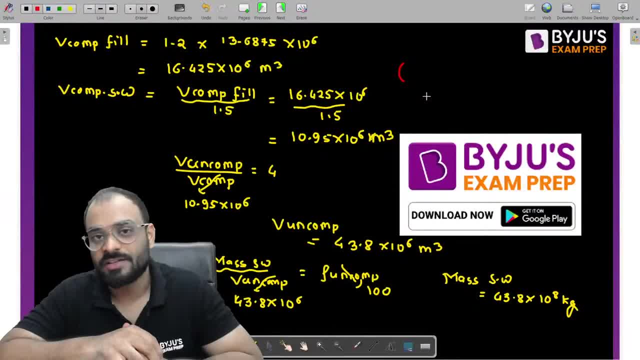 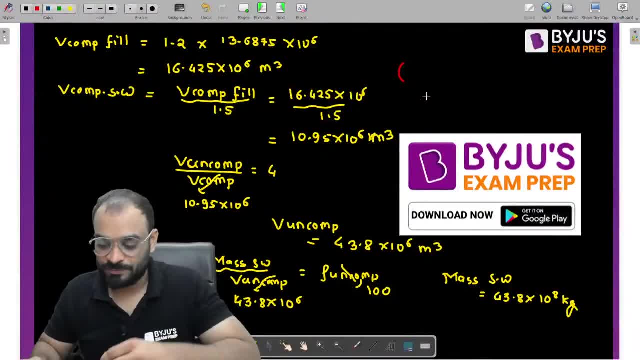 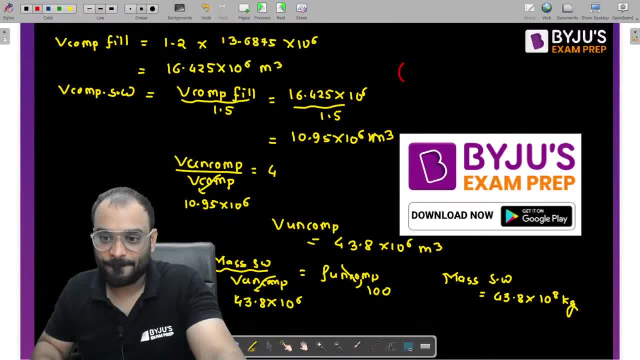